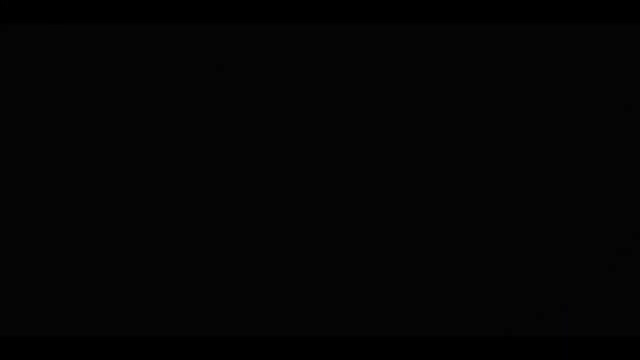 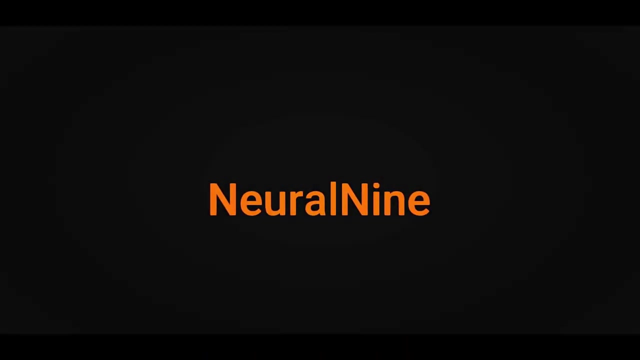 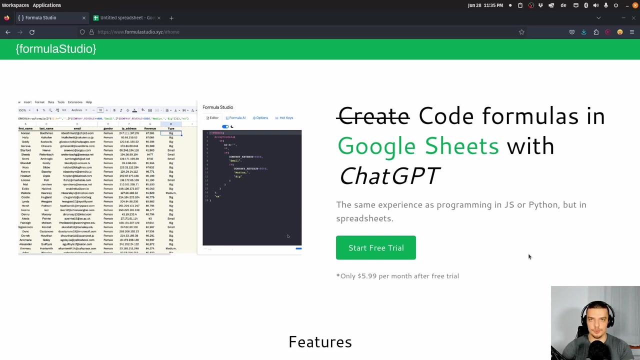 Matplotlib crash course. So let us get right into it Now. before we get into the actual tutorial, I would like to mention that this video is sponsored by Formula Studio, which is a GPT powered Google Sheets extension that can be very interesting to a lot of you guys, So don't skip this part. Now we can look at the functionality. 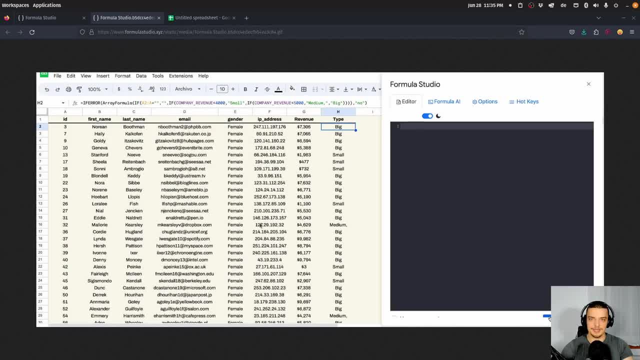 here in this example. I'm going to open it up in a new tab. here. This is an animated application, So we're going to open it up in a new tab. here. This is an animated application, So we're going to open it up in a new tab. here. This is an animated 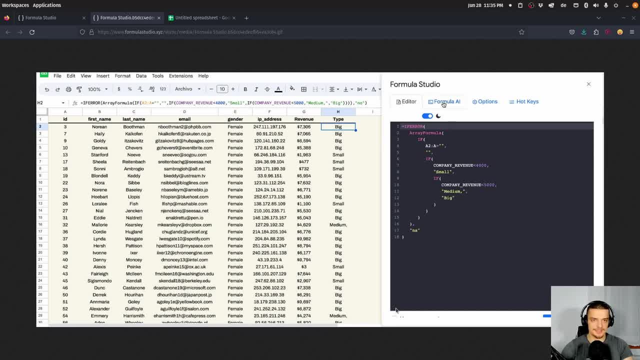 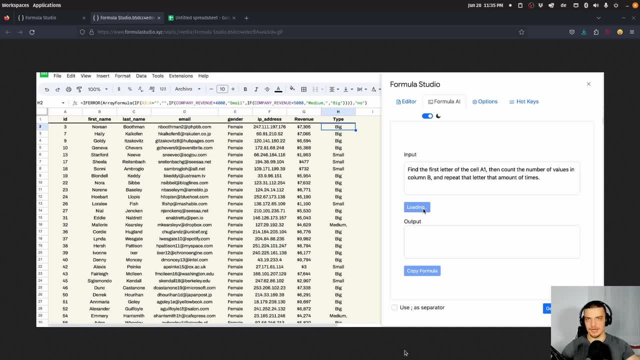 image And we can see here. one of the features is this editor on the right side which allows us to edit these Google Sheets formulas in a way that we would also edit Python code, with syntax highlighting and with multiple lines. And the second feature here is we can 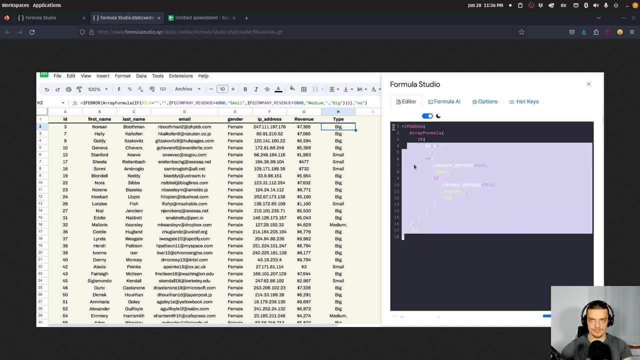 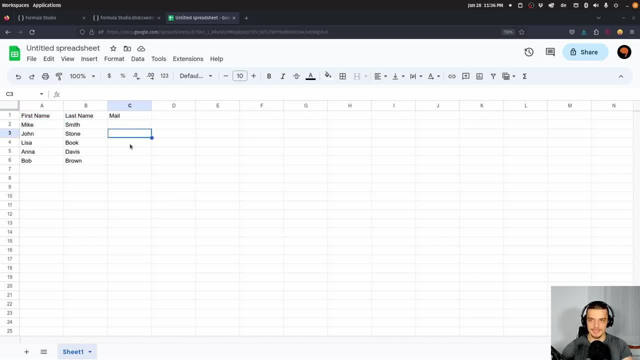 ask GPT to generate the Google Sheets formulas for us. I have prepared a simple example here. We have two columns- first name and last name, And then we also have an empty mail column, And now I want to just take the first name, the last name, I want to concatenate them in. 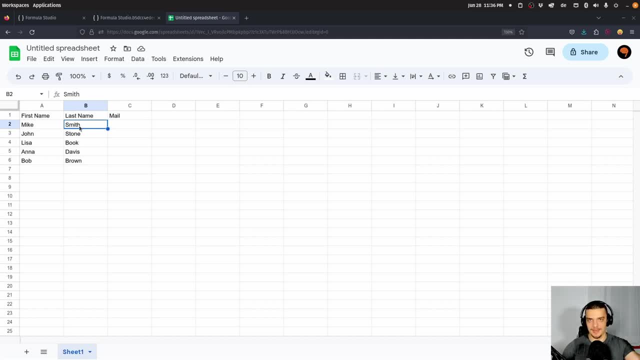 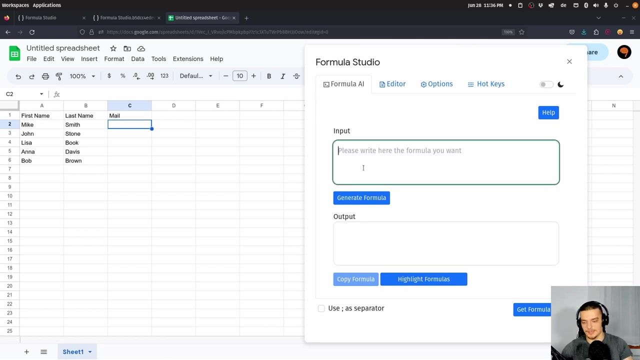 to an email which has the pattern first name, dot, last name at mailcom. A very simple example, but it's going to show you how this tool works. So I'm just going to open up the extension here, formula studio, open editor, And then we're going to go to the formula AI And I'm going to 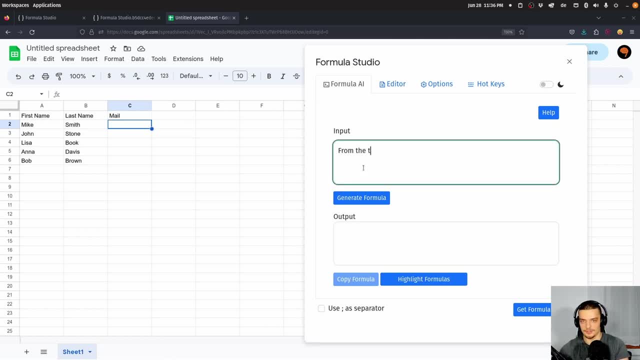 I'm going to say, from the two name columns, take the first and last name And combine them to an email all lowercase using this pattern, And then I can provide a pattern- first name dot, last name- at mailcom And I can just generate the formula here And this is going. 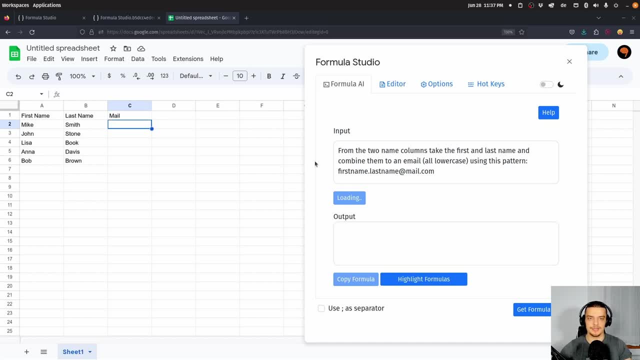 to give me something that I can just copy paste into the mail column, And if I'm not satisfied with the result, of course I can change the query, But in this case I'm going to just copy paste this here. There you go. And then I'm going to just copy paste this here, And then I'm going to. 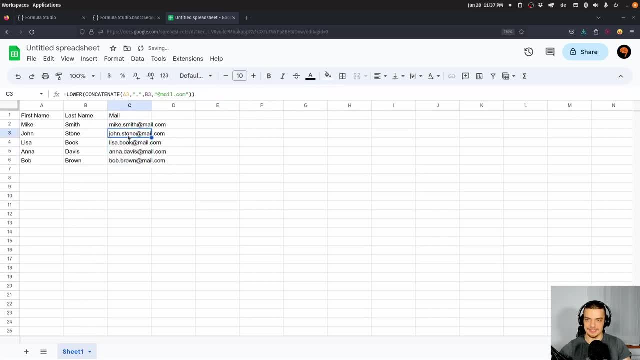 and now I can just drag this down And you can see that this produced a result that I was expecting. Now, as I mentioned, this is a very simple and trivial example, But you can do much more with this tool, So make sure you check it out at the link in the description down below. 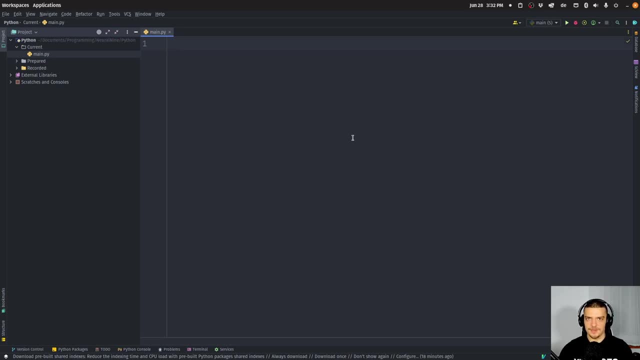 Alright, so we're going to do a full crash course on matplotlib in this video today And, as I already mentioned, matplotlib is the most used data visualization package in Python And it's super important for data science and machine learning processes because a lot of these steps 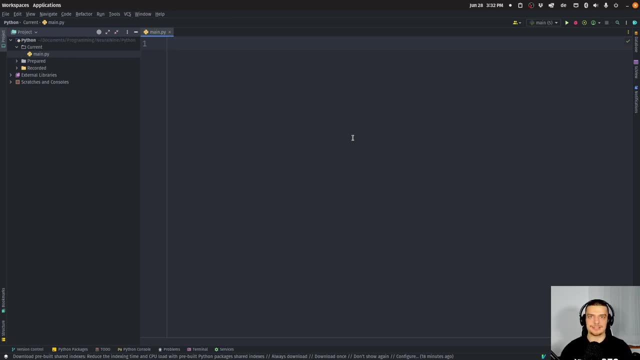 in those processes involve data visualization. So I'm going to go ahead and do that And I'm going at least can benefit from data visualization. So, for example, what you usually do is: you get data, you explore data, you pre process data, you train a model on the data and then you evaluate the 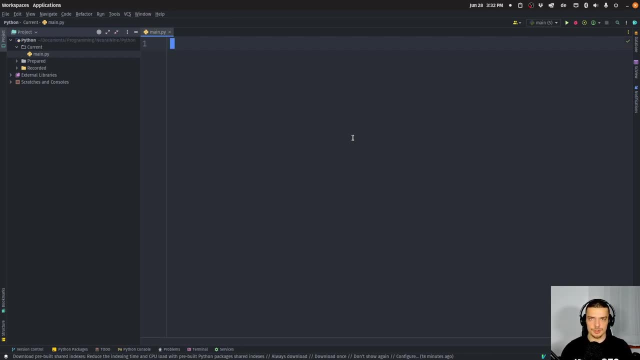 model using test data And, for example, in the exploration part. you usually don't want to just look at text or at numbers, at statistics that are not visualized, But you usually want to look at histograms, box plots or any other graphical representations of the data to get an intuitive 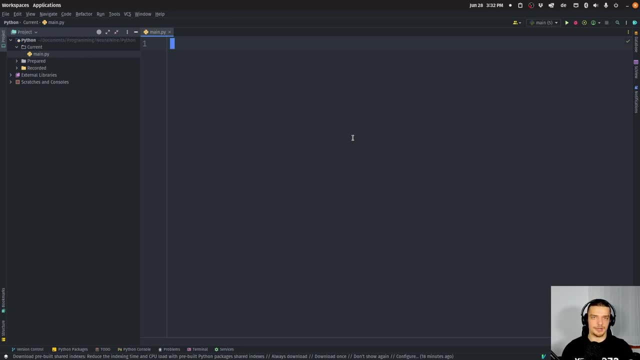 understanding of the data. So I'm going to go ahead and do that And, as I already mentioned, I'm going to go ahead and do that, And I'm going to go ahead and do that, And I'm going to go ahead of the data and to see certain patterns immediately that you would not see if you just look at a bunch. 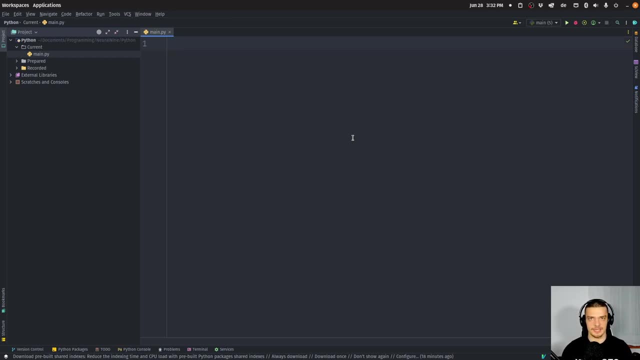 of numbers, And then you can also have some more advanced visualizations like correlation heat maps And, of course, when you evaluate a model, you can have certain graphical representations of the results that are more intuitive, especially when you have to present it to a business person. 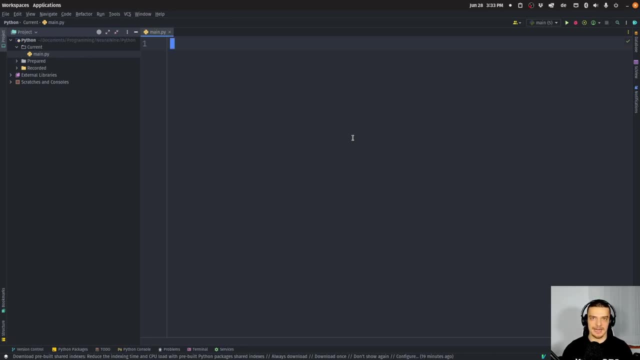 not to a technical person- that might make a lot of sense. And then you also have certain situations like in k-means, clustering, to choose the optimal number of data. And then you can also have certain plots that you can, you can draw so that you can find the quote unquote optimal. 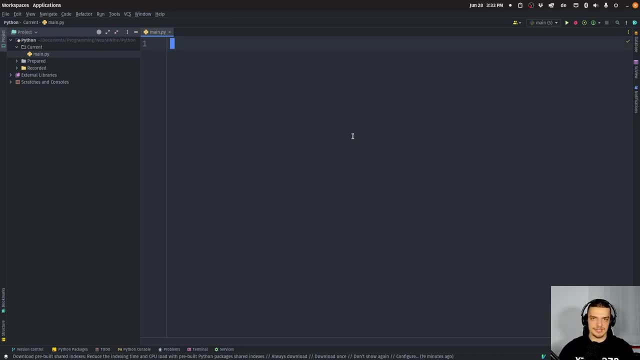 number of clusters. So there are a lot of use cases in data science and machine learning where visualization can help you not only understand the results, but also to to find better parameters for the training itself and to actually understand the data before you build the model in an intuitive 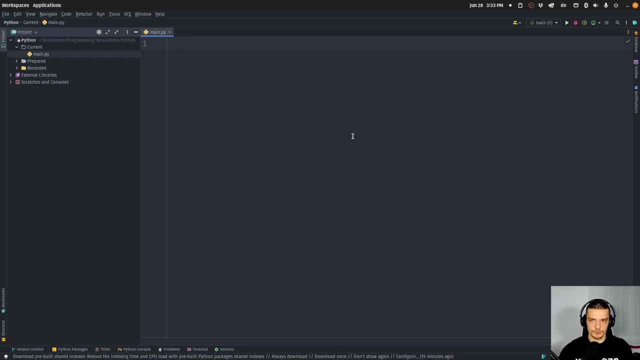 way, And matplotlib is a very powerful tool that allows us to do that. And today we're going to cover the different aspects of matplotlib. we're going to start with some basic plot types, then we're going to go into styling, into plotting multiple plots, into into animations, into 3d. 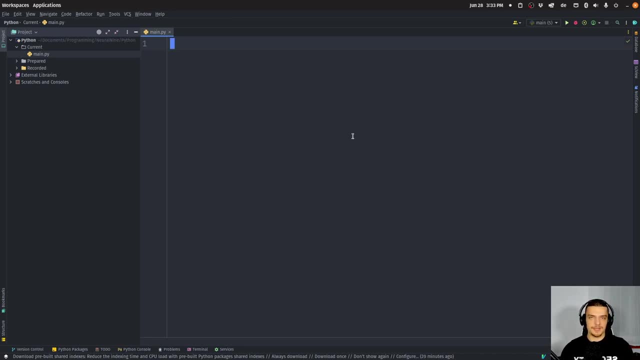 plotting and stuff like that. So it's going to be very beginner friendly. we're going to start from scratch And then we're going to go into some more advanced topics as we go on here- everything in one video today. So, of course, the first thing that you need to have is you need to have matplotlib. 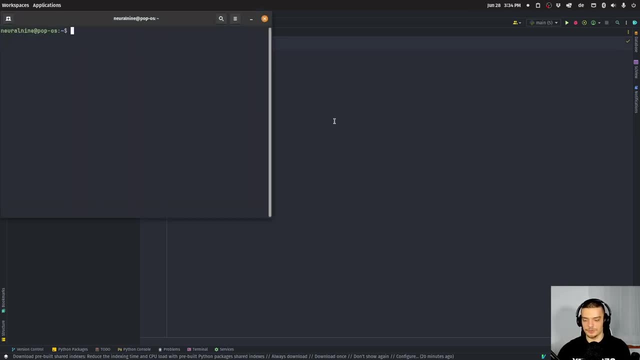 installed on your system. And for that we're going to open up the command line and we're going to use matplotlib, And then we're going to go into some basic plot types. And then we're going to go into some basic plot types And then we're going to use pip- in my case pip three- and we're going 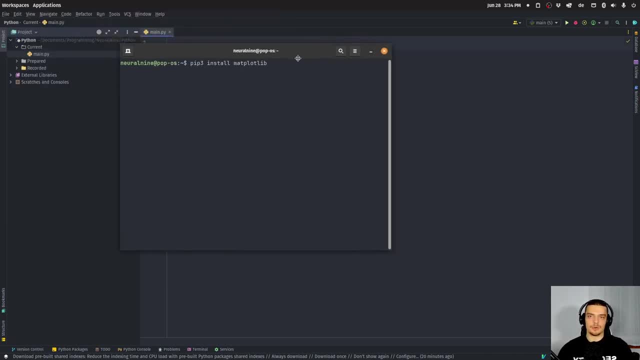 to install matplotlib. Now in this video today we're also going to use numpy. Now numpy is not necessarily a prerequisite for matplotlib. you can use matplotlib with ordinary Python lists. But in data science usually you have data sets that you process with pandas. 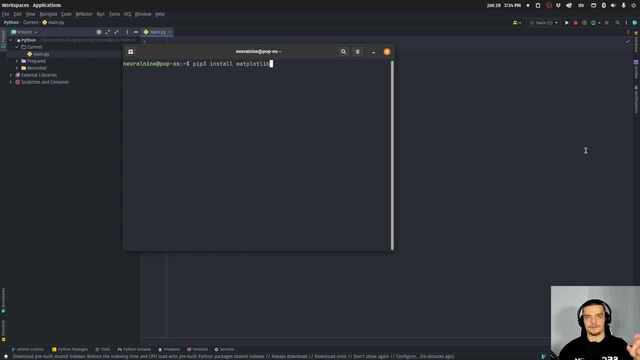 you have the visualizations that you do with matplotlib And you have numpy that you use for basically everything: for working efficiently with arrays, for taking data and feeding it into machine learning algorithms, for transposing it, for pre processing in general, for doing all sorts of things you use numpy. So I also have a numpy crash course on my 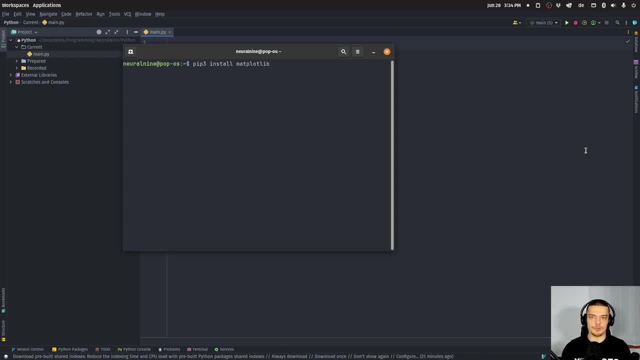 channel if you want to check that out. But for this video today we don't need some advanced numpy. we're just going to generate some data that we can then visualize using numpy, But because of that we're going to also install numpy here. So, pip, install matplotlib and numpy And once you, 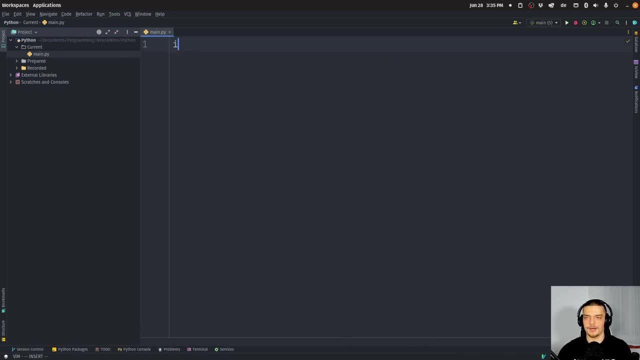 have that you can just go into a Python list And then we're going to go ahead and install numpy into a Python file And you can import numpy as np And we can import matplotlib, dot, piplot as plt. This is the usual convention, because most of the stuff that we need is going to be provided. 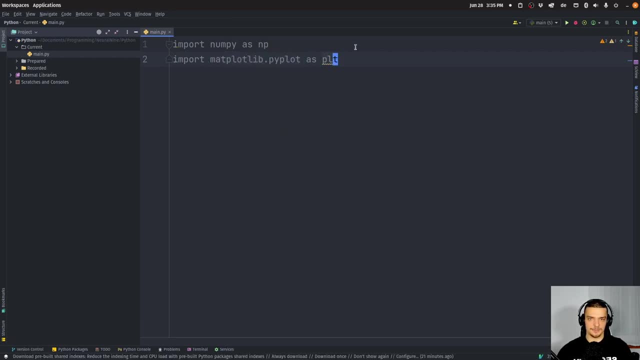 by the piplot module of matplotlib And because of that we import it specifically and we imported as plt. This is just an alias here which is used everywhere essentially. So what we're going to do is we're going to use numpy to generate some random data. So we're going to say here: x. 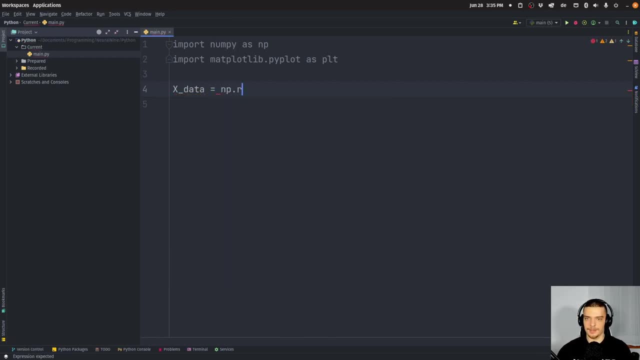 underscore data equals and then numpy random. let me just lower my microphone a little bit so that I can see my keyboard to minimize the mistyping here. So np, random, dot random, we're going to have 50 values And we're going to multiply with 100. Then we're going to get y data here as well. 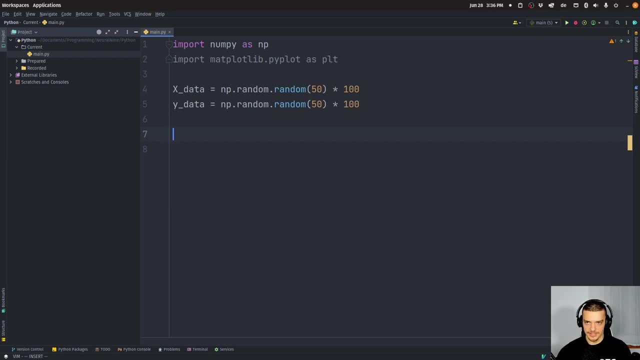 Same principle, And then we're going to use the first plot type that we're going to learn about in this video today, which is the scatter plot. The scatter plot is just a bunch of different data points plotted as dots, as points. So, in order to create a scatter plot, we just have to say: 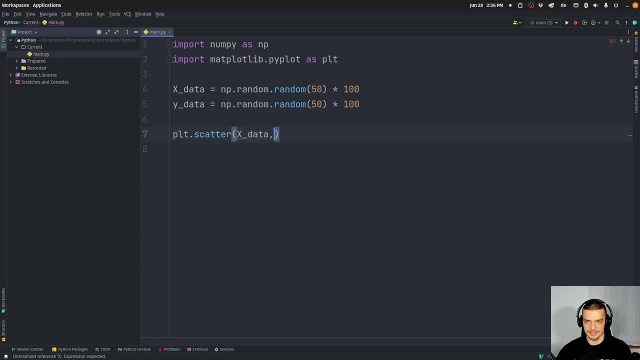 plt dot scatter and we pass the x data and the y data And then every time you make a plot in matplotlib you need to also show the result specifically, unless of course you're working in Jupyter Notebook environment, then the plot is displayed automatically usually, But if you are, 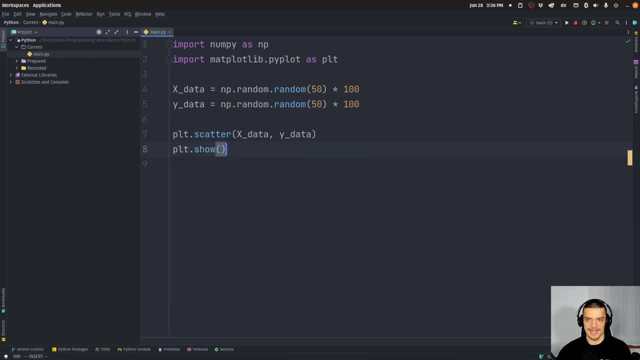 working in an application like this, you have to say plt show, to actually show the graph, to actually see the result, And when you run this you can see. this is the first plot of this video today. So essentially we just have the individual data points, in this case, randomly generated points. 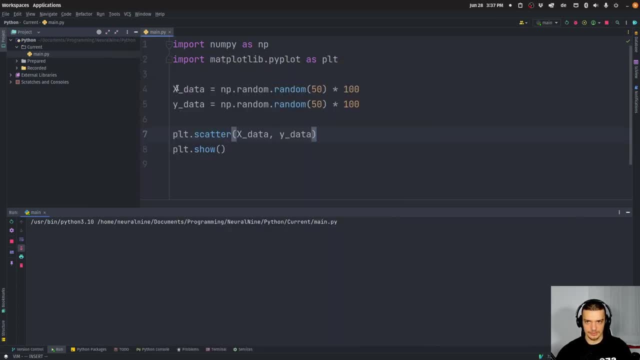 between zero and 100.. So that's the logic of these two lines. we have random numbers And when you use the random function of NumPy you get values between zero and one. we get 50 values between zero and one and we multiply all of them by 100 to get data points between zero and 100. 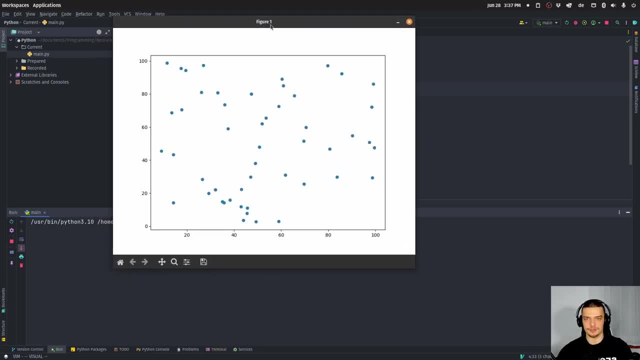 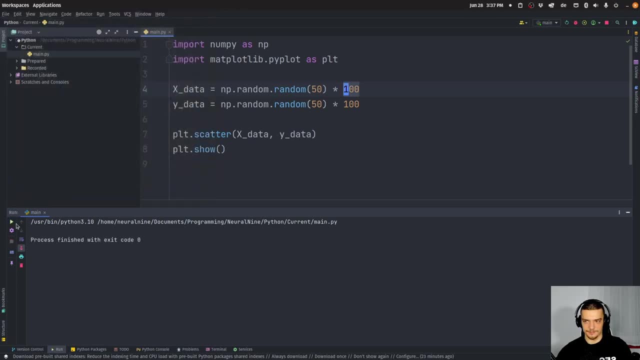 And this is the result. So a scatter plot is just taking individual data points and plotting them as points And, of course, when I run this again, we will get different data every time because the points are randomly generated. Now, for those of you who have no intuition of 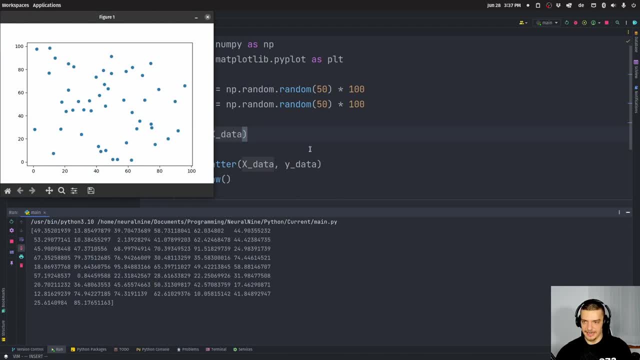 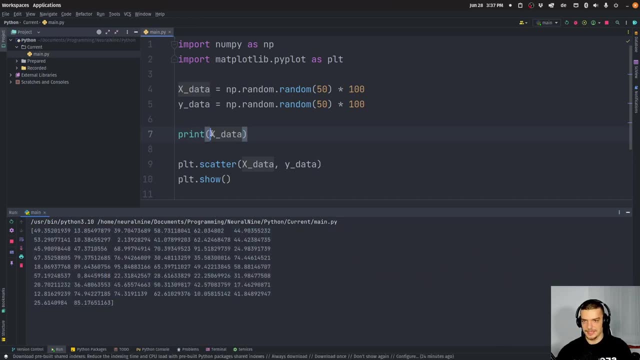 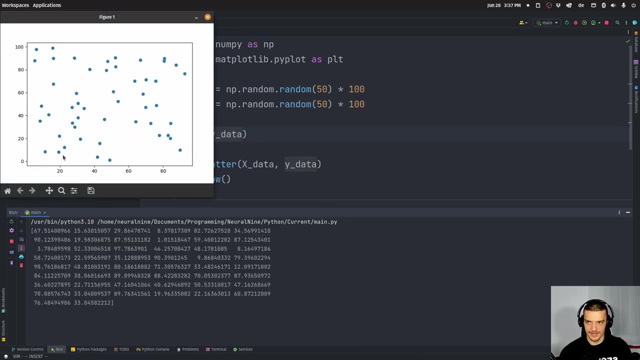 NumPy we can print the x data And you can see those are just the x values. Those are just 50 values between zero and 100. Nothing special about it. And the y data- same thing. So we just have 100 values for the x axis, 100 values for the y axis And then the combination. 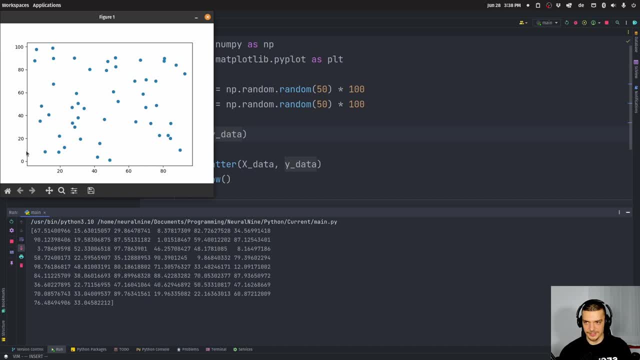 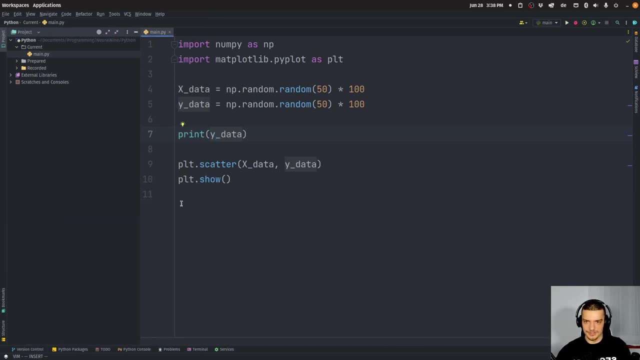 of these two values is a point. So we have this x value, this y value and this is the data point, and thus we plot it. We're going to get into styling later on. I'm not going to discuss the different parameters that we have here, like color, line, width, line type or in. 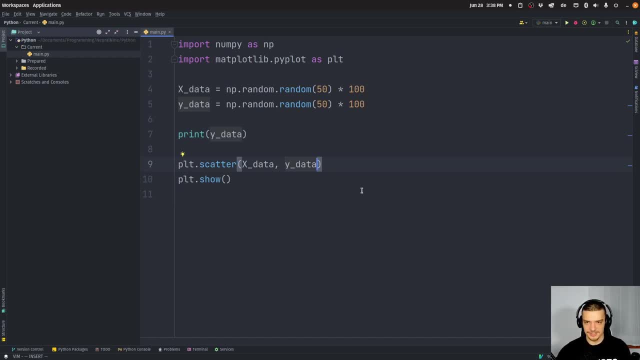 this case we don't have lines, But you can have markers, you can have sizes, you can have colors, But for now we're just going to cover, or actually we're going to do it like that. I'm going to show. 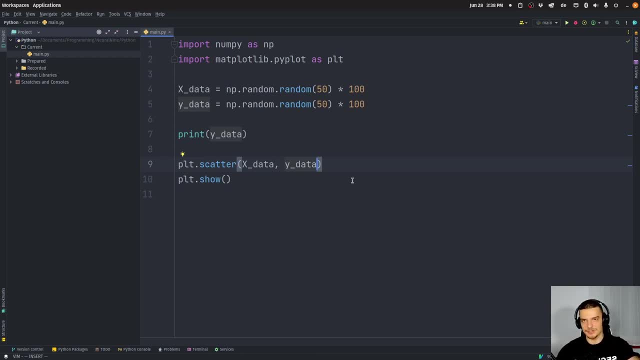 you the basic styling options for the individual functions. But later on we're going to get into styling in general, into more detail. But of course, if you want to have the complete picture for every function that I show here today, for every concept, for every plot type, there's a lot. 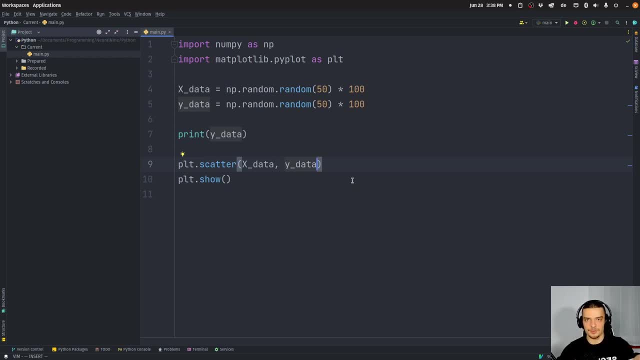 more than I can show in one video. So if you want to have the complete parameters to complete descriptions, all the different values that you can have, it's always a good practice to go into the documentation and look up the individual functions, the individual parameters to individual. 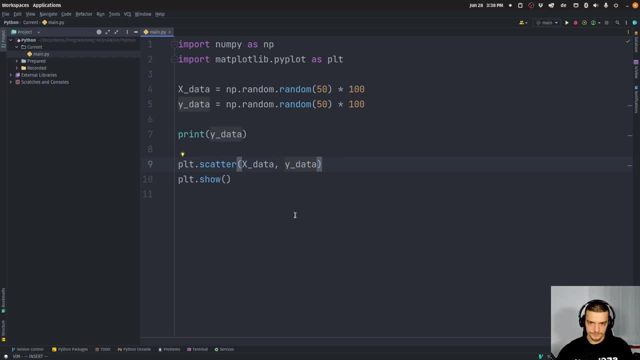 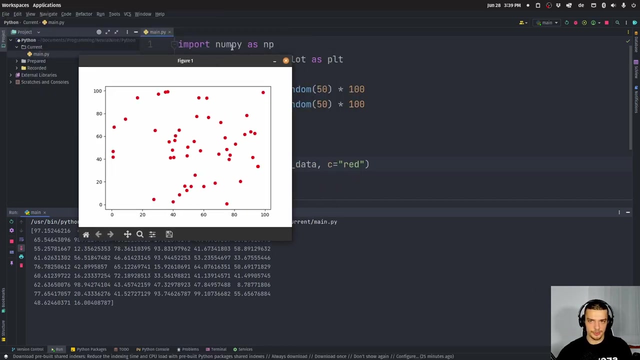 examples, because of course you have a lot of options here, But we're going to say here now, for example, if I want to have a different color, what I can do is I can say C equals, and I can say red, for example, as as a word, And now you can see I have red points instead of blue points. 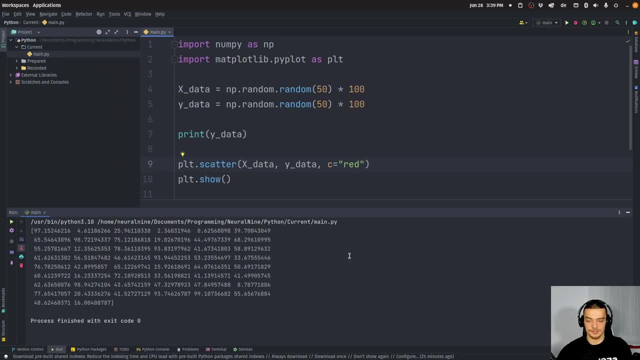 here in the scatterplot. But of course you don't have to provide color names. you can also provide hex color. So I can say hashtag to specify a hex color code And I can say, for example, 000,, which would be black, Or technically it's 000000.. But you can abbreviate it. 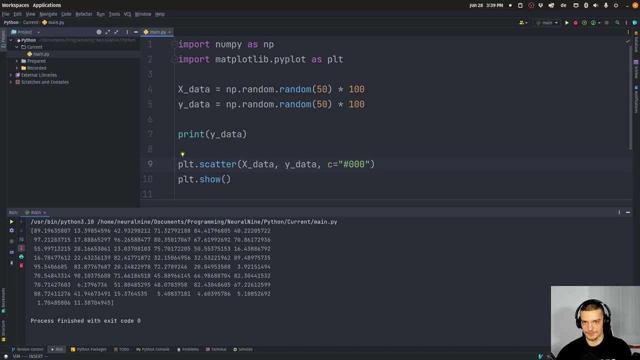 or you can write it in a short form by just using three zeros, And then you can also do: for example: green RGB means 02550 would be zero F, zero for green, So you can specify colors like that as well. And then what we can also do is we can provide. 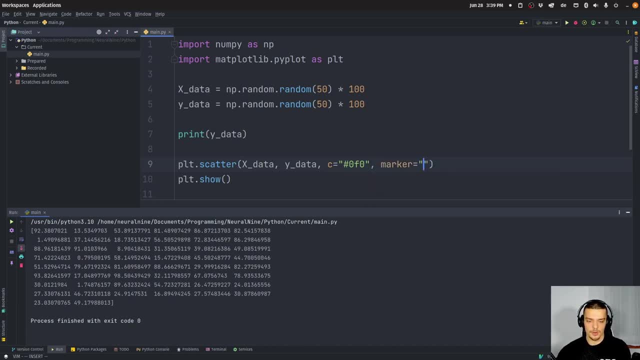 a different marker, we can say, okay, I don't want to have points, I want to have stars. So I can provide this asterisk symbol here And you can see now that the data points are stars, And maybe you can see that better if I go for a blue color. There you go. 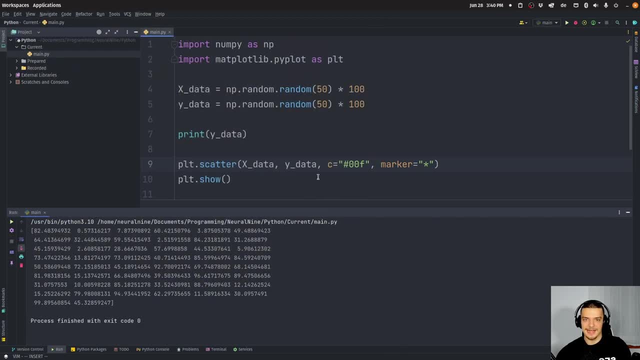 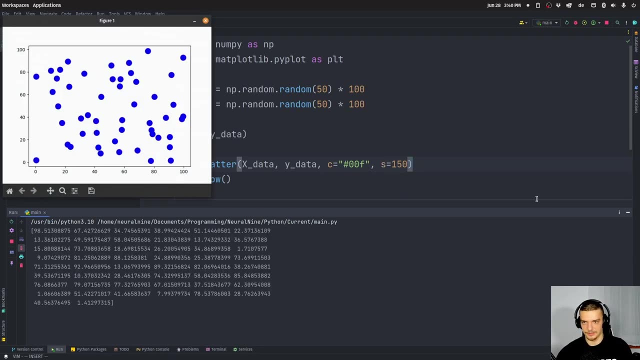 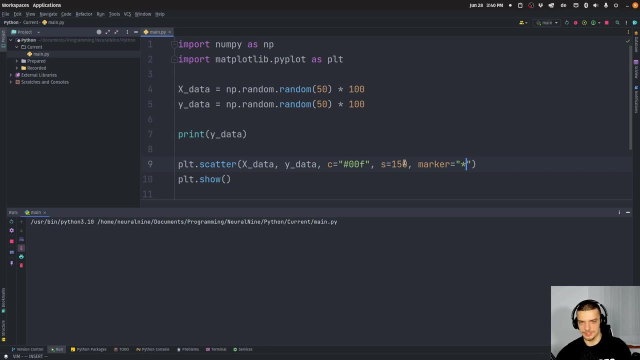 So those are the individual data points, now with a different marker, And if you think that those are too small, you can just go ahead and say: s equals 150.. I think this should be larger. There you go, But I deleted the marker, So now we have points again. Let's go for stars again. 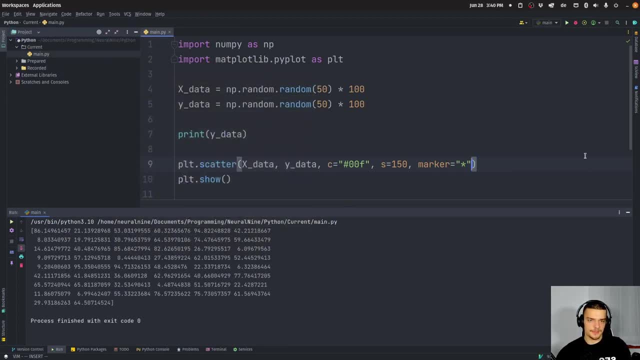 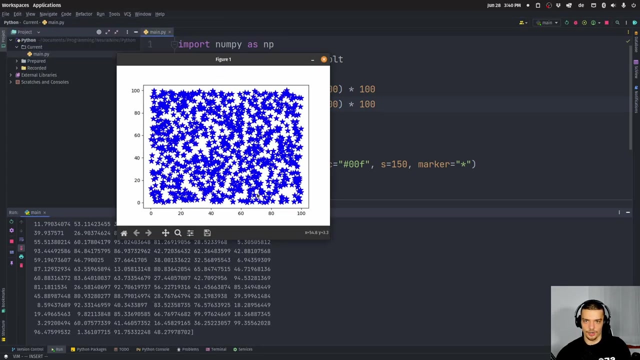 There you go, And of course I can also make them transparent. So you can see that this might make sense. if I have 1000. Or actually, this is the wrong number to change- If I have 1000 data points instead of 50, you can see that a lot of them are overlapping. 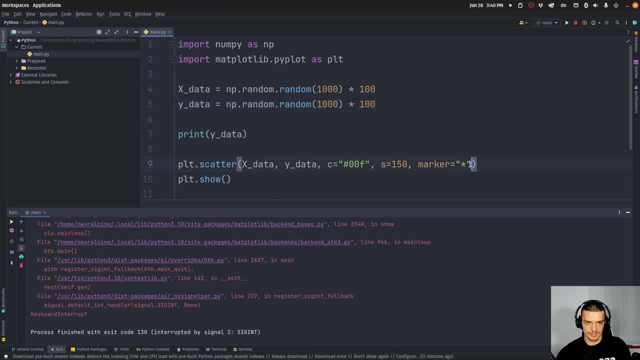 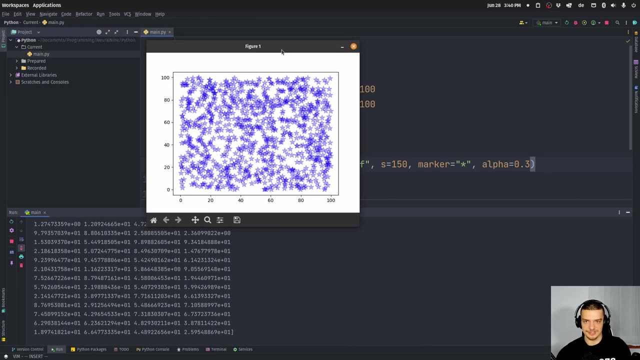 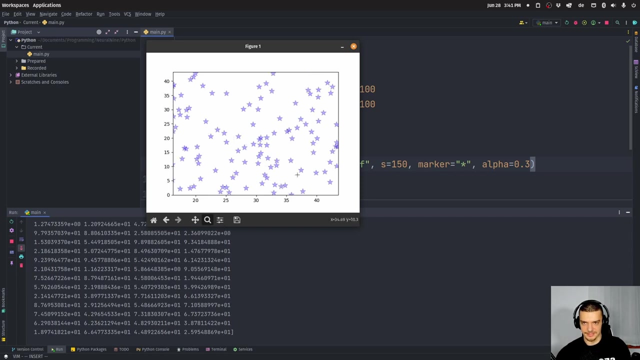 And to see where I have more elements, I can just go ahead and say alpha equals 0.3., Meaning there is some transparency here And you can see if those stars overlap. we have darker zones here. I mean, actually now when I zoom in they don't overlap. 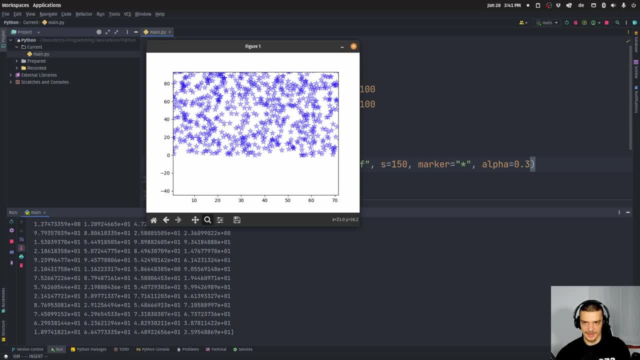 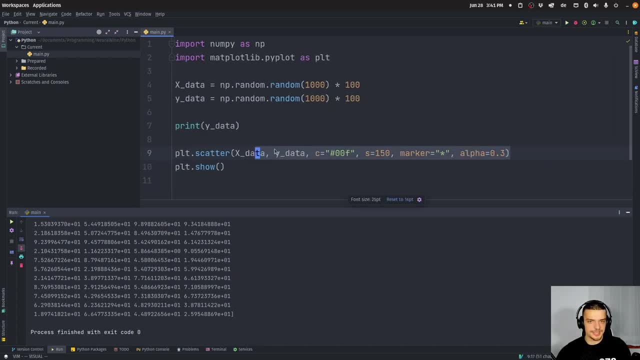 But if we have some overlap you can see that we have darker areas and we have some more lighter areas if there is no overlap. So yeah, those are some basic, interesting parameters for scatter plots. you can adjust the color, the size, the marker and the transparency. 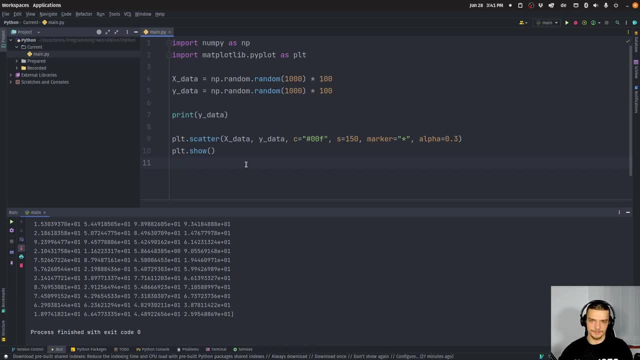 Now, sometimes you don't want to plot data points because you don't just have two attributes and you want to scatter the points. you want to have actually some connections. you want to plot a line because you have, for example, time series data, you have certain years and you have 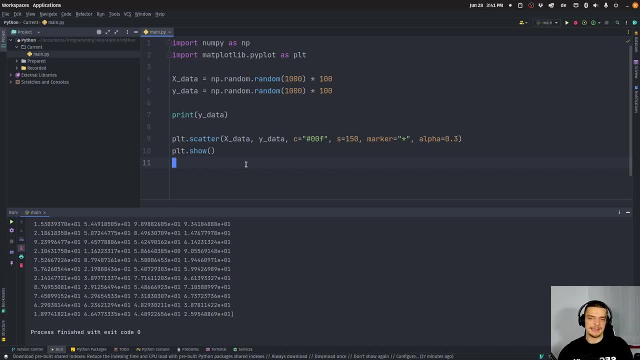 another attribute that you want to keep track of over time. in this case it makes sense to not use a scatterplot but to use a line chart, And for this an example would be to say: I'm going to use an ordinary Python list here. Now let's say I have years. any years are. 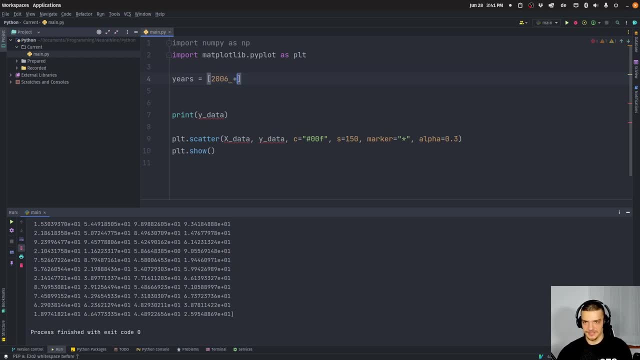 let's say 2006.. And I'm going to use a formula for this because I don't want to use, Don't want to write out all these values here myself. I can say plus x for x in range 16.. I'm going to have now 16 years, So I'm going to print this so that you can see what this actually. 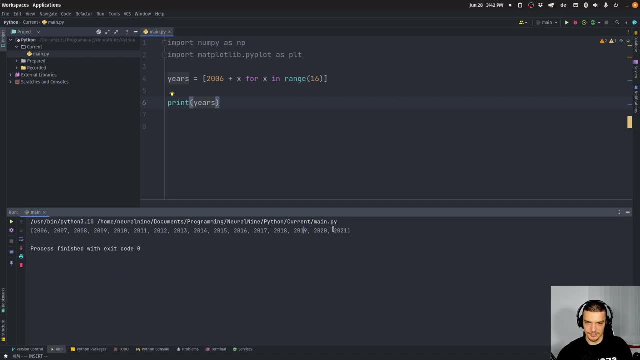 does is I got 2006, 789, 10 and so on up until 2021.. So I just generated some years here And I'm going to do the same thing with weights, or actually the weights I'm going to put in myself And the 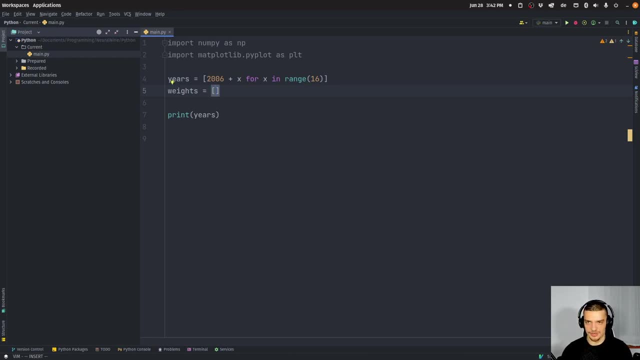 idea is that I want to visualize the weight change of a person over all these years here. And how can I do that? I just have the years And I have some weight, So I'm going to use kilograms: 80, 83, 84, 85, 86. Then maybe 82, 81, 79, 83. And how do we? how many values do we need? We need: 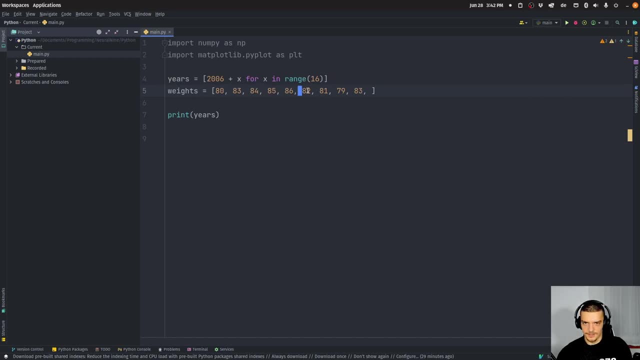 16.. So 123456789.. Let's go with 8010.. So now we have 82, 82, 83, 81, 80, 79, I think this should be 16.. We can actually confirm that by saying length of years and length of weights. But that is some typical data of. 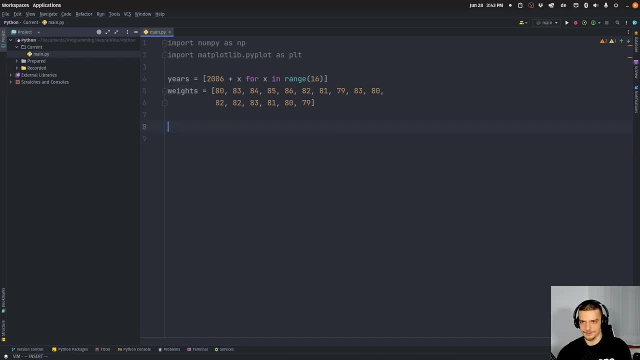 course that you would want to plot as a line chart. And here what we can do is we can just say PLT dot plot. we don't need to say PLT line, because the default plot function plots a line chart. So PLT plot, years and weights or weights, and then PLT. 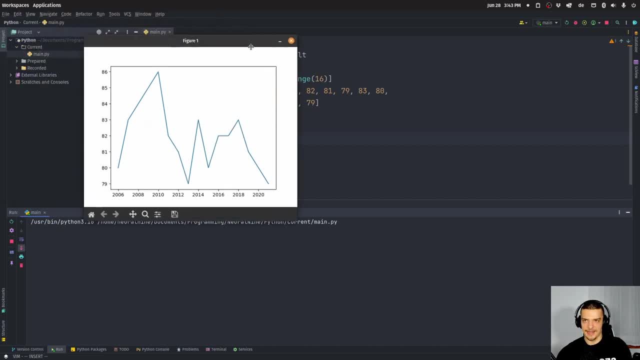 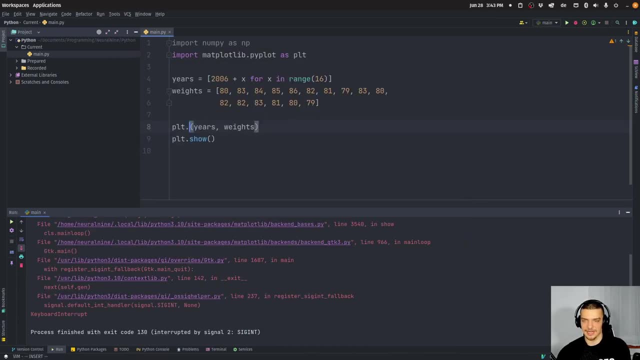 show again to actually display the chart, And then you can see: now we have a line chart, So the points are interconnected and not just individual points. Now, of course, I can also plot this as a scatter plot. this would still work, of course, But then you get a different picture. So I have the individual. 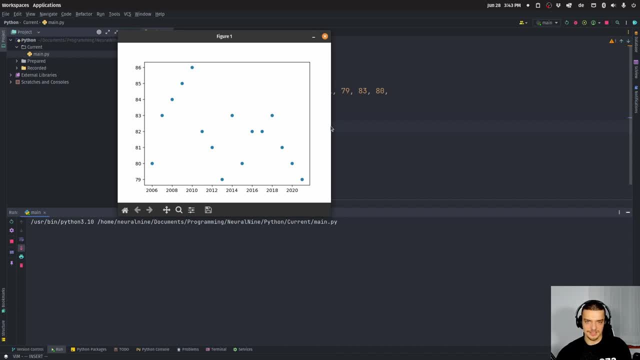 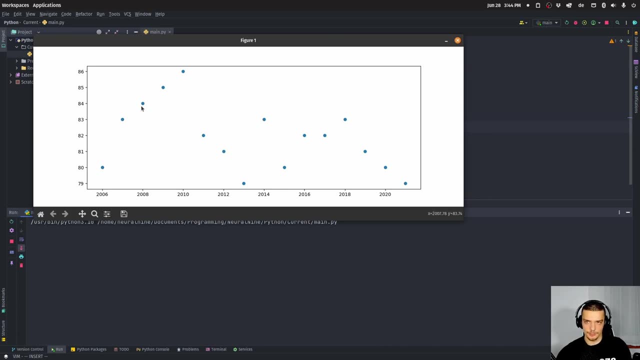 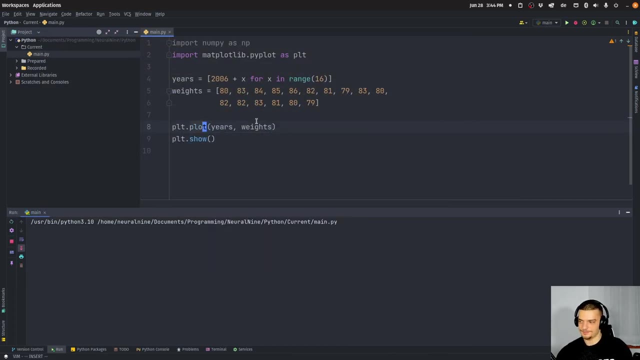 data points instead of a connection, which doesn't make a lot of sense here, because we have progress over, or change over, multiple years And of course, these points are connected- they're not just individual data points here. So it makes sense to use a line chart, As you can see here, And of 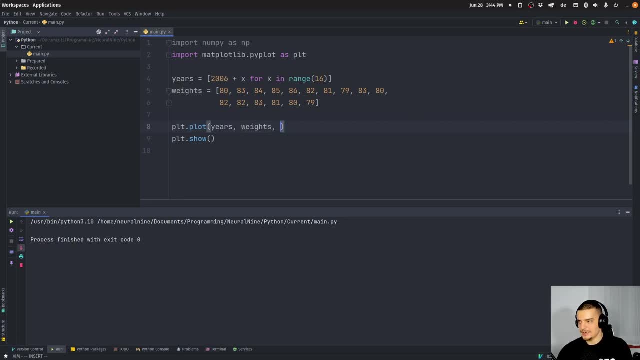 course, here we have again different customization options. So I can say that I want to have a certain color. again same thing. I can say color equals red, and I have a red line chart. I can also, by the way, just say color equals R. 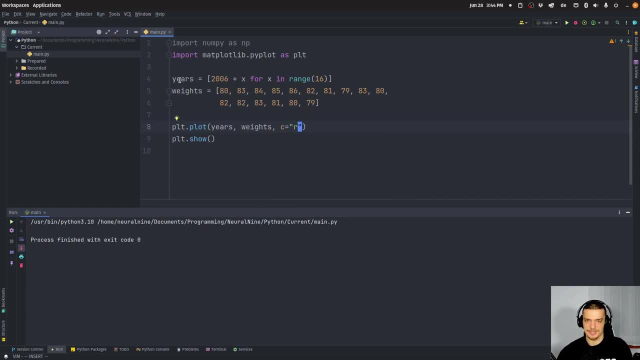 So if I go with red, it's going to be red. So in this case, R is red. I think if I go with blue, it's going to be blue. If I go with, or if I go with B, it's going to be blue. If I go with G, it's going to be green. 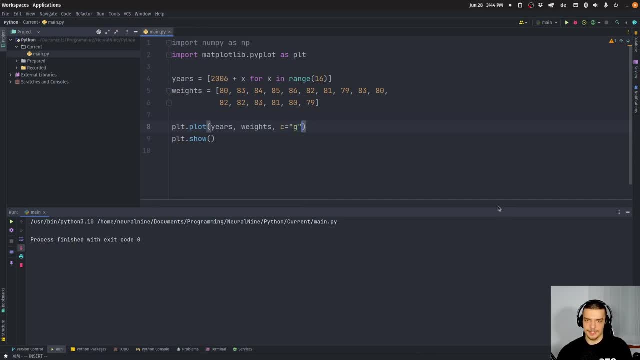 Yeah, So you can do it like that as well. And then we can do stuff like line width. So I can say, okay, I want to have a thicker line, So LW is going to be equal to three. And now you can see the line is. 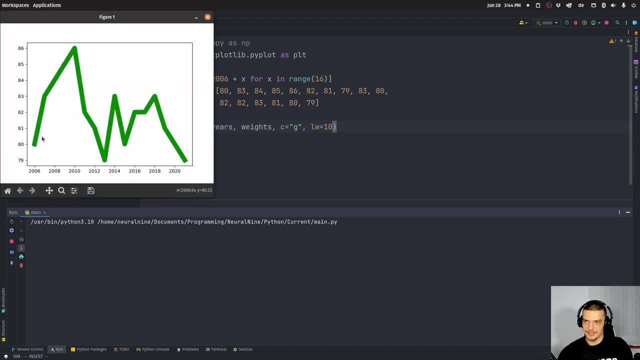 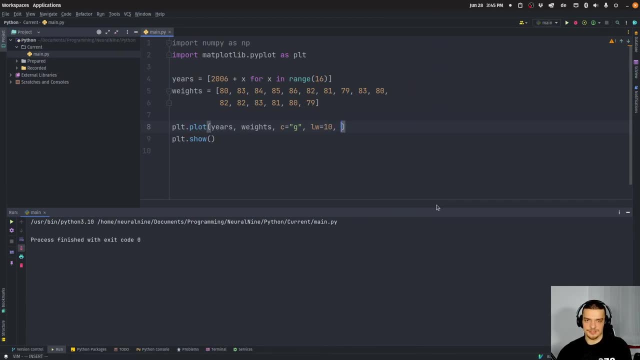 thicker. I can even make this more extreme by setting this to 10.. And you can see that we have a very thick line here. and also i can change the line type so i can say, for example, i want to have a dashed line, i want to say, uh, line style is going to be equal to dash, dash, like this: hyphen, hyphen. 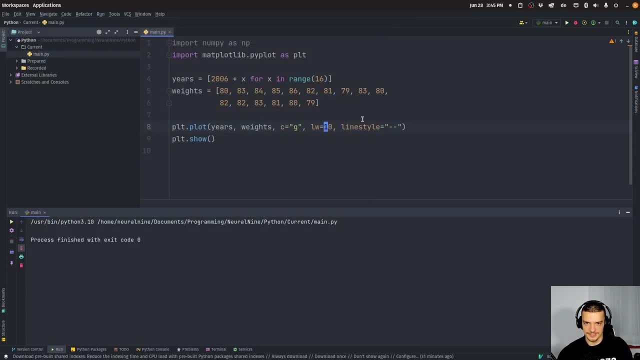 it is going to produce a dashed line and of course, in this case doesn't look too good because we have such a thick line. but yeah, this is how you can also change, uh, the styling here. uh, by the way, this can also be done, uh, by just specifying a positional parameter. so i can say years and 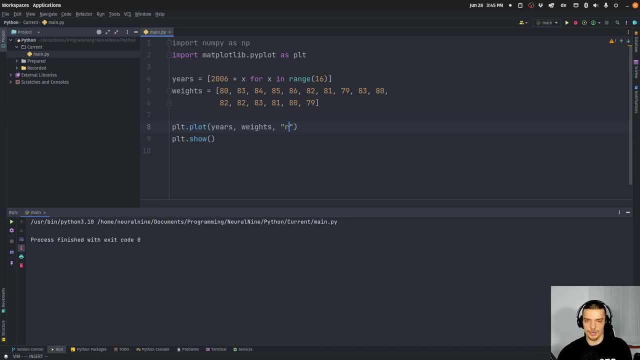 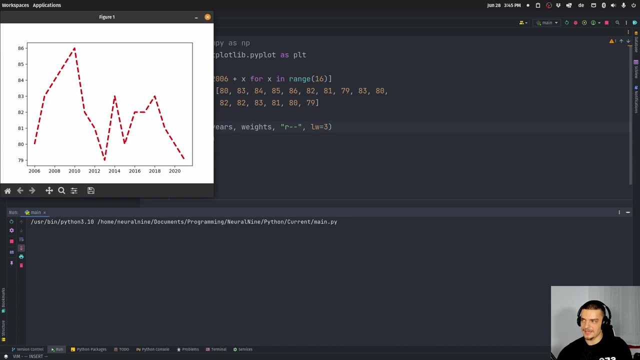 weights, and then i can pass a string here, and i can say r, dash, dash, to have a red dashed line. so this also works. i think, though, the line width needs to be passed separately, so i would have to say l, w and three. there you go, so this also works here now. so now we have basically just scattering. 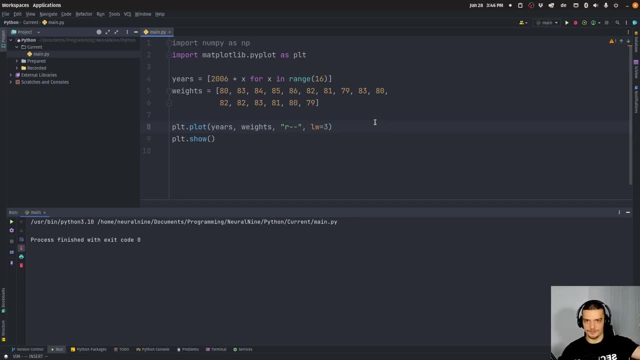 just plotting out different points, connecting them on on a time series, for example, and now we want to look at categorical data. so sometimes you might have a poll, you might ask the people what is your favorite programming language, and then you want to visualize the results of that poll, of that survey. 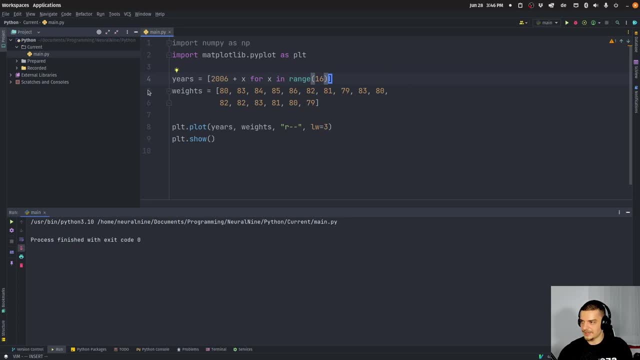 so, for example, you could have: uh, let's go ahead and say x equals, and i'm going to say c plus plus c, sharp. so we have a lot of different types of data. so, for example, we have the data of python, java and go and then we have the y data would be the votes. 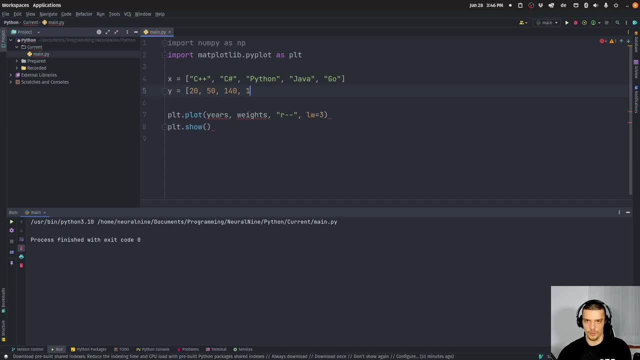 so i could say we have 20 votes for c plus plus we have 50 votes for c sharp, we have 140 for python, we have one for java and we have, i don't know, 45 for go, and then i would like to have a bar. 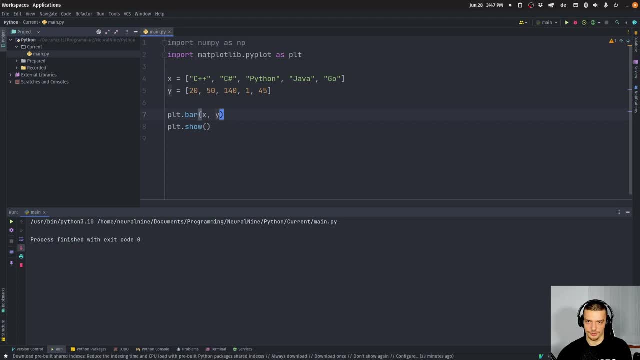 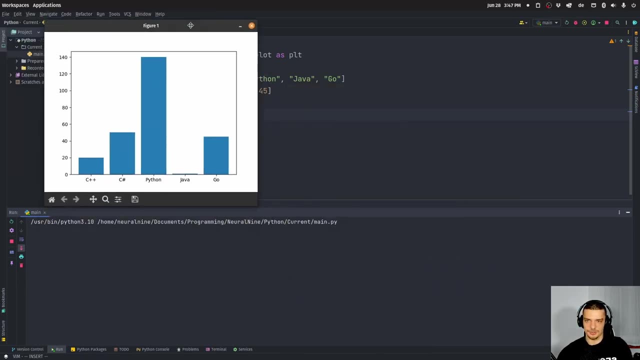 going to try that now. I think by default it should actually also work like that, But the function we use here is PLT dot bar and we can pass this. Oh, it actually works right out of the box. I thought that maybe I have to pass first of all some numerical values and then have to. 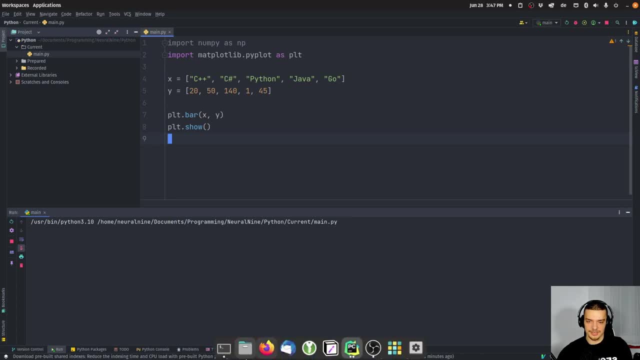 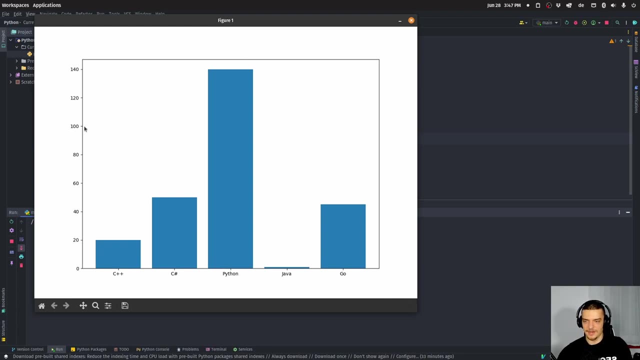 label them, But it actually works if you have just the text values right away. So you can see here. this is a simple bar chart. I just have the y values, the x values, And this makes sense, of course, for categorical data if I want to say: okay, how many people voted for Python? 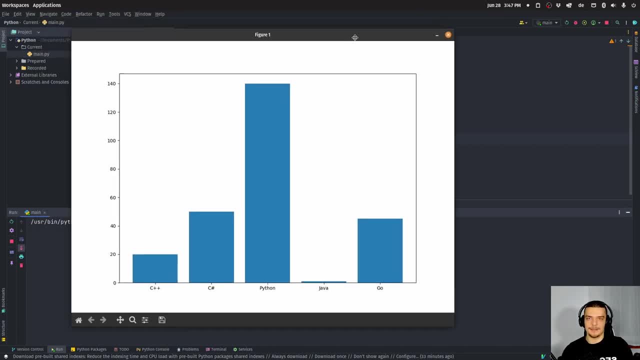 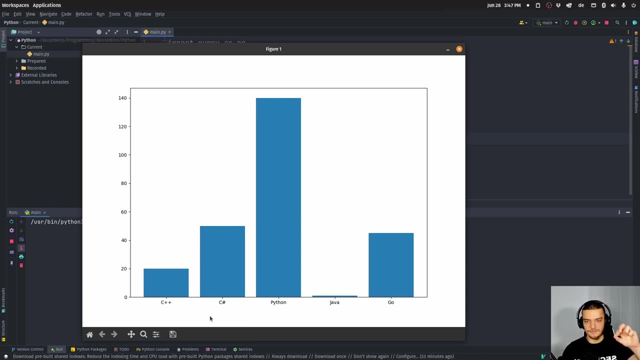 how many people voted for Java, and so on, Which is, of course, not to be confused with a histogram, which we're going to talk about here next, because a histogram is a statistical plot that shows the frequency of the values on the x axis, and not just categorical. 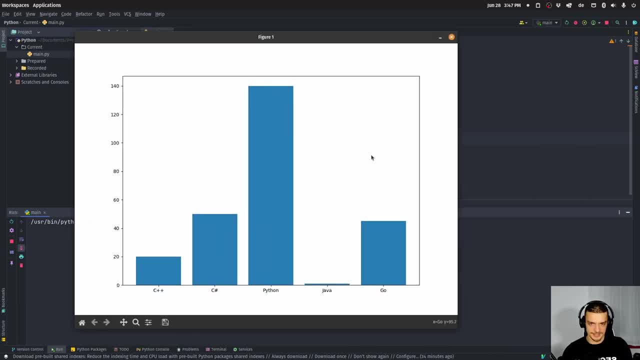 amounts here. So this is not a histogram, even though a lot of times histograms and bar charts look quite similar. One thing that you can remember: in most histograms, you're not going to have gaps. in most bar charts, you are going to have gaps. 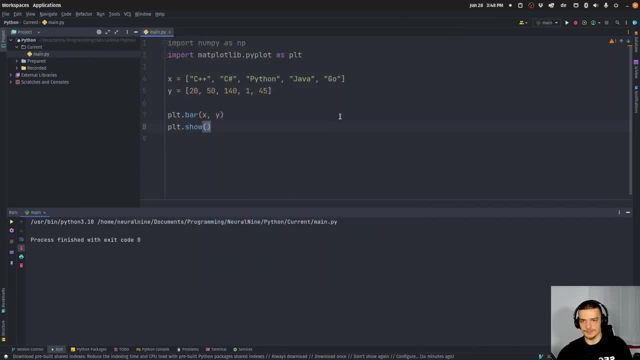 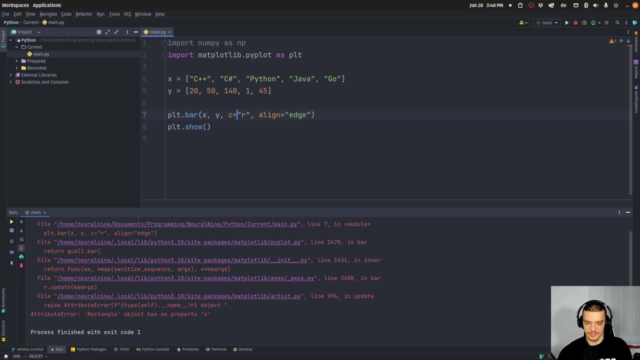 But yeah, here of course we can also do some, some styling. we can say, okay, color is going to be red. I can say also the alignment and say alignment equals edge. What's the problem here? Oh, actually, here we need to say color, not C. 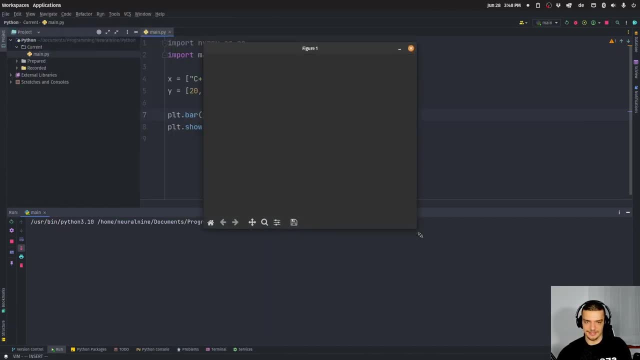 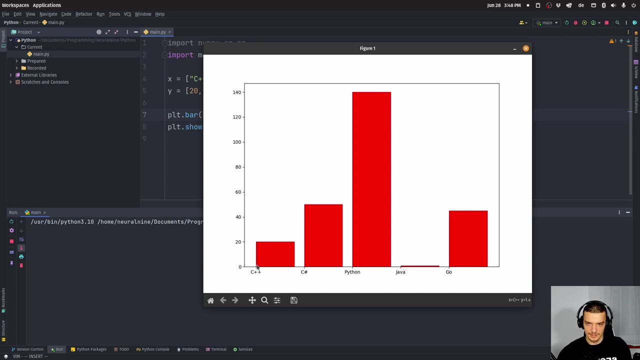 And alignment edge essentially tells us that the bar itself is going to start here, at the specific point. So here we have C plus plus. here's the point, And you can see the bar. it is at the right of C plus plus, And this is true for all the. 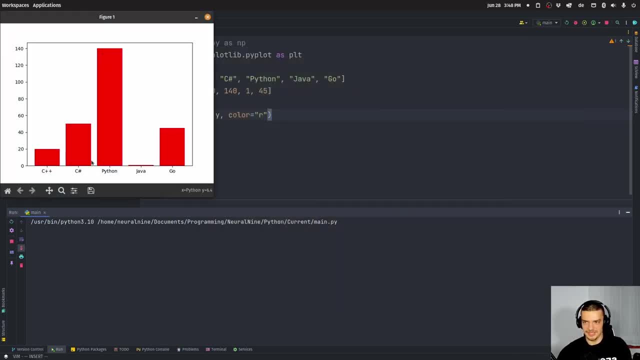 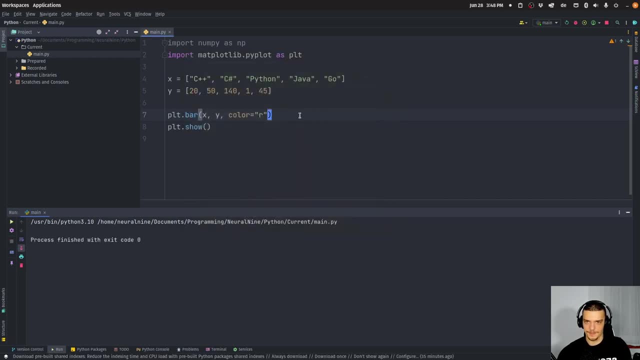 languages here. If I omit this parameter, you can see that the line is actually in the center of the bar chart. So we have the C plus plus point here and the bar above it centered. So this is something we can do: align equals edge. Then we can also say the width of the bars. 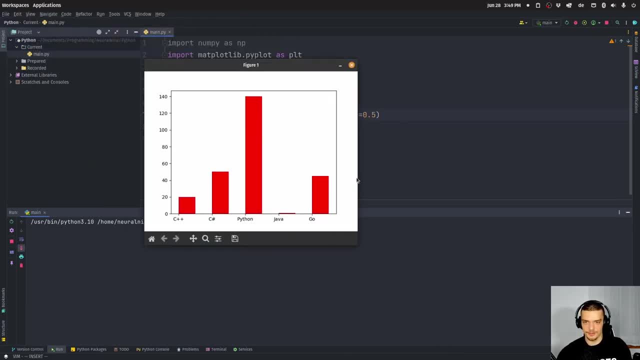 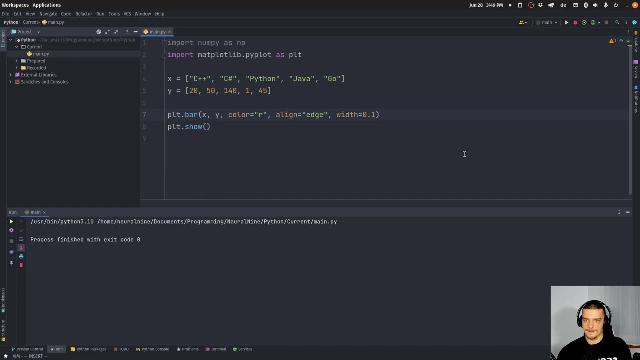 I'll be 0.5,, for example. and then you have some smaller, thinner bars. I can also say 0.1. And now you can see we have very slim bars. Then we can also say: we want to have a different edge. 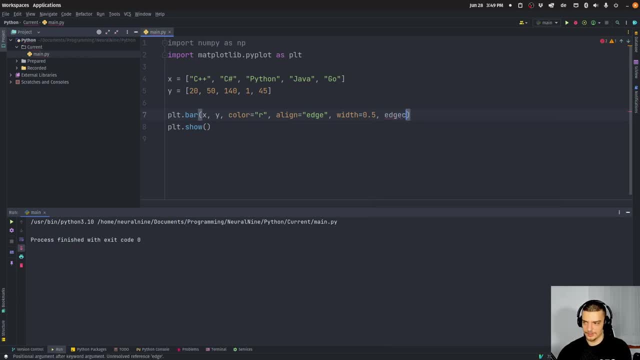 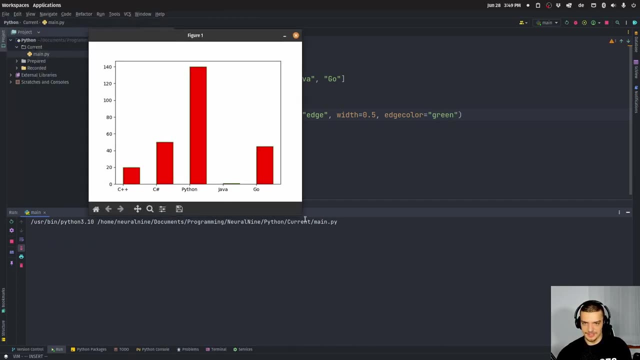 color. So let's say, the edge color is going to be green. And now you can see- I don't know if you can see that in the video So well, but you can see we have some green edges around the red bar. 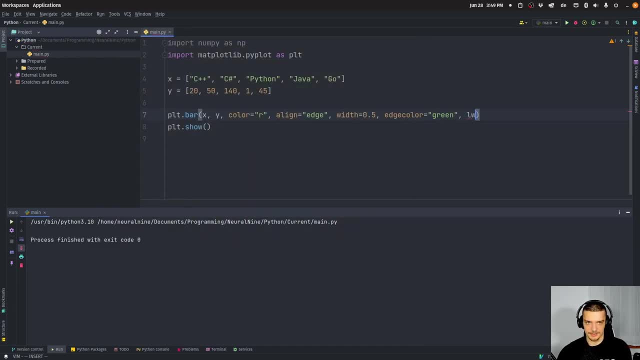 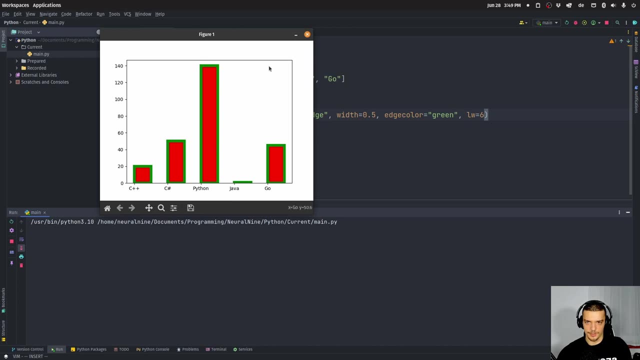 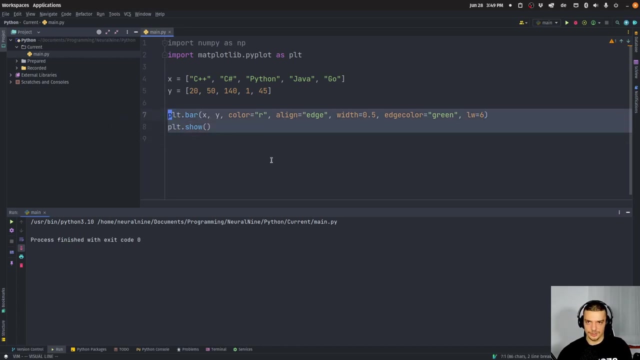 Now we should be able to see that better. If I say line width equals six, for example, there you go. Now you can see we have green lines around the red bars. So yeah, you have a bunch of styling options here as well. Now let's move on to the histograms that we just mentioned For this. 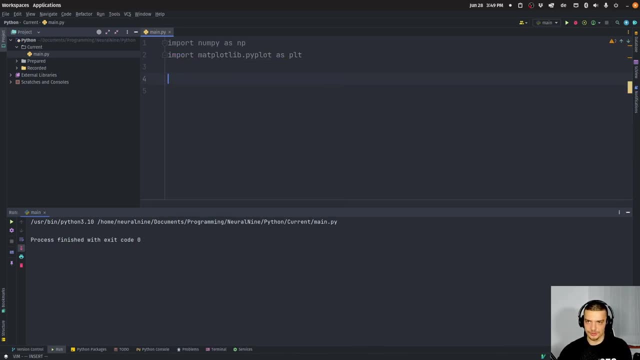 we're going to just generate some data here using a normal distribution. So I'm going to say ages, for example, equals numpy And random. We're actually not an umpire, sorry. NP, random and then normal, So a normal distribution. 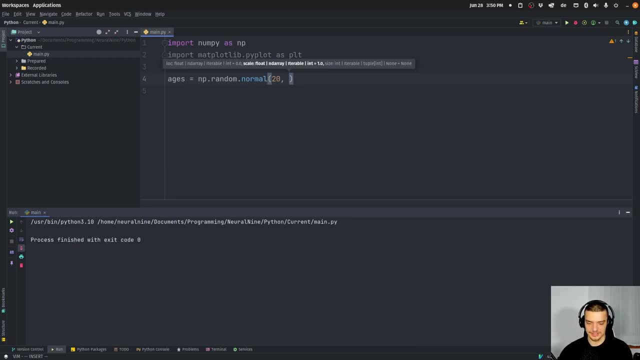 with a mean of 20 years old and a standard deviation of 1.5 years. And then we want to have 1000 different ages generated, So I can print that So that you can see what this looks like. We have a bunch of ages with a mean of 20.. And with a standard deviation of 1.5. 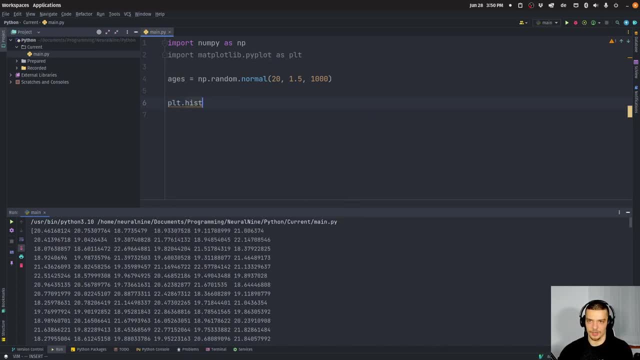 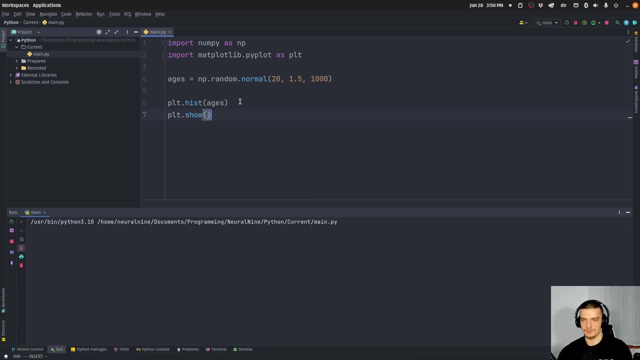 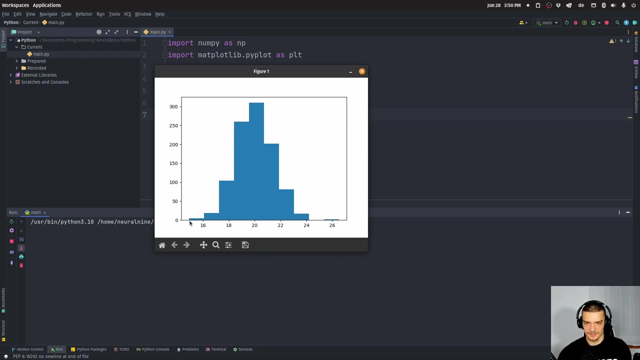 And now I can just go ahead and say PLT dot- histogram on the ages. So plot a histogram based on the ages And then PLT dot show the result. And now we have a histogram. you can see the mean here at 20. And you can see that we have, I think, the smallest value. 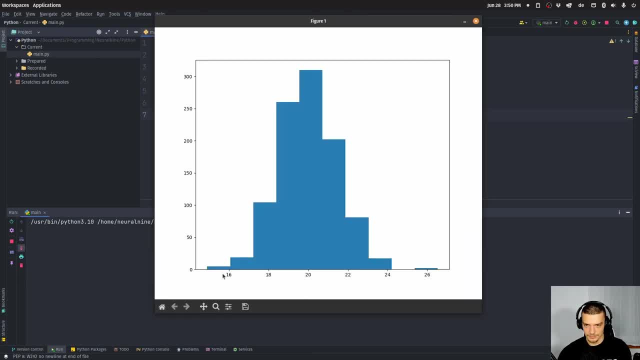 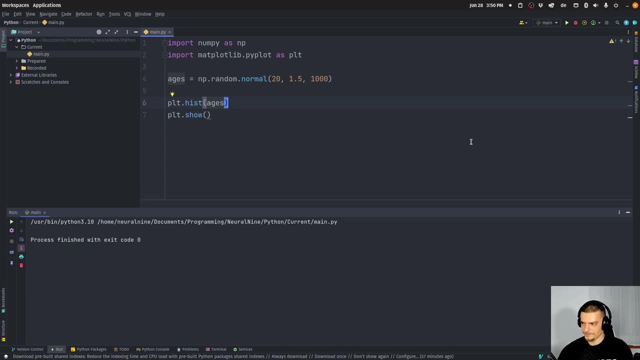 is somewhere around Yeah, 1615, something like that. And yeah, so it is the histogram. of course, here we can also change certain things. we can say that we can specify the bins so we can customize the bins manually. Now I'm not sure if we 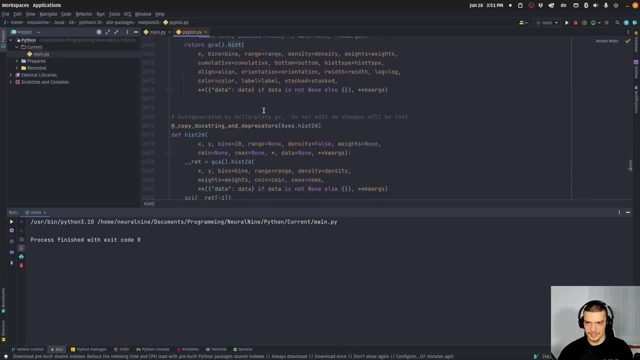 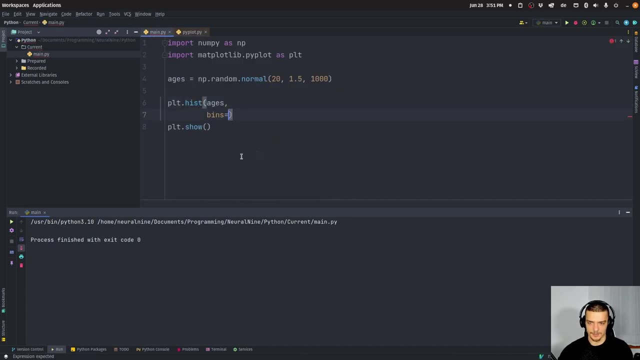 can also provide a number here. let me just look up the function, Because I know that in pandas we can set bin equal to a number and then we can get that many bins. I'm going to actually try this to see if this works. seems to actually also work here, Yeah. 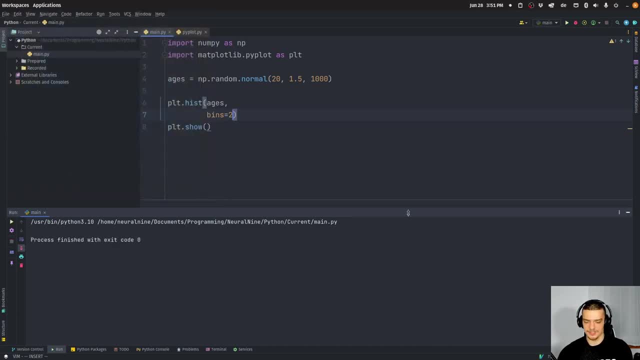 so we can do it like that: we can specify a number of bins. we can say 20 bins, and then we have 20, different bins in the histogram. but what we can also do is we can specify specific bins as a collection here. so i can say ages, dot, minimum up until 18 is going to be a bin, um, or actually from. 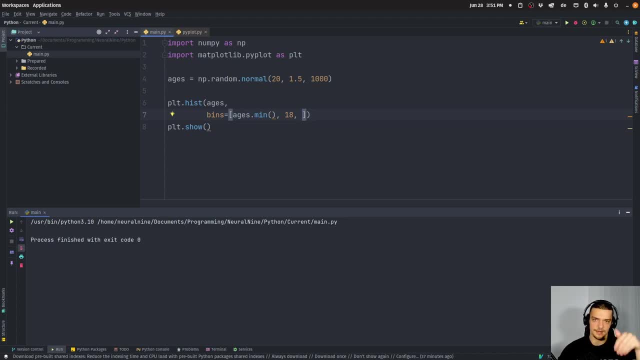 from zero up until ages min is going to be a bin. from ages min up until 18 is going to be a bin, from 18 up until 21, and then from 21 up until ages dot max up until the highest, uh, or actually this is already the minimum. so we only have this to this, to this, to this. that's the basic idea here. 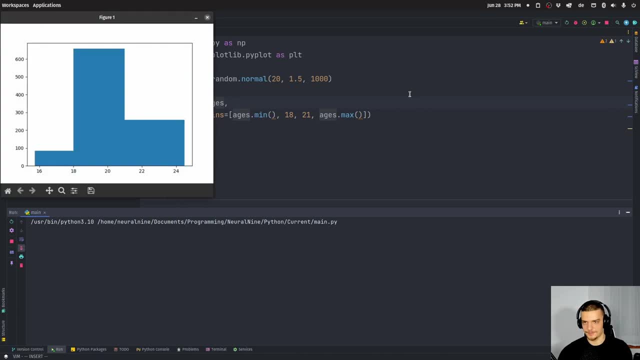 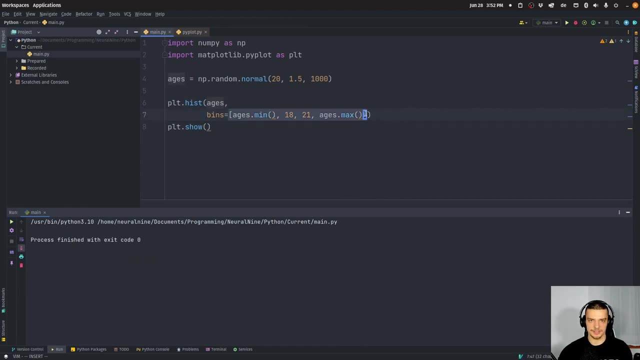 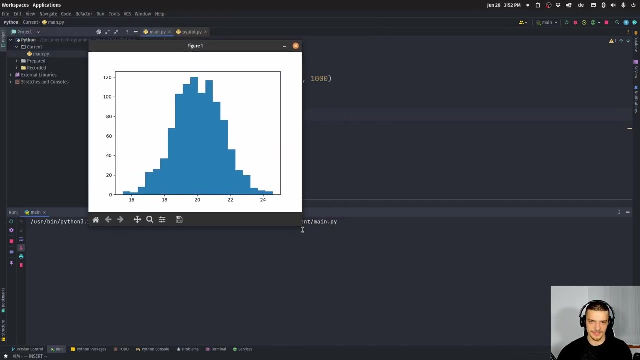 and i think actually: yeah, this works as you can see here. so you can either pass a number here or you can pass a collection of actual bins. so either you want to force it to have 20 different bins or you just specify the 20 different bins yourself. if you want to do that, um, we can also change the values a little bit. 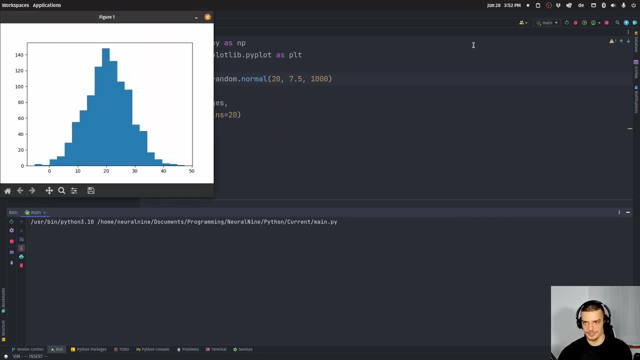 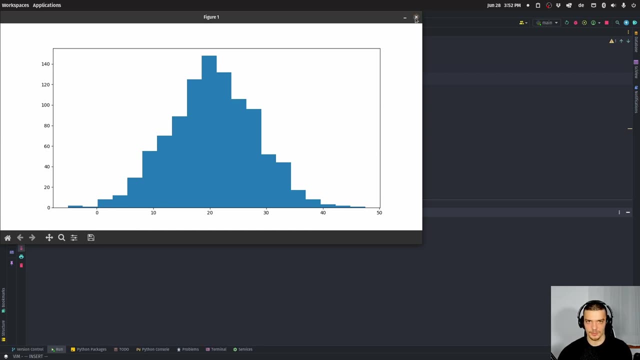 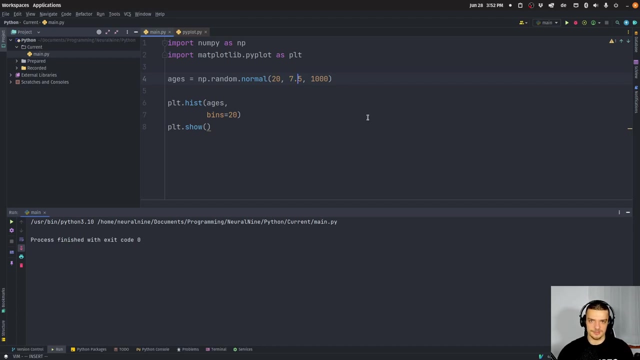 if i change the standard deviation to 7.5, for example, you can see that we now have values ranging: uh, actually we have values below zero, which is, of course, not what we want, but this is what happens when you have a normal distribution. with this standard deviation, it will probably go if you generate a thousand values. 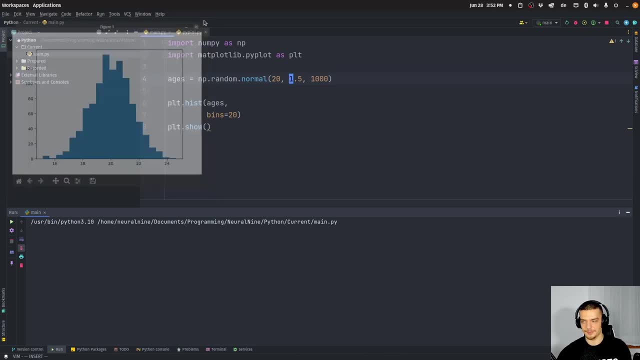 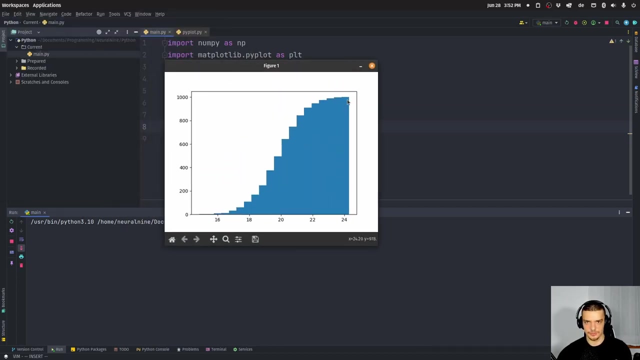 below zero, uh. but yeah, this is how we can plot histograms. we can also plot a cumulative uh histogram so we can say actually here cumulative equals true, to plot the cumulative distribution function. so you can see, it goes from zero to one thousand, basically telling us how many. 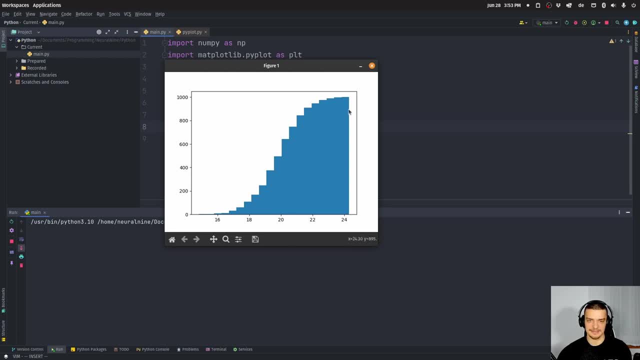 uh, people are at this or at this age or below this age. so, uh, the max age seems to be somewhere around 24 point something. uh, all, all of those people- 1 000 people, because we have 1 000 data points here- are below that h or equal to that h, and you can see, if we go to this age, only all the 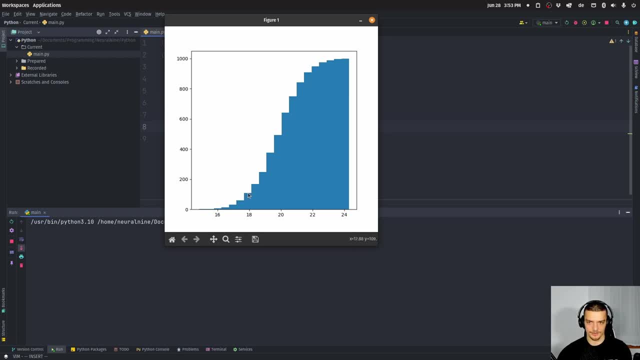 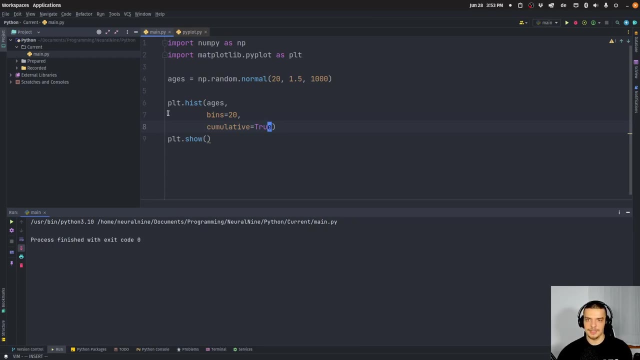 people, uh, below 18 are, or or how many do we have here? should be around 100. around 100 people are of age 18 or below. that's how you read. that function all right, so, uh, what else could we do? we can also do a pie chart. sometimes we have um independent plots, so sometimes we have independent categories. 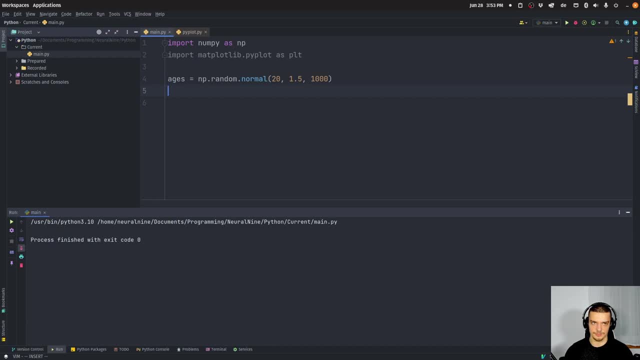 so, for example, you're either that or something else. you don't overlap necessarily. and then it makes sense to show the ratio of the different people, and to do that we can use a pie chart. so so let's say, this time we don't ask for just. 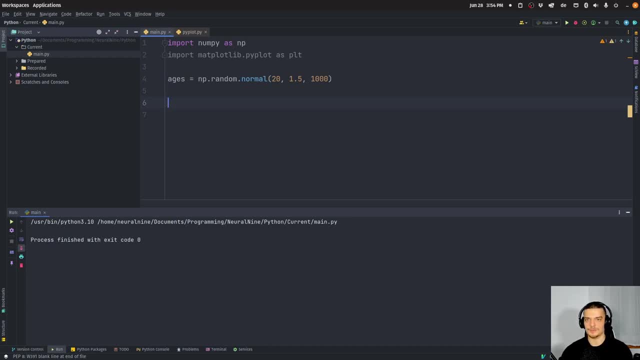 programming languages in general, which programming language do you use? but we want to know, okay, which is the one programming language which is your favorite. so you can only have one. if your favorite programming language is python, it cannot be c plus plus at the same time. so we can do that by saying: 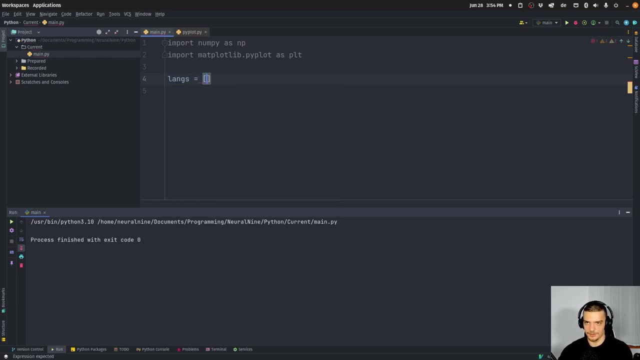 that here: um c plus plus instead of Mus calc islands c. you can do that no matter which programming language is there. so um she. so we need to do this again. languages is going to be equal to python c plus plus java c and go. i think before we had c sharp. so let's. 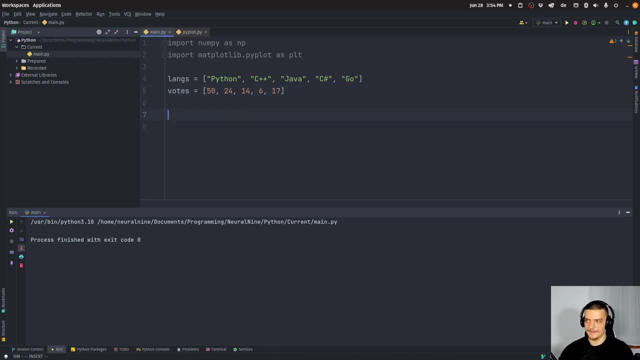 six for C sharp and 17 for go, And then we're going to just say PLT pi. I'm going to have the votes And the labels for these votes are going to be the languages PLT show to see the result. 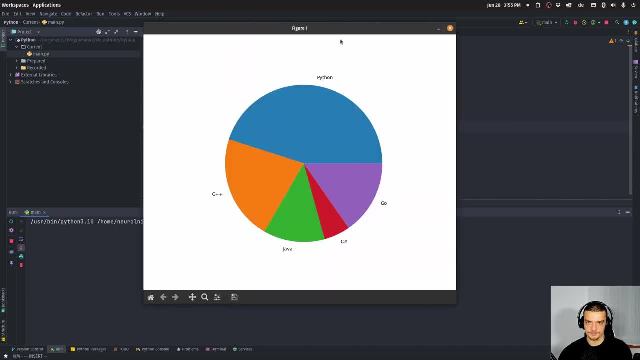 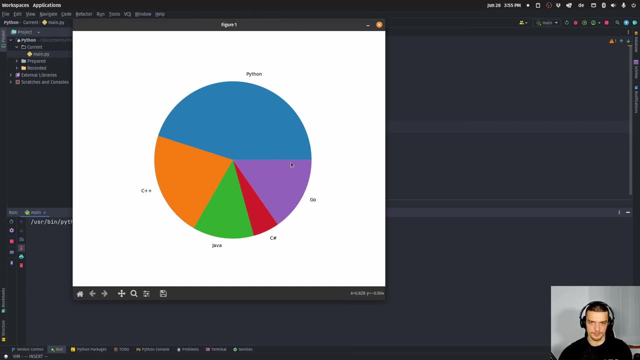 And now you can see we have a pie chart And you can see we have: Python is blue, C++ is orange, green is Java, red is C, sharp and purple is go. And of course this chart makes sense if the 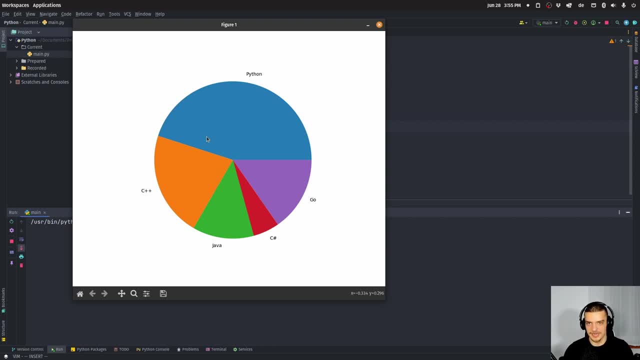 communities are not overlapping. So if the question is, for example, how many of you guys use Python, How many of you guys use C++, A person using Python might also use C++. But if that is the case, if that is our question here, this plot doesn't make a lot of sense. 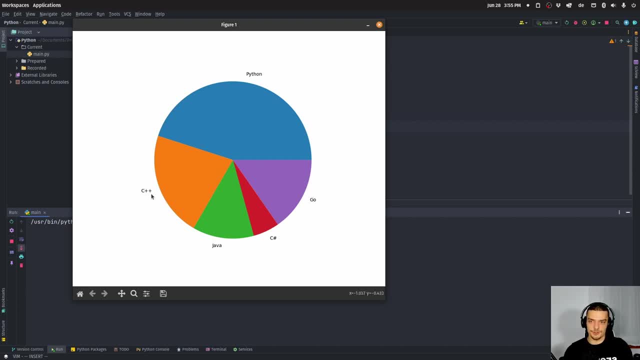 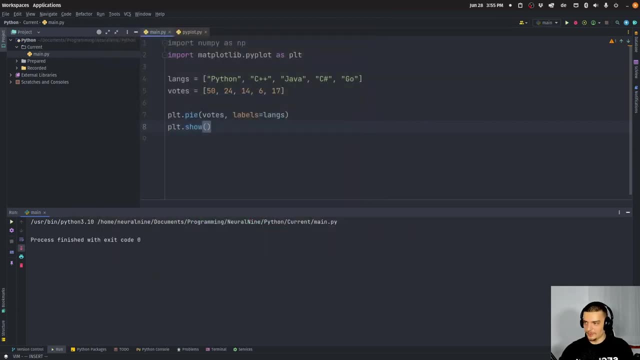 because it shows how many people use Python versus C++ and not it shouldn't be overlapping when you use it In the optimal case. Now, here we do have a lot of customization options, So, for example, one thing that we can do is we can explode certain pieces So we can take certain pieces. 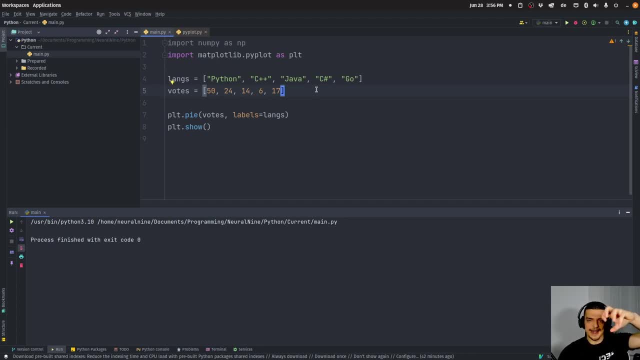 from the chart and we can pull them out of the pie chart a little bit to highlight them, for example. So we can say: here explodes equals, and then we can say: for Python- maybe we want to pull it out a little bit- 0.3. And the rest stays where it is, So 000.. 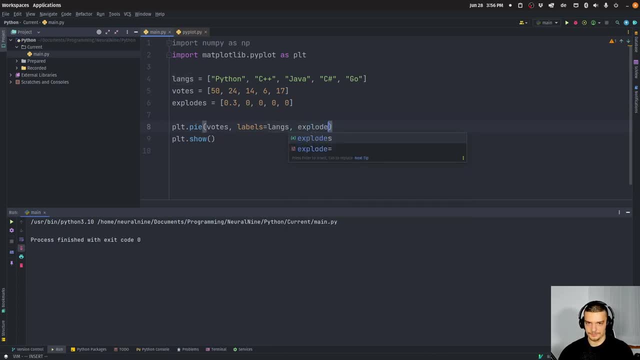 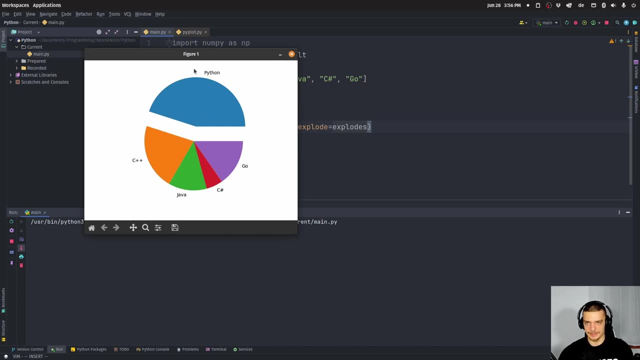 And then we can say: here, explode equals explodes, And what this results in is that we pull Python out a little bit. or maybe we want to do that with C sharp, because it's the smallest number, So we'd go to. 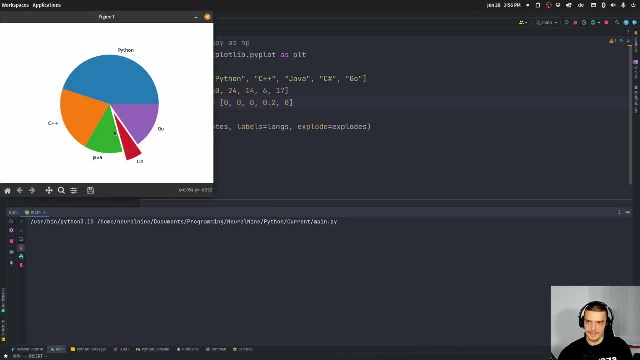 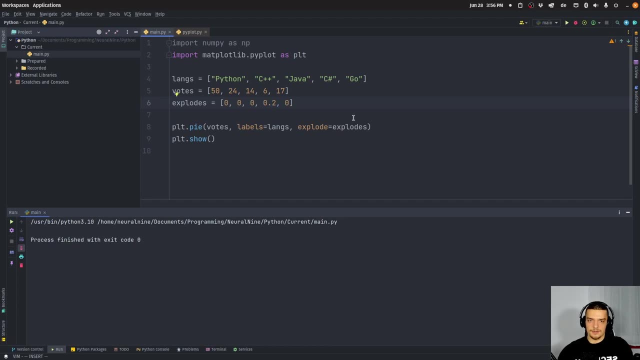 that position here and I would say 0.2, for example, And now you can see it's dragged out of the, out of the pie chart a little bit. Other customization options: of course you can also write the percentage inside of the or outside of the pie chart by saying auto: percent equals, and then you can. 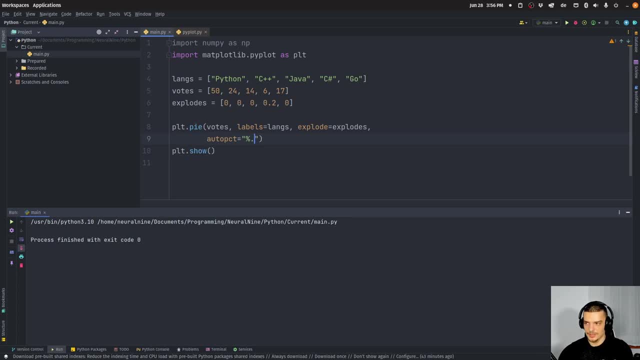 specify a format, for example percent two or percent point two F. so two decimal places percent percent. So we have these two percentage signs And inside we have a floating point number up until two decimal places percent. I think that already is enough to show the percentages here. 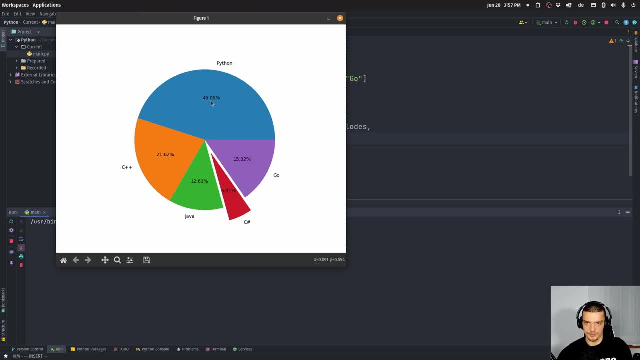 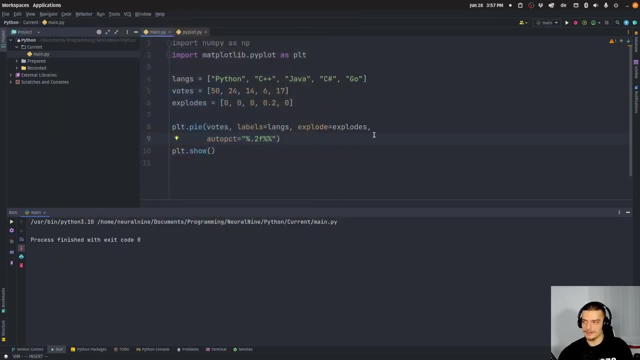 as you can see. So 45,, 0.05% Python for, or 5.41% for C sharp. And then of course we can also specify the distance of the percentage. So we can say: percentage distance equals to 0.8.. For example, to not have it. 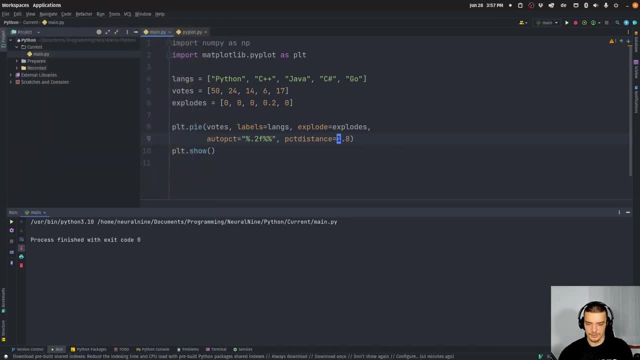 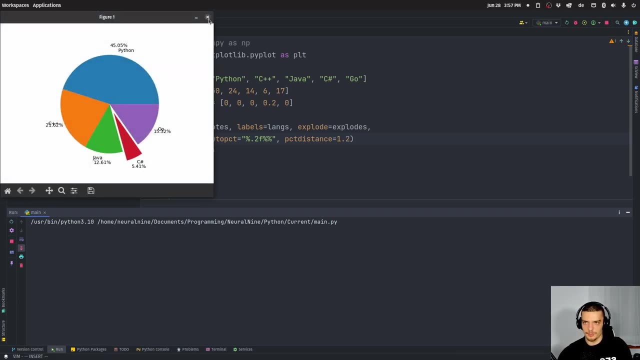 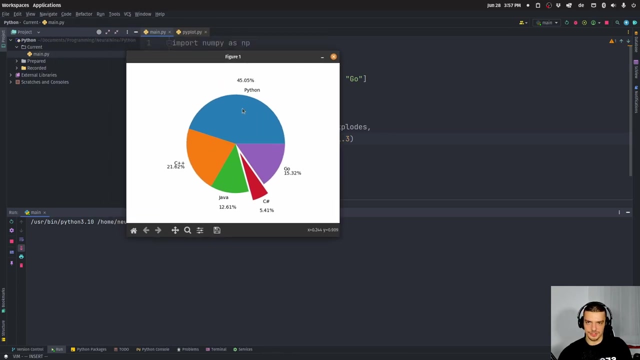 completely in the middle. we can also increase that. actually, to think 1.8 is too much, maybe we should go with 1.2.. Maybe 1.3.. 90 degrees- Yeah, I mean it's fine. So we have the percentages now distanced from the center. 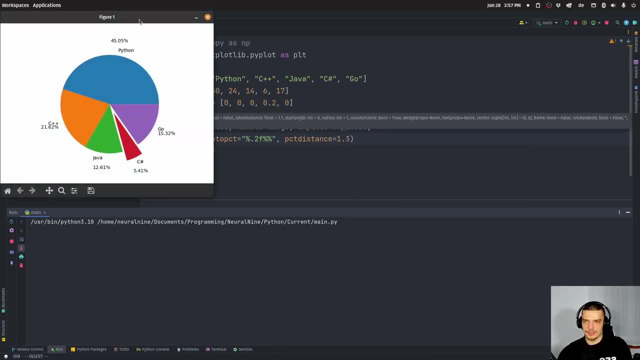 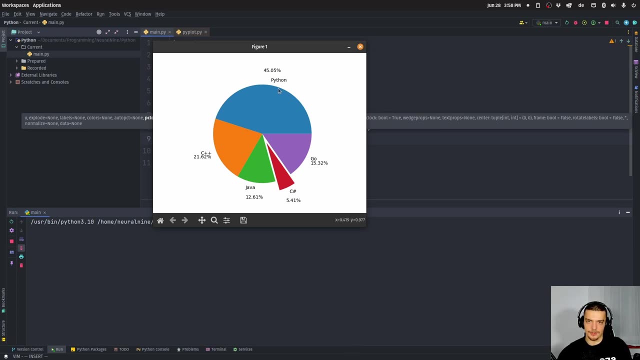 And what we can also do is we can choose a starting angle. So when you look at this, you can see that the histogram or not histogram sort of pie chart starts here and then it goes full circle. you can also start it at at 90 degrees. So if you go, this is zero, 90 degrees is here, So you can. 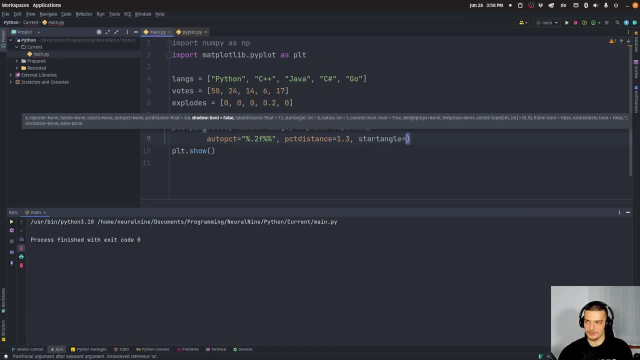 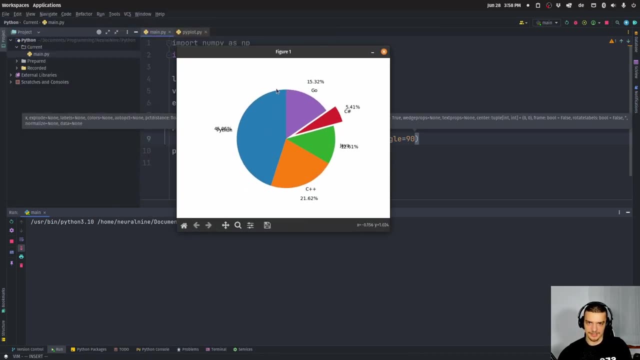 start it At the top And you do that by saying start angle equals 90. And then you can see it starts actually here and it seems to go actually backwards. So it seems to go counterclockwise to the left. 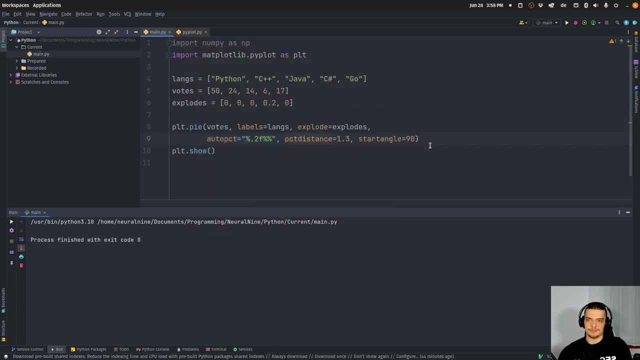 but it starts at the top here. So those are some customization options for the pie chart. Now the last plot type that we're going to look at is the box plot. So the box plot diagram, basically a statistical plot, showing you the different quartiles, showing you the median. 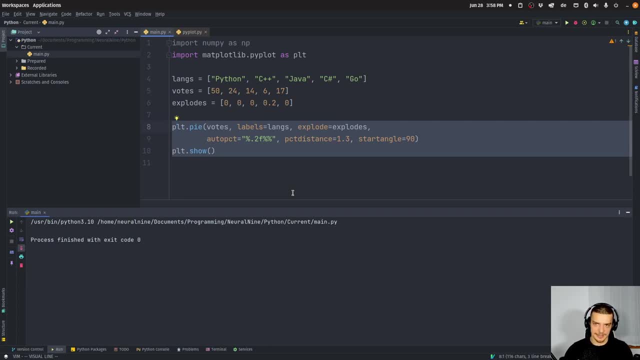 showing you the maximum and the minimum and showing you outliers. So for this, what we're going to do is we're going to again do a normal distribution. we're going to say, this time we have heights, heights is going to be NP, random, dot, normal, And we're going to have a normal. 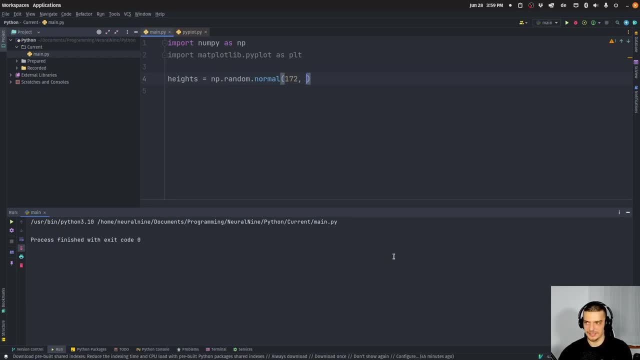 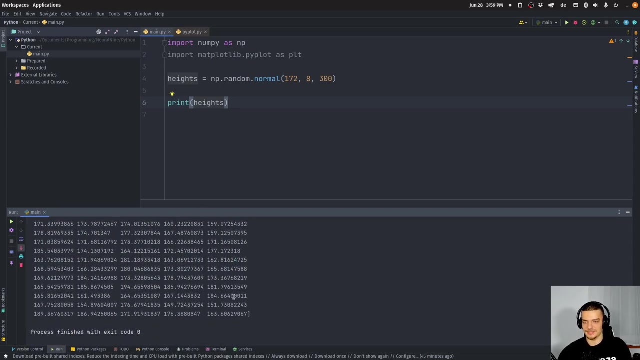 distribution, with 172 centimeters as default, eight centimeters as the standard deviation, and we're going to generate 300 heights. So, again, this is what the numbers look like. Whether that's realistic or not doesn't really matter, But this is what the numbers look like, And what we're going to do now is we're going to 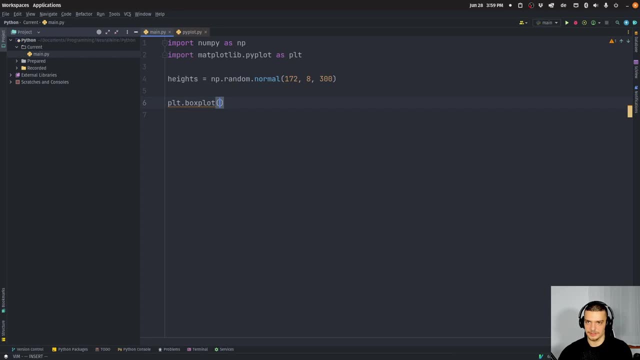 plot, a box plot, by saying box plot heights and then PLT show And you can see here now we have a box plot. And how do you read a box plot? you have the median here, the second quartile, you have the third, the fourth, the fifth, the sixth, the seventh, the eighth, the seventh, the sixth. 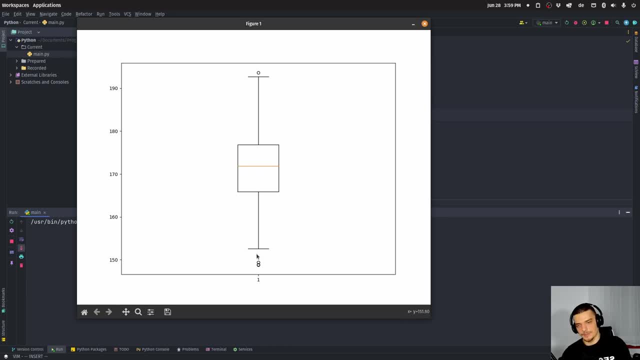 the seventh, the eighth, the sixth, the seventh, the seventh, the seventh, the eighth, the sixth, the eighth, the ninth, the sixth, the seventh, the eighth, the seventh, the seventh, the eighth quartile and basically you have the minimum value, the maximum value and all these dots are. 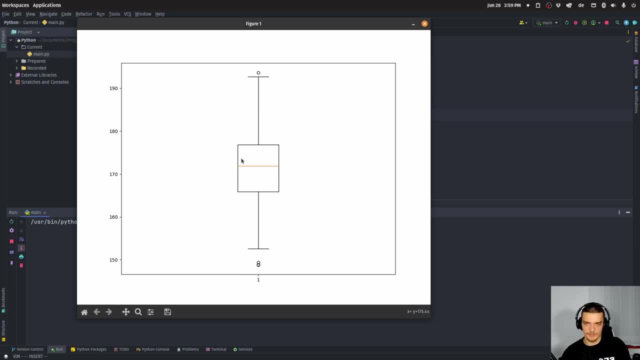 outliers, That's how you read it- And within these boxes here. so from here to here, you have equally as many values as here. The reason this box is wider is because the values are further apart. So it goes from here to here, And here's an extreme example. So the values range from here. 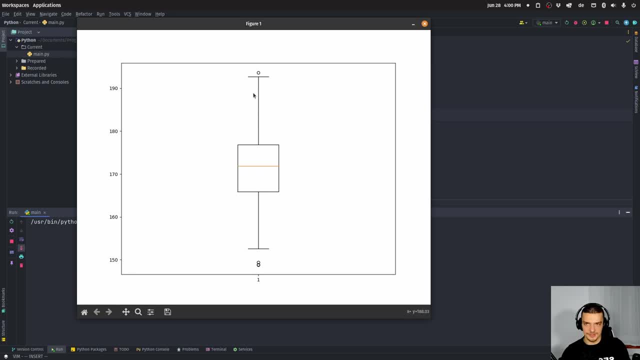 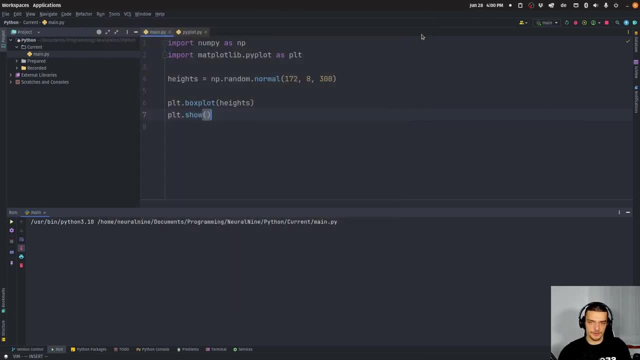 to here, But it's the same amount of values that we have as here, it's just that the range is wider. That's the basic idea for box plot And this can also be useful to explore the data to see how is the distribution of a certain feature in the data science process. 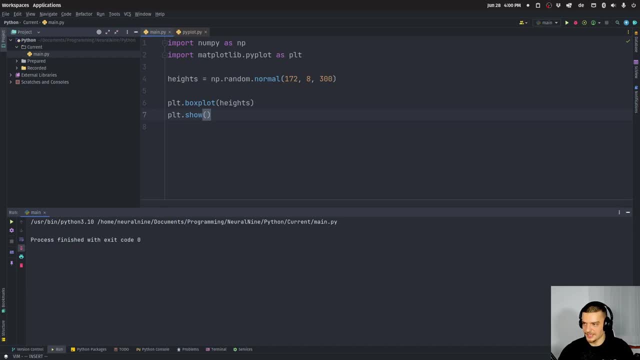 So actually, I'm going to copy paste an example that I have here on my second screen, because I prepared some code here And I'm going to show you that this is the case. So I'm going to copy that real quick. I'm going to paste it here. We have artificially created sections here for the box plot. 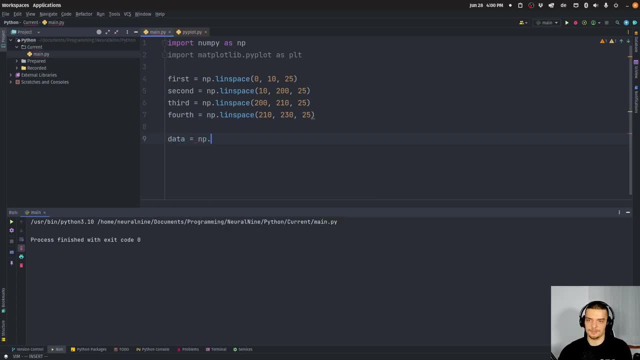 I'm going to copy, or actually I'm going to write this myself: data equals NP concatenate. we're going to just concatenate these numpy arrays here: first, second, third and fourth, And this needs to be put into brackets, all of this. Then we're going to just say PLT, box plot. 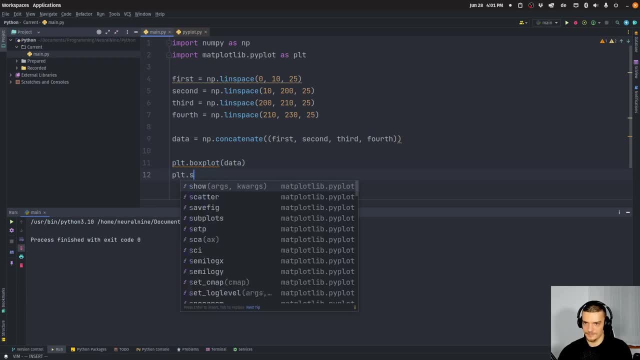 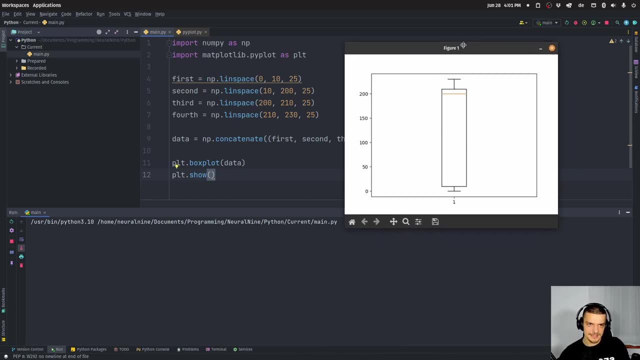 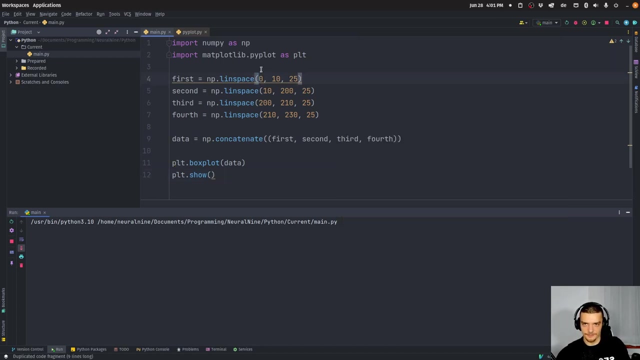 data PLT show And you can see now that we have a pretty extreme box plot, meaning that we have a very wide range of values in here. This is, I think, the second one, So you can see in the first one we have values from zero to 10.. 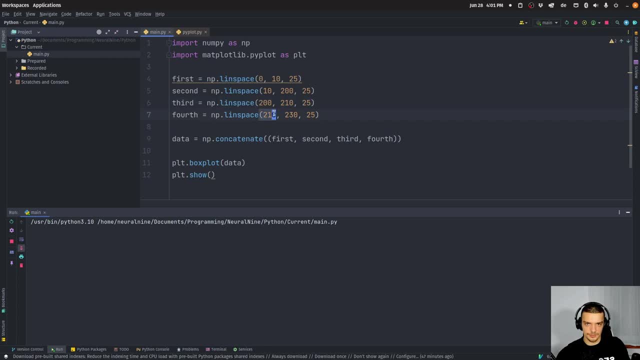 In the third one we have 200 to 210. And here we have 210 to 200- 230. But here we have from 10 to 200, which is a wide range. But you can see that all of these have 25 values, And this is. 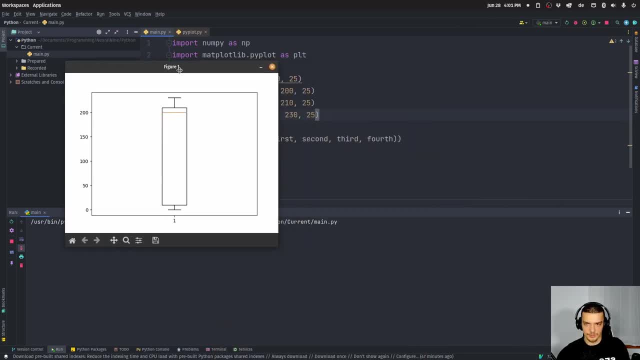 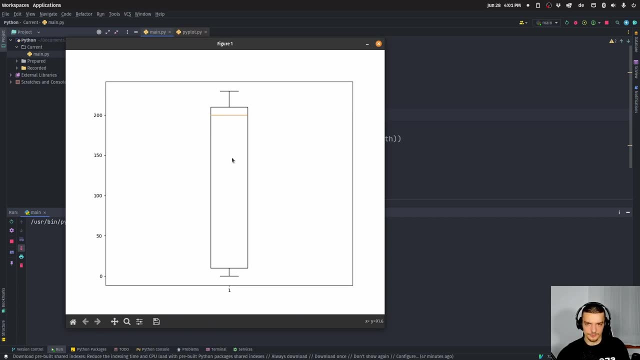 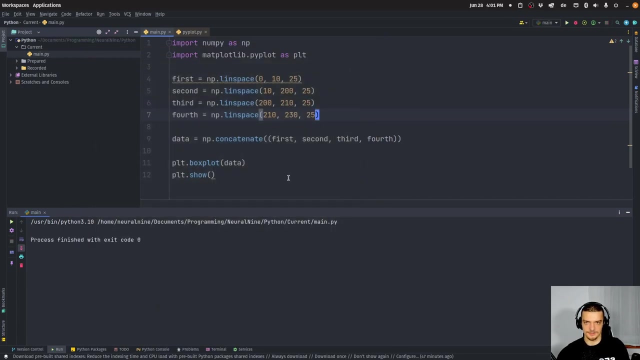 why we have- where is it- the box plot that we have here? Because the amount of values that we have from here to here is the same amount of values that we have from here to here, But the range here is much wider. So, yeah, this is the effect that such numbers produce in the 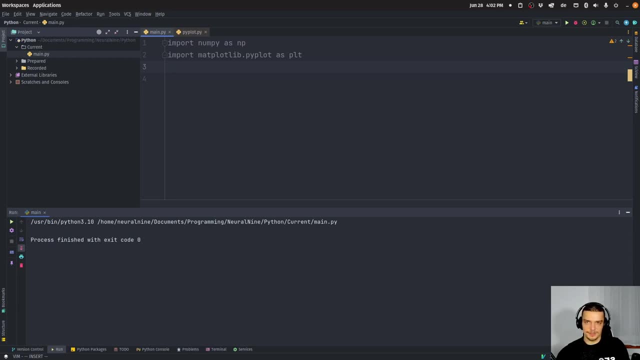 box plot. Alright, so those are some basic plot types. the list is not complete. you can always come up with some fancy plots. there are a lot of plots that we don't cover here today because I don't want to just go. 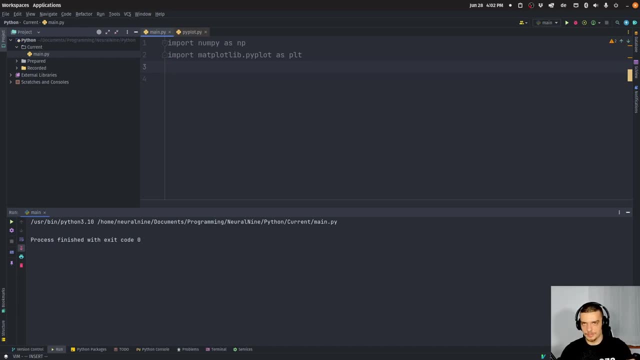 Through all the different types of plots that we have. those are very important plots. you should know about them. But of course you have also some more advanced plots, like heatmaps and like crazy silhouette plots and stuff like that. But of course it's also makes sense to 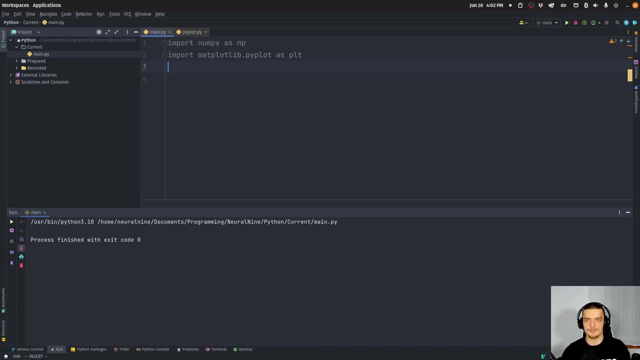 sometimes use some more advanced packages like seaborne to plot heatmaps, because they make it easier than when you do it every when, when you do everything from scratch in matplotlib. But that's it for the plot types. Now we're going to move on to 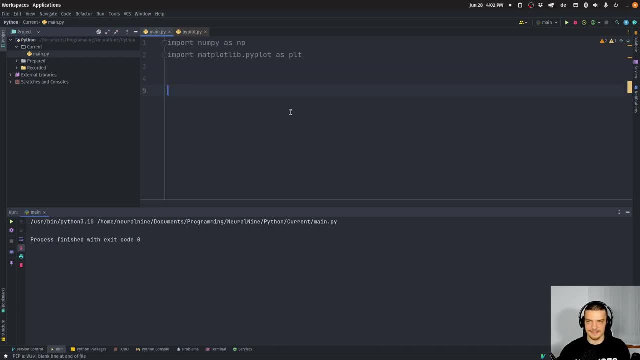 customization of axes and titles and stuff like that, Because all the plots we had up until this point were just the plot itself, And maybe we had some text here and there, But the plot wasn't telling us what it's actually visualizing. So what we're going to do now is we're going to say here: 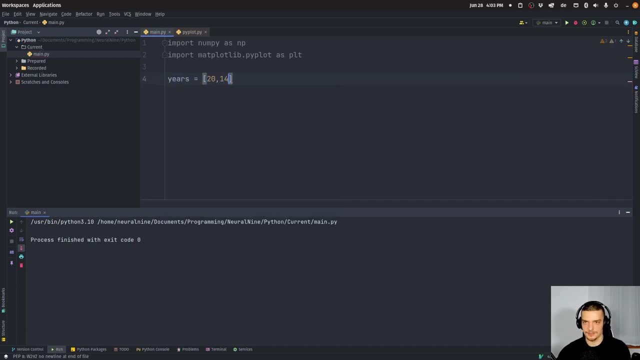 some sample data: years equals 2014.. Actually, let me copy this as well, because the tutorial should not be about just typing stuff. So we just copy this here And then we're going to paste this year. So what we have here? some 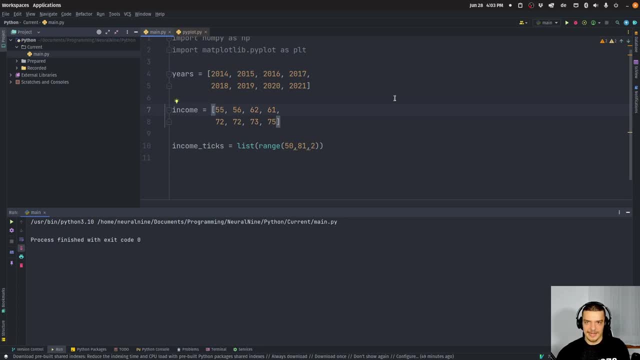 sample data. we have years, we have income and we have income ticks. So income ticks are just for for the, for the y, for 40 for the y axis, so that we have the actual ticks that we want. to plot, Mike Antony, over here, I'm going to show you here what this means in the second. but we can just 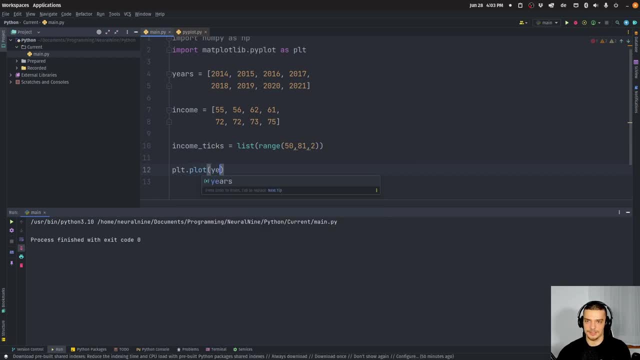 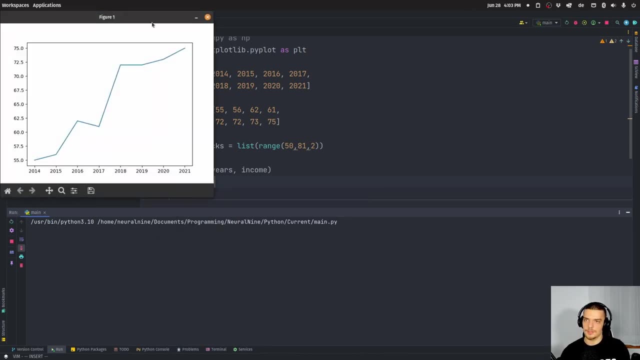 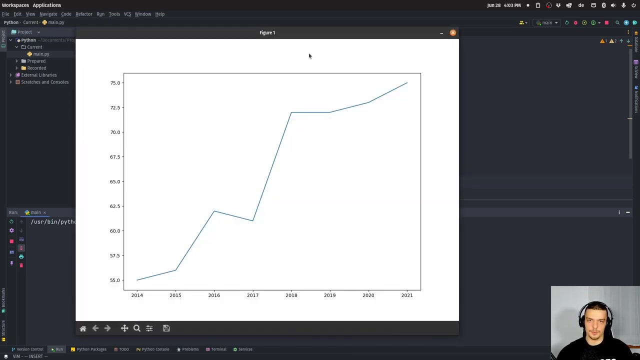 go ahead now and we can say PLT, dot, plot, years and income. Of course we need to show the plot. There you go, you can see the income is rising, which is optimal. But now we want to do some customizations here. So, first of all, what we want to do is want to have a title actually explaining 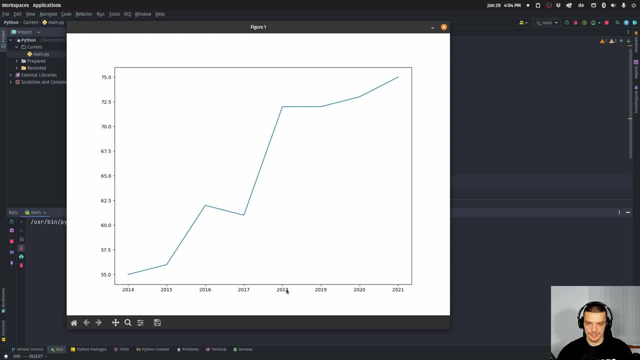 what we're visualizing here, because we can see, okay, we have some years down here, we can assume that those are years, we don't actually know that, And then we have some values here, But what is this actually? So the idea is that those are years, those are numbers of income. So this is US dollar. 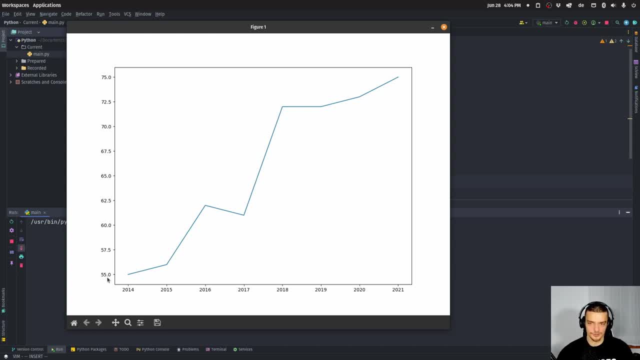 income in 1000.. So it's not $55 per year, it's actually $55,000 per year. The whole chart is the income of john, let's say, And this doesn't tell us much yet. So we just have a line we have. 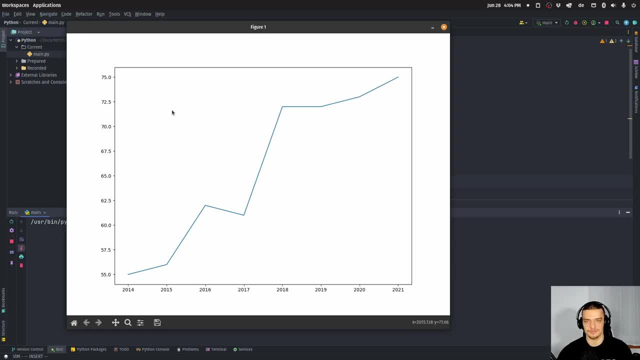 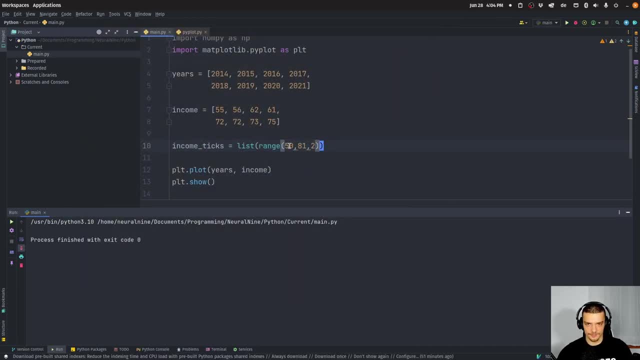 probably some years, and we have some values on the left side. we want to make this more explicit, want to actually explain what's happening in the chart And this is actually why we have these income ticks here. we just have from 50 to 81. So this includes all of these. 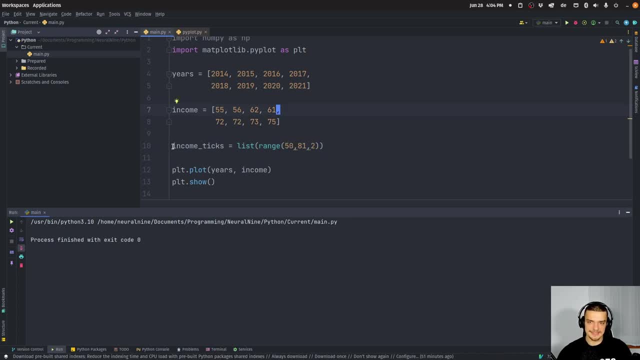 values this range and want to take these income ticks to actually format them into something saying that this is in 1000s US dollars. So we have not 50, but we have 50,000 US dollars. So what we're? 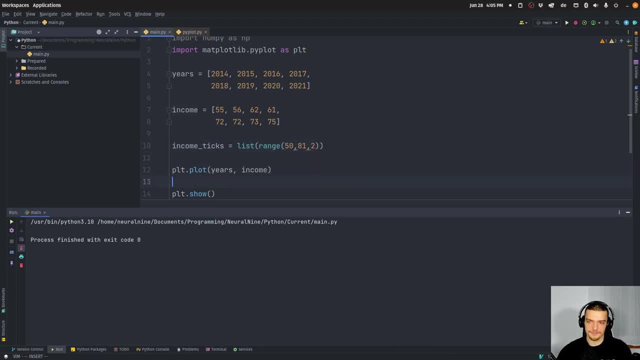 going to do here is we're going to say: after or before, plotting doesn't really matter. we're going to say PLT dot. title is the first thing that we want to say. So we're going to say PLT dot. title is the first thing that we want to say. So we're going to say PLT dot, title, dot, title. Okay, so if I 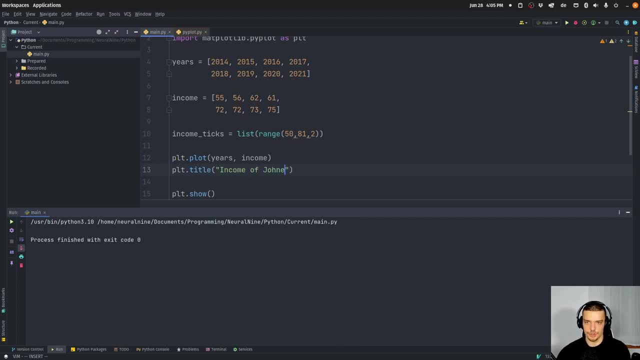 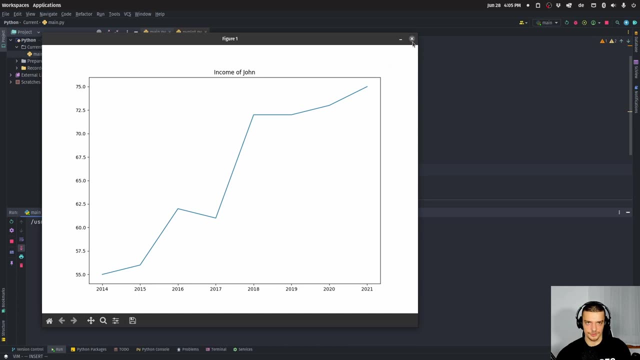 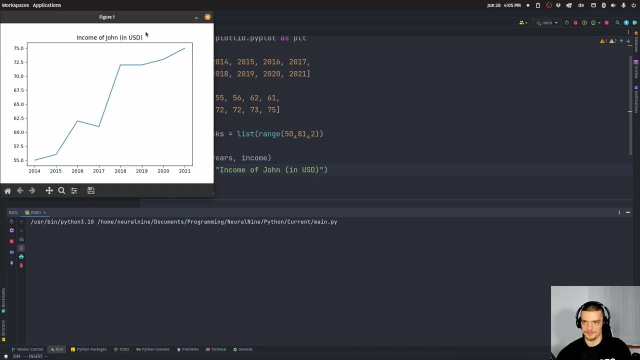 see here: income of john. this is what we're going to see at the top here. So this tells us actually that this graph is the income of john, And maybe I want to add in us dollars or something like that. There you go Now for every access for the x and the y axis, we can also specify a label. 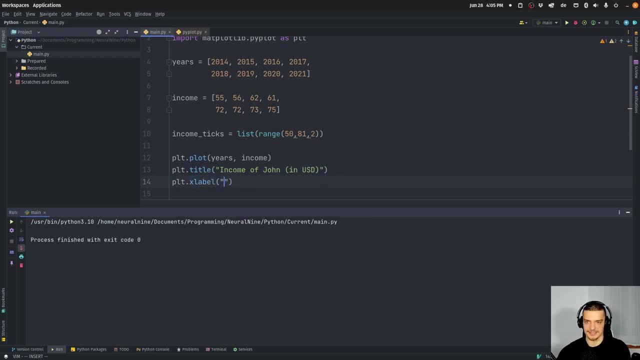 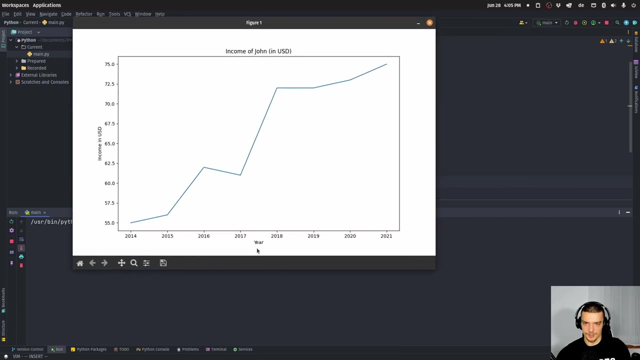 so I can say PLT x label for the x axis axis is year And PLT y label is income in US dollars. So we have the year, we have the income in US dollars and we have the income of john as a title here. Now, of course this is not entirely. 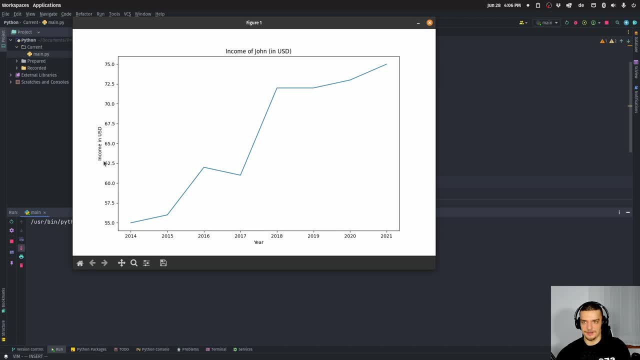 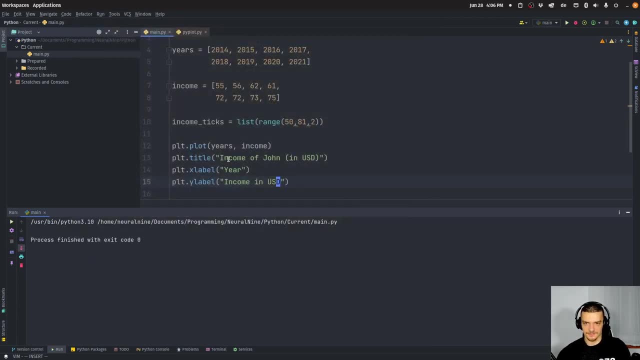 correct yet because we have not 55 $55 of income. we need to add a K here to make this correct, And maybe I should also specify that this is the yearly income in US dollars. Now, to actually format the y ticks, Now we use the income ticks we generated here again, just to explain this. 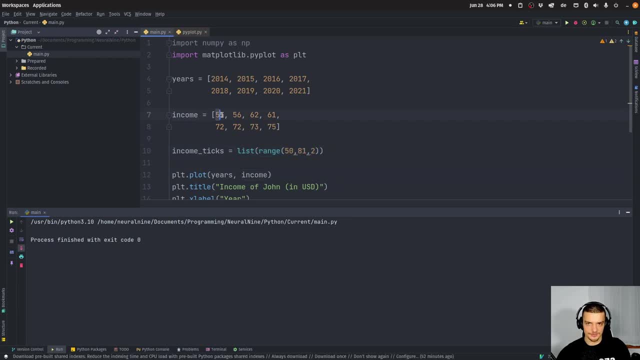 the only reason I generated like this is because we have values from 55 to 75. And if I want to plot, if I want to show all the ticks between 50 and 81, I can- just I can- include all of this. 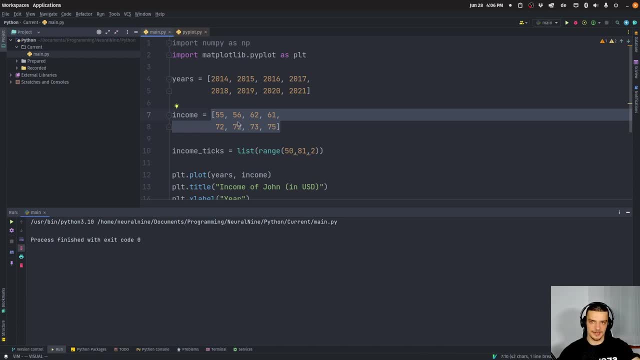 range here And I have more than just the data that I want to show. So I want to go a little bit below the minimum and a little bit above the maximum. So instead of doing 55 and 75, I go with 50 and 80. And I use 81 because that's then not included. But yeah, what I can do now is I can say: 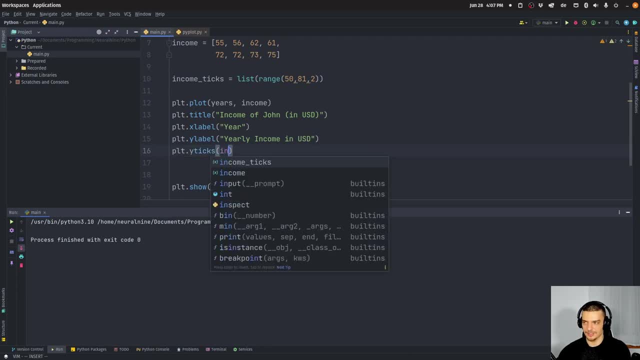 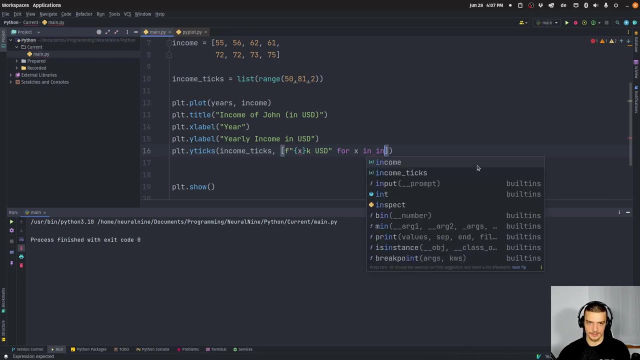 PLT, dot y ticks And I can say here income ticks for the actual values, And then we're going to specify a list comprehension here in F string which says sum value x and then k US dollars for x in income ticks. So this is the logic here And what happens. 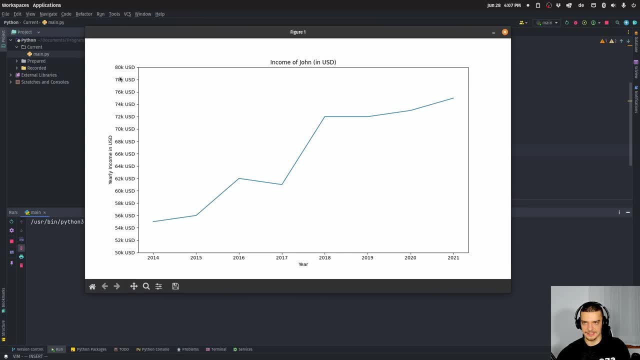 here now. as you can see, on the y axis we have now 80k US dollars, 78k US dollars, and so on and so forth. So that is now the correct representation. or maybe you want to do it with a dollar symbol. 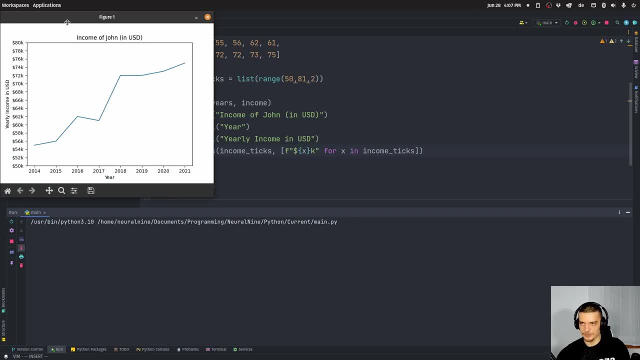 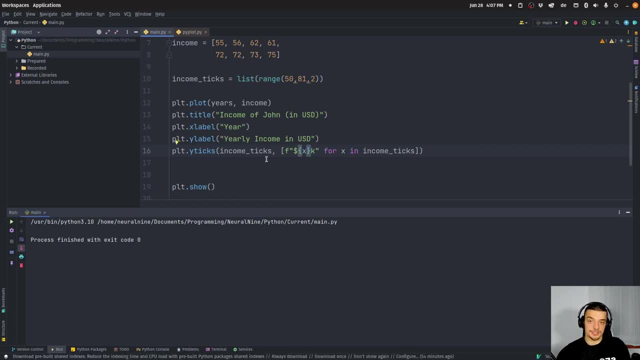 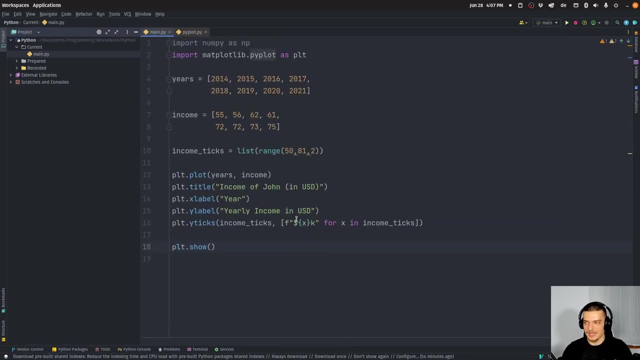 like that. This also works, of course. Um, and yeah, this is how you can, or just how you should- also customize your plots, because you don't want to just plot something and not explain what it is you want to show in the plot itself: What is this exactly? Now, what we can also do here is we can style the 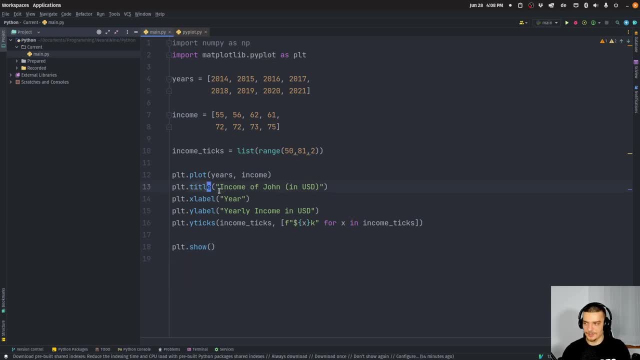 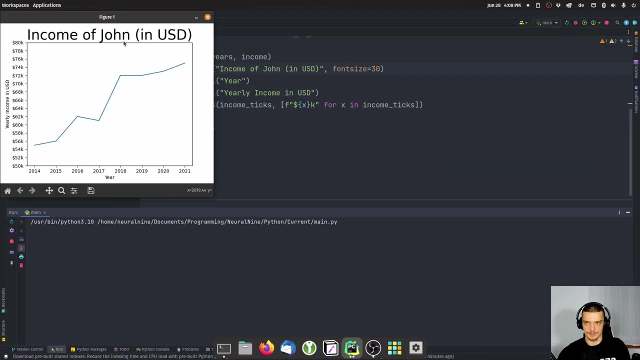 individual elements. we cannot just say, okay, there's a title, there's a label, we can also set the font size, the font family and stuff like that. So I can go ahead and say here for the title, font size of 30,, which is quite big, But you can see that this then, sorry, this then transforms the. 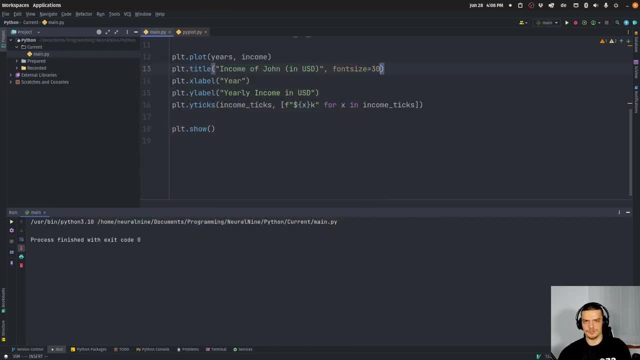 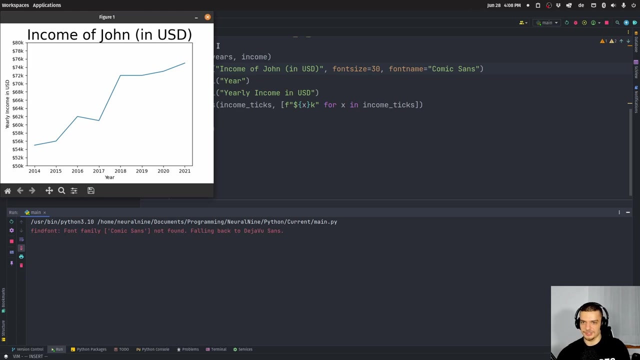 title into a very big title, And I can also change the font family, Or actually the font name is the keyword. I can change this to Arial. I'm not sure if this is the default. maybe we can change it to comic sans. No, actually, I don't have this on my system. 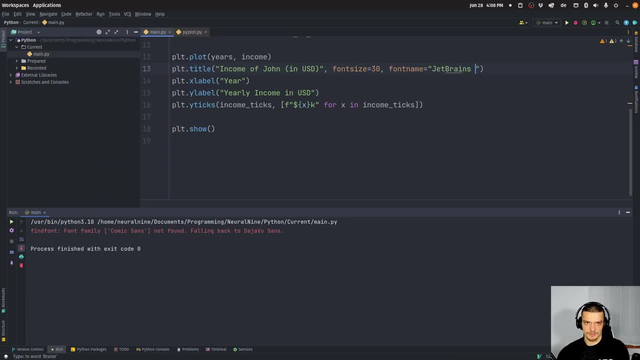 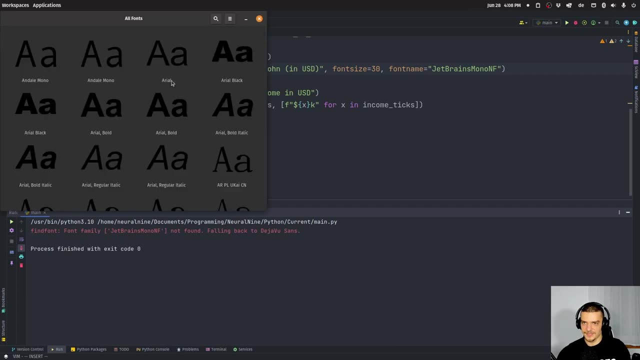 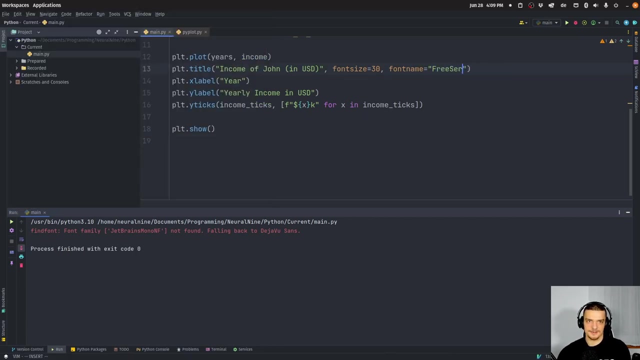 This is a font that I have on my system. jet brains Mono nerd font doesn't work as well. We just check out the fonts. Let's pick a font that's easy to recognize, Maybe something like something with a simple name, free serif, maybe that. There you go. You can see I can change the font family here to font. 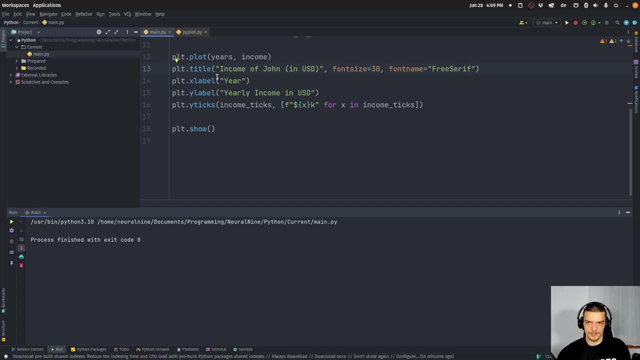 name, And this can be done for all the different functions here. I can do that with x label as well, with y label as well. Just use the same parameters: font size, font name- And this is going to change the styling of the actual labels. 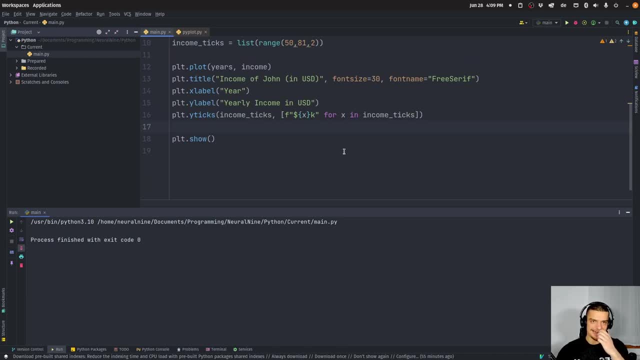 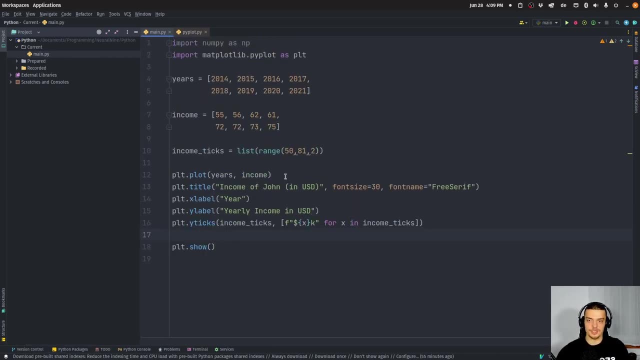 Now, what we can also do is we can also add a legend to the plot. So maybe you have different things that you want to plot, And this is also something you can do. by the way, you can just call the plot function multiple times And when you do, 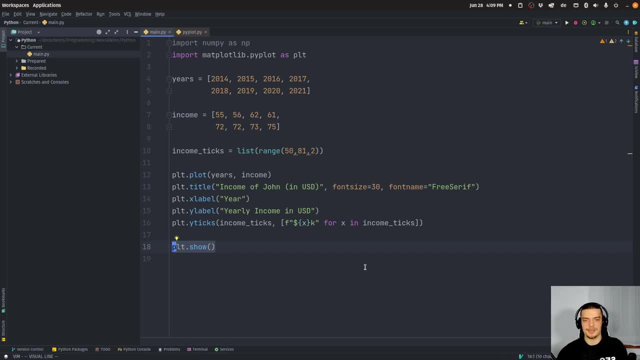 PLT show. you're going to see the different line charts, for example, in the same plot, And then, in order to explain the difference between them, you can use a legend. So let's delete all this here, And I'm going to give you an example for this. Again, I'm going to 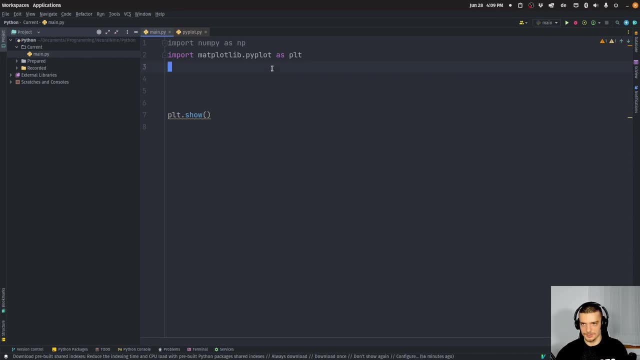 copy the data that I have prepared, Not not too complex here, just some artificial stock data. We have stock a, stock B, stock C and we have some stock prices over time here And we want to visualize those. So what I can do is I can say PLT plot. 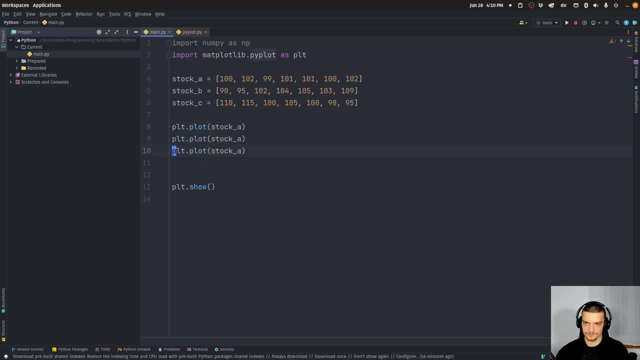 And then we can say stock a, stock B and stock C, And now we have these different line charts. By the way, you can see, if I only provide the values, the x values are generated. So if I only provide one list here, not x and y, but just y, in this case x is going. 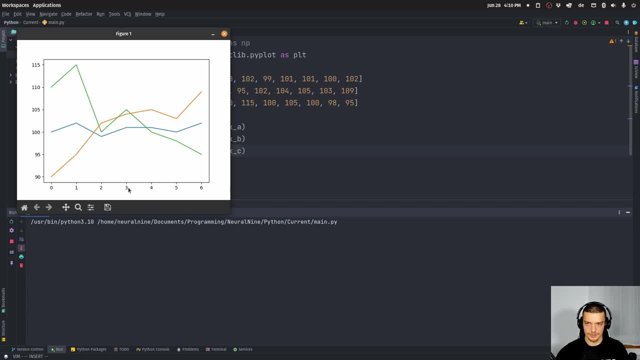 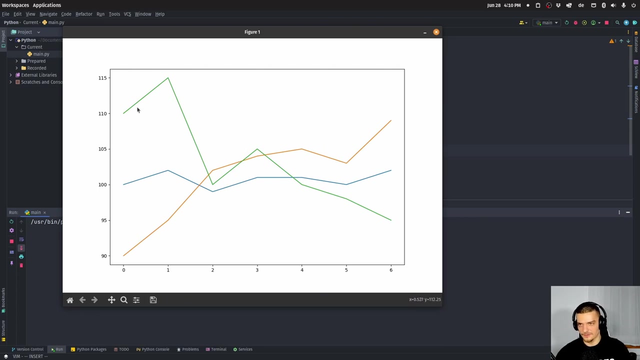 to be generated automatically with enumeration, So 0123456.. But you can see, we have now the different line charts with different colors, And what we want to do is want to add a label somewhere in the graph, for example in the upper right corner. that explains to me. okay. the orange graph is Microsoft, the 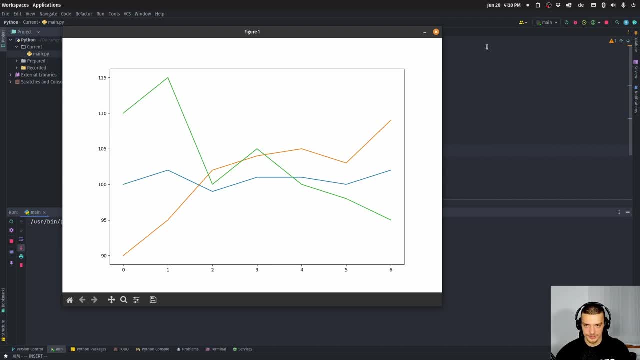 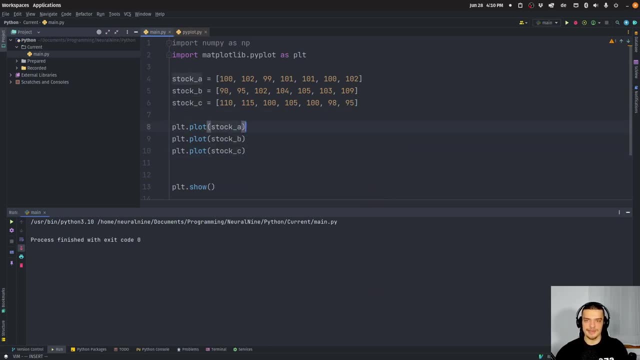 green graph is Tesla and the blue graph is Apple, for example. Of course there's not a case in this graph here, But this could be the case. And how we do that is we first of all set in the plot function the label equal to a name, So for example, company one. then we 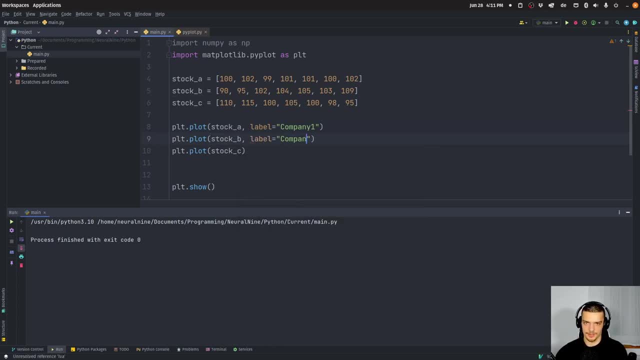 have label company two, then we have the label company three. Now this alone won't do anything. I can run this and you're not seeing a legend, But now all I have to do is I have to say PLT dot legend. And this is going to add a legend to the plot And here, in this case, by default it positions it in the upper right. 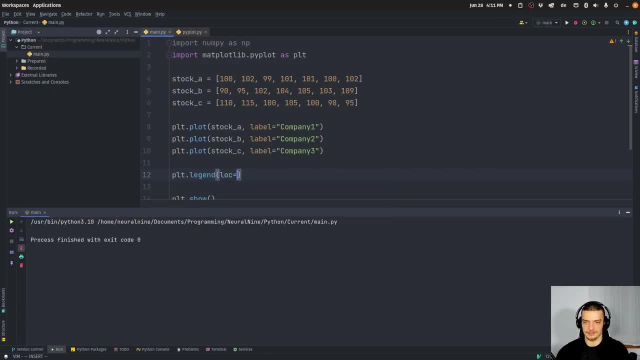 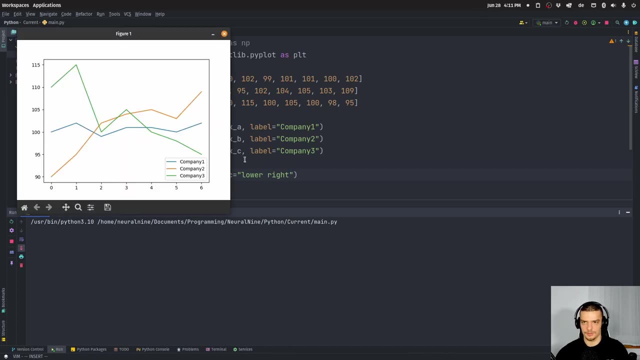 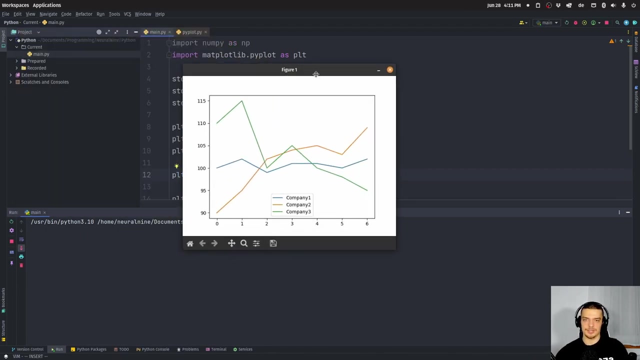 corner. I can, of course, also change this location by providing the lock keyword and setting it to lower right. or was it bottom right, Sure, I'm not sure. No, lower right is fine. Or I can also say lower center, I think. There you go, So you can reposition debts legend. 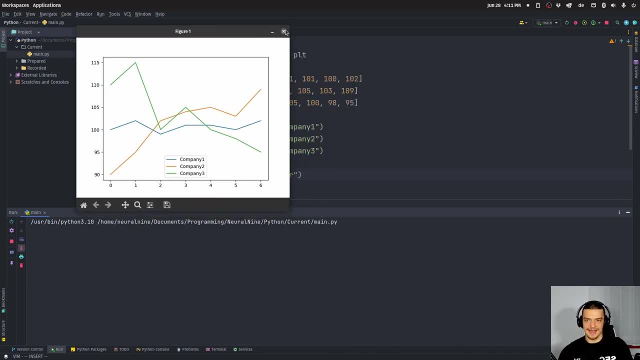 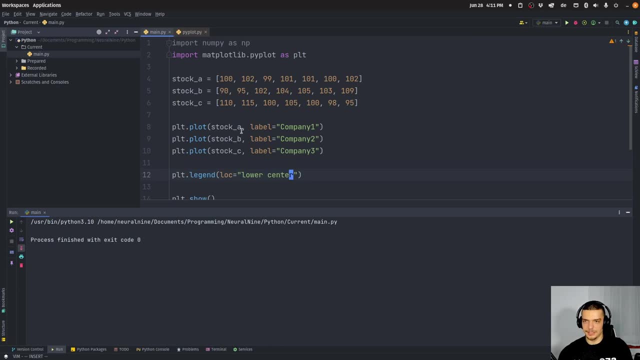 how you want, But this is also a way of adding information to the plot, making it more understandable, more readable, And this works for all the different plot types. If you have a pie chart, We can also do that with pie chart. here I can say: maybe let's call this a. 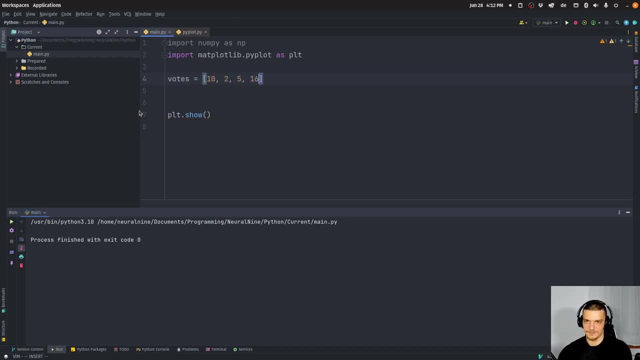 votes, And we're going to say 10 to 516, 22.. And then we're going to say people, we're gonna just say A, B, C, D and E, And here we're going to now say PLT, pi votes And what we want to do here. 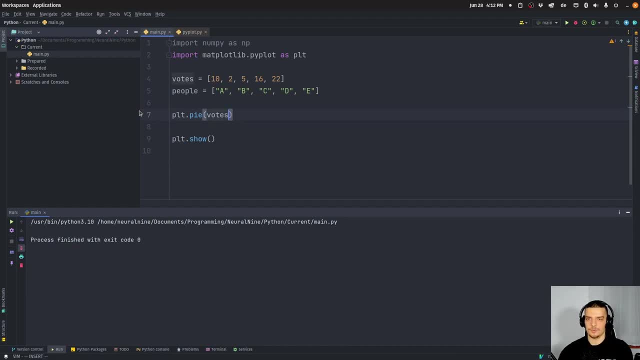 is: we want to label the vote, So we have the different votes. we're not going to actually, we're not going to actually label in the pie chart, So we're going to actually say here, labels equals none, because by default, of course, we could also just add the labels, as we did with 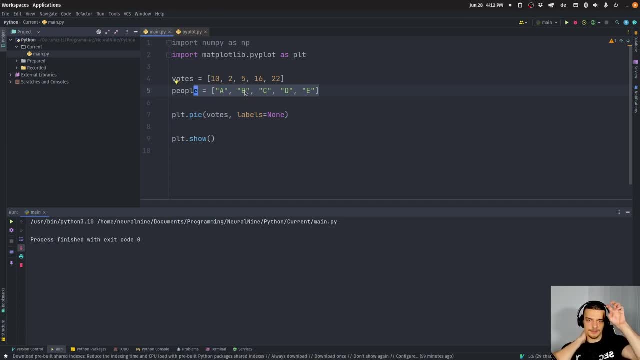 the programming languages and they would be displayed in the pie chart itself. But we can also say labels equals none, And then we can say PLT legend, And we can actually specify the labels here directly by passing the people list, And what this results in is that we can actually 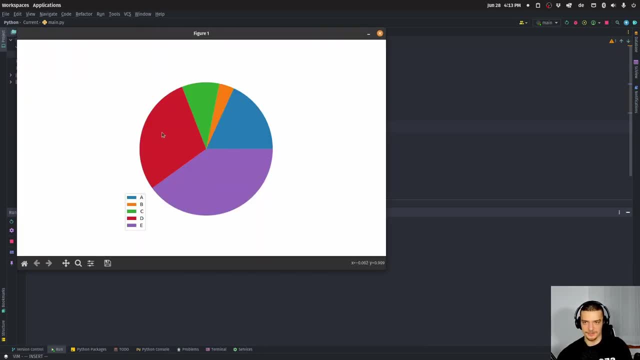 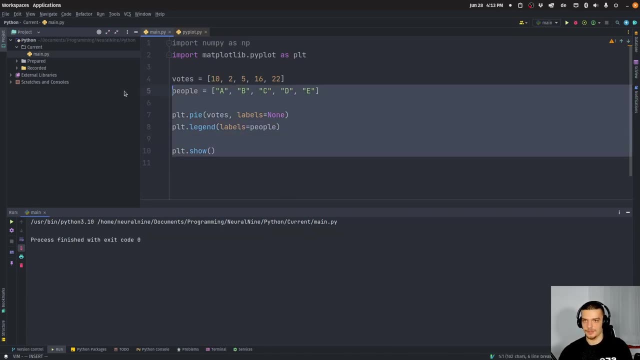 have the pie chart without the labels inside of the pie chart or around the pie chart, but we have them in a legend here. So this is also a way of labeling pie charts. All right, so let's move on to style sheets, because what we can do in Python or what we can do in matlab is we can also. 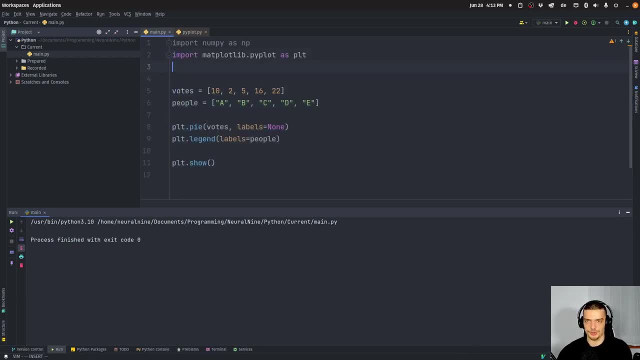 customize the styling. I'm going to keep that example here to show you that this works in a very simple way, And for this, however, we need to import something specific. we need to say from matplotlib: import style. then we can just use some style sheets So we can say: 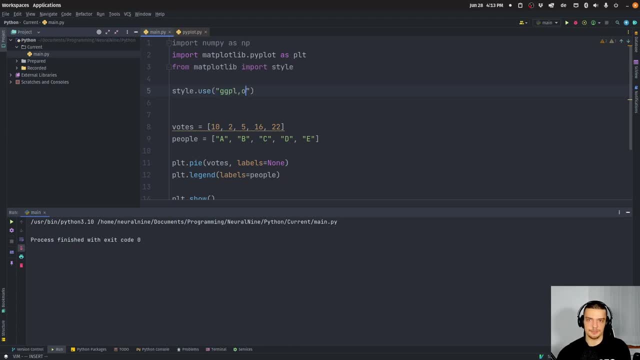 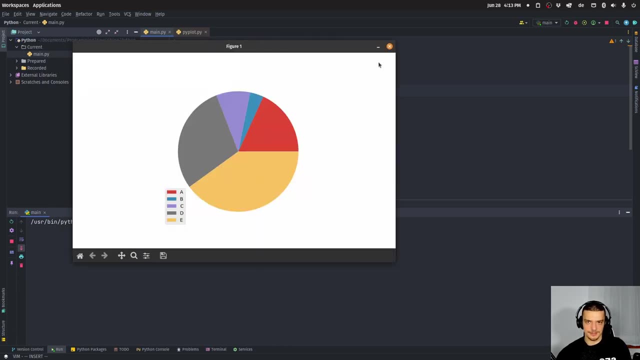 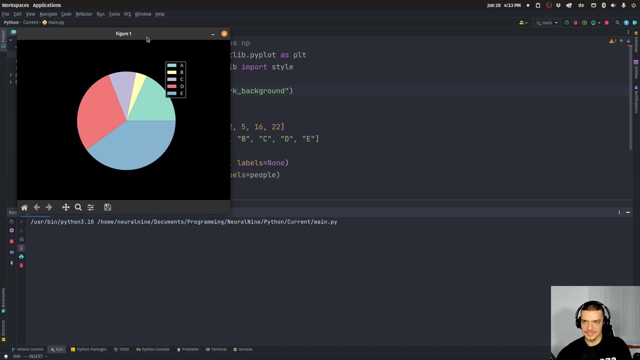 for example, style dot dot. use ggplot to get this particular style sheet And then you can see: okay, we have a different style than we had before. And then we can also go with dark underscore background And this is going to give us a dark theme And to get a full list of that, 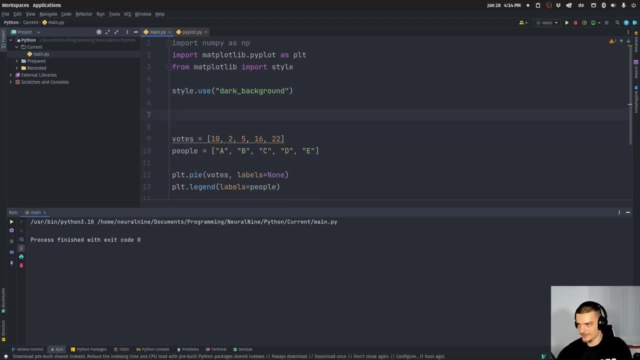 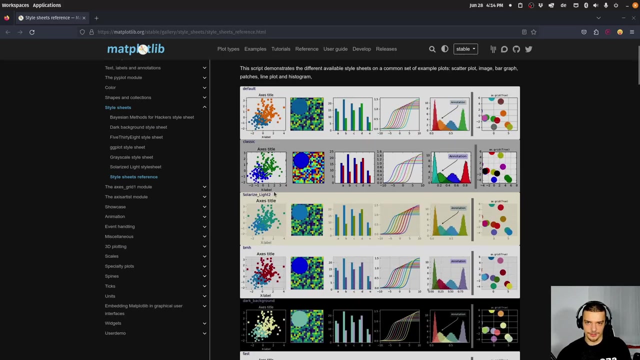 you can actually visit. doesn't copy from my prepared script here. You can actually go to these two websites. the first one will give you an overview of the existing style sheets that we have. So we have here classic, we have dark background, which we just saw, we have grayscale. 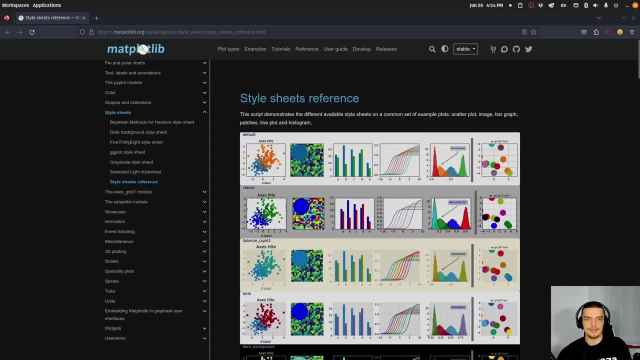 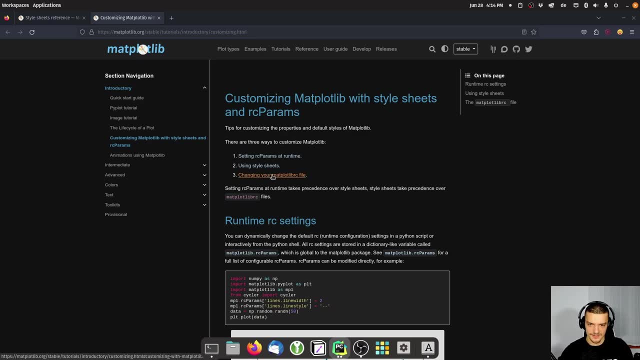 we have all these different style sheets that you can play around with. Those are the defaults, But you can also have the possibility to customize our own style sheets. Now, this would go beyond the scope of this video. Also, I think I have a video on this separately, but you can customize your own. 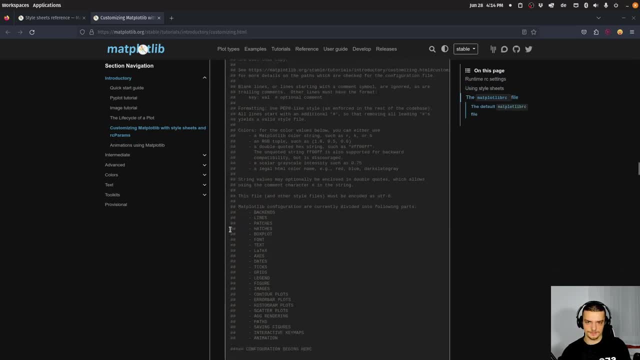 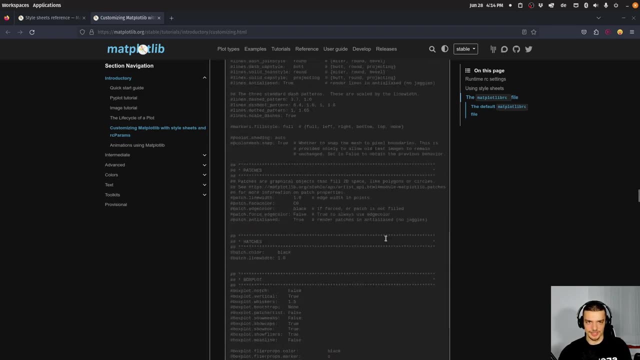 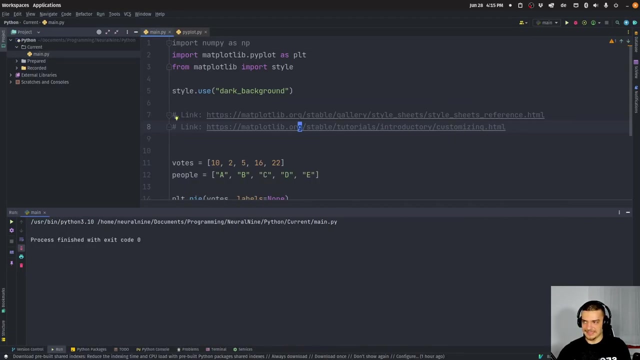 you can create your own customized style sheets and use them afterwards. But, as I said, this is a little bit too too much for this video today. You can just visit the documentation and check this out, Or you can watch my video on the topic. I'm pretty sure I have one on the channel, But yeah, 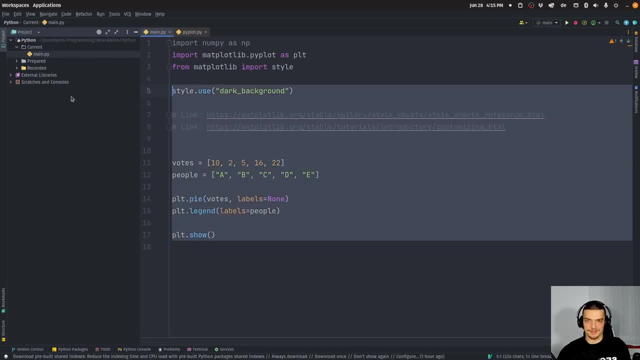 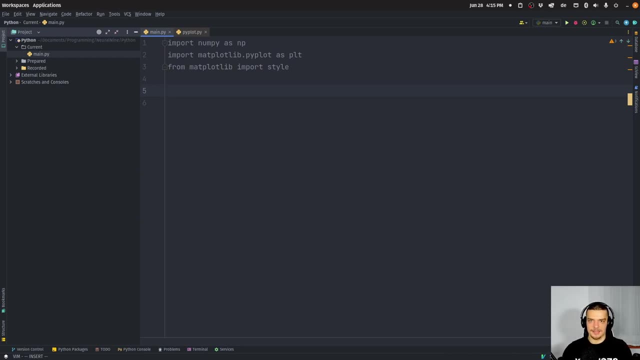 that's that. So let's move on to something more functional, which is not just about styling, but actually about functionality. Sometimes we want to plot multiple things side by side, So maybe I want to have six different histograms in the same plot or in the same window, Or sometimes I want to have different. 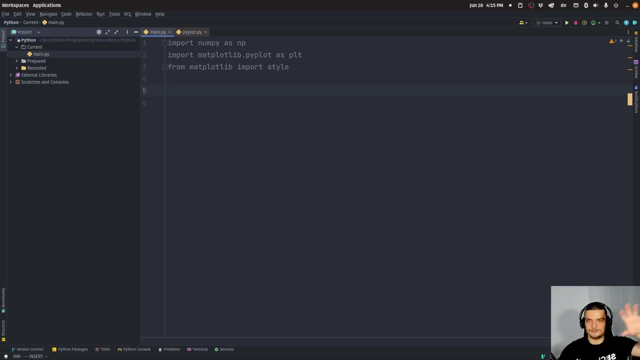 figures. So I want to have one line chart here, one pie chart here in different windows. We can do that quite easily with matplotlib. All we have to do is we have generate x1, x2, let's say we're actually x1, y1,. 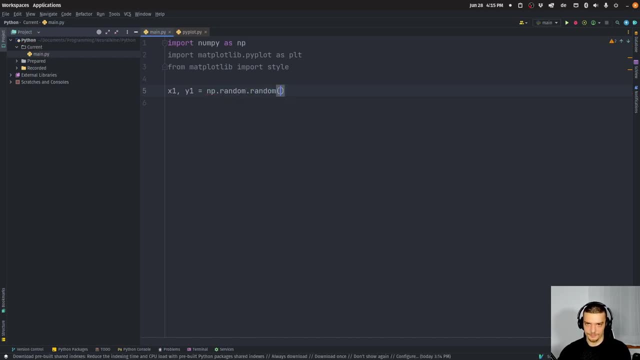 it's gonna be the endprandom dot random 100 in p random God random 100 again. And then x2, y2 is going to be for a different plot. it's going to be npa range 100 values and nprandom dot random 100. 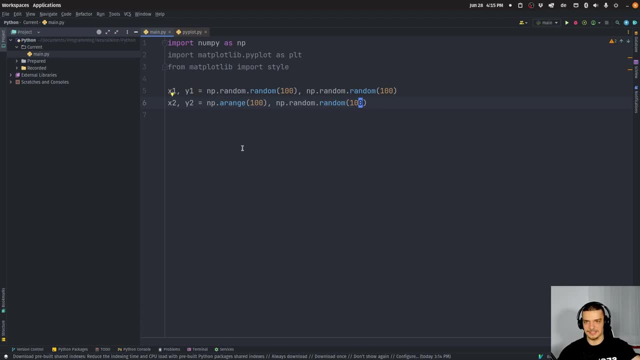 value, So range, basically. just, we're going to use this for the x axis to make this a line chart and make this more reasonable. say now: PLT, dot figure. I'm going to say figure one. I'm going to say PLT scatter x, one data and 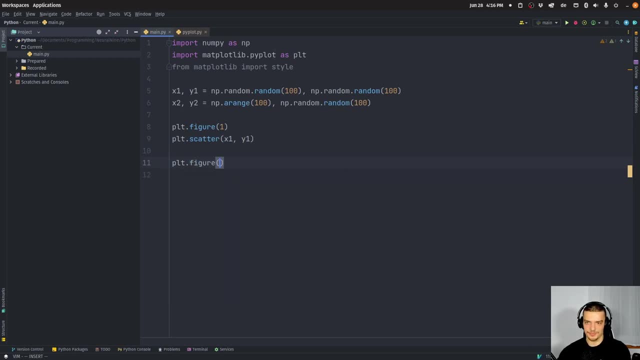 y, one data, And then on PLT, figure two. this is how I specify that I want to have a second, separate figure here. I'm going to say PLT plot, then x, two, y, two, then PLT show, And you will see that. 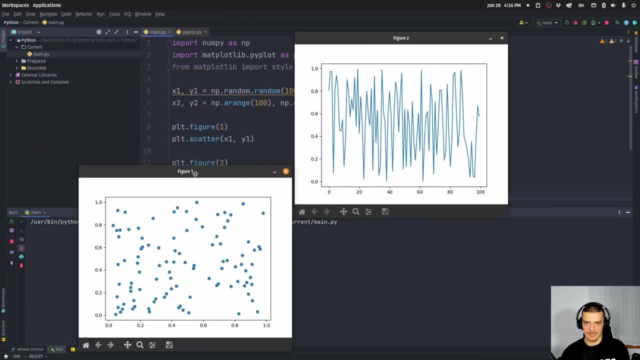 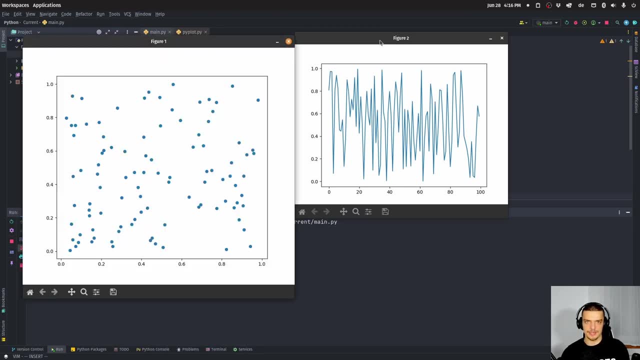 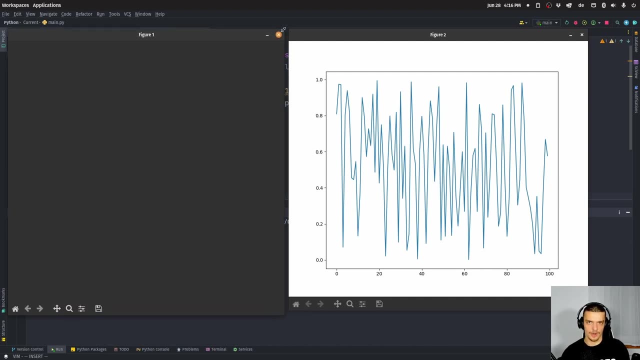 this plots two figures here in separate windows, because I'm defining two figures and then I'm calling the show function after I plotted on both the figures, And those are now two independent figures, two independent windows that I can look, look at while interpreting the data, for example, 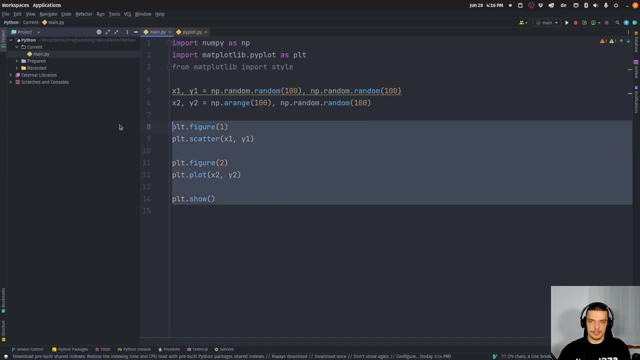 So this is one way of doing it. what you usually do is you do sub plotting, So you use one window, one figure, but you have different sub plots in that one window. So for this, what we're going to do is we're going to say: 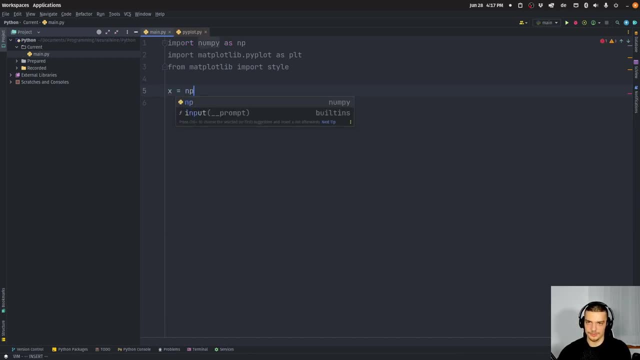 say, x is going to be equal to NP, a range, a range: 100.. figure axis equals. now we're going to use the function called subplot, So PLT subplots. we're going to define a grid. we want to have a two by. 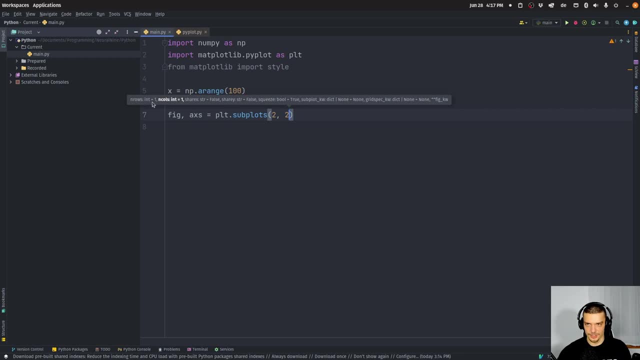 two grid, So two rows, two columns. you can see the parameters are n rows and columns And now we have basically one figure with four different axes. we have zero one, one one or actually zero one, or, sorry, we have 00,, 01, one zero and one one. So this is a grid of four subplots in. 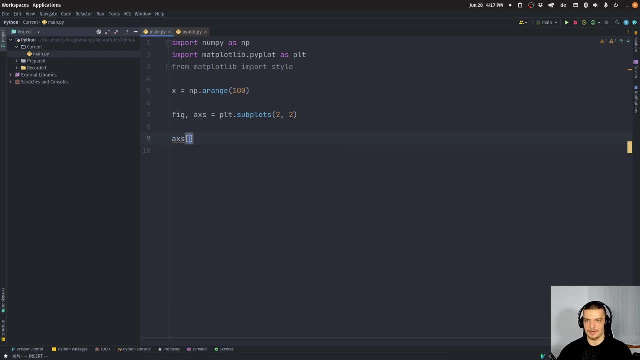 one figure, And we can access the individual axes here by saying axes 00,, for example, plot x and then maybe NP sine of x. So we're just going to plot some functions here. then we can say: axis 00, dot set underscore title. Now we cannot just say dot title here. 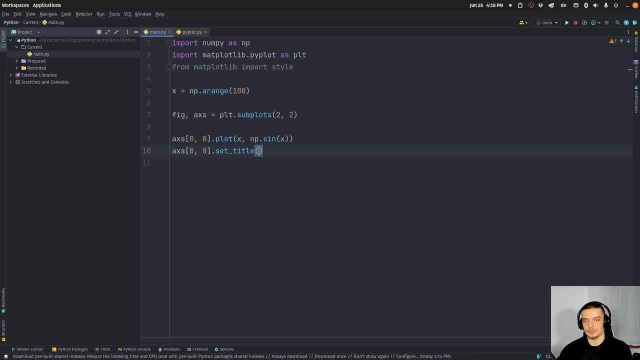 we have to set, say set title on the axis. So set title sine wave, for example, And then I can copy this here. I can change this to 01.. So the first parameter here indicates the row and the second one to column. So this would be row zero, column zero. this would be row zero, column one, And you. 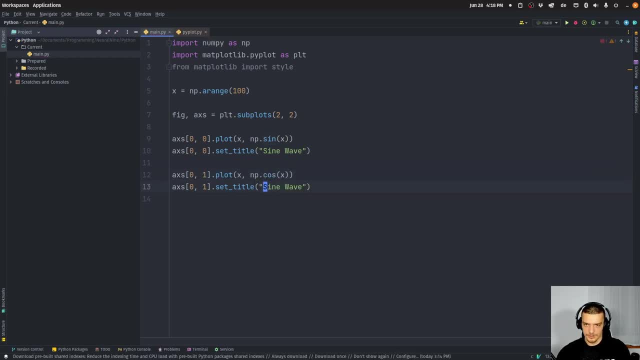 want to do a cosine, for example cosine wave, and then we can copy this again: One zero, one zero. and then want to do x and then plot it against some random noise or random random 100. And then we're going to say random function And then finally want to say: 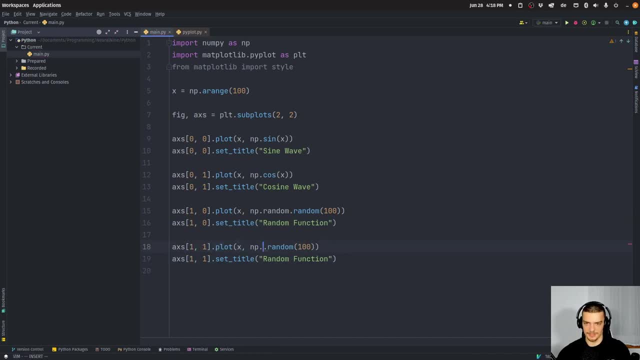 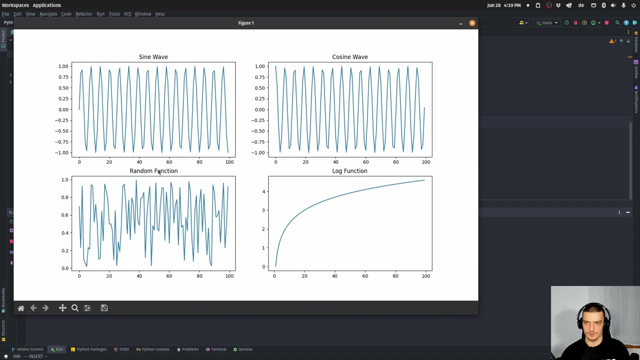 1111, want to plot maybe the logarithm effects. So log function, and then we can just say CLT show, And we're going to see that we have four plots in the same figure here. So you can see we have sine wave, cosine wave, random function, log function And of course on each 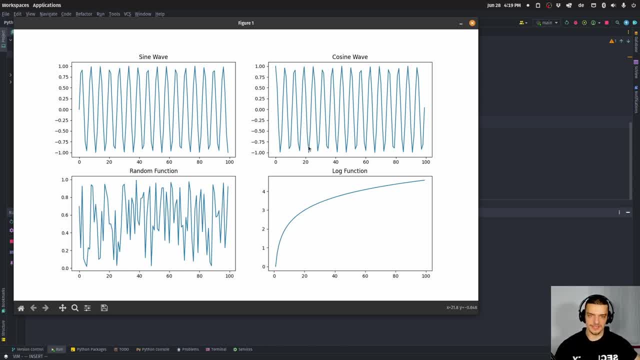 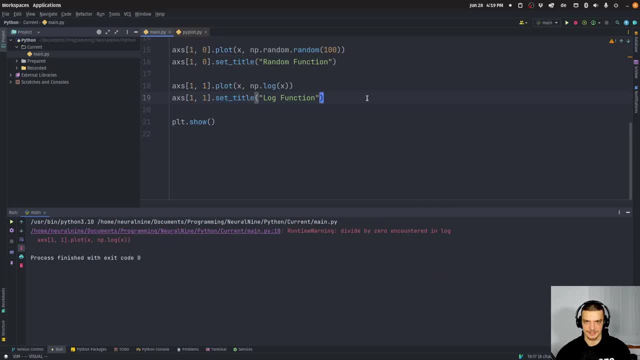 of those subplots we can now actually specify all the different parameters that we talked about before, So the title, the x label, the y label. but we have to do it with this set type of function, So axis or axes 11, set x label test, for example. 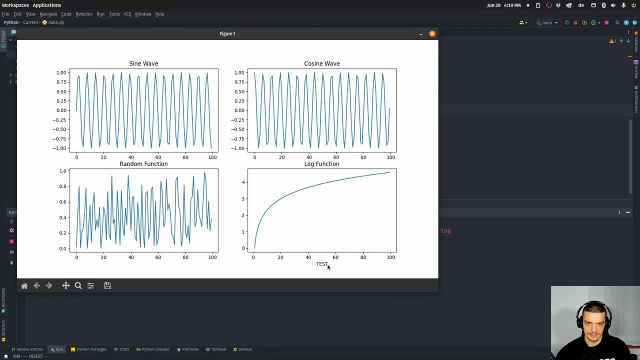 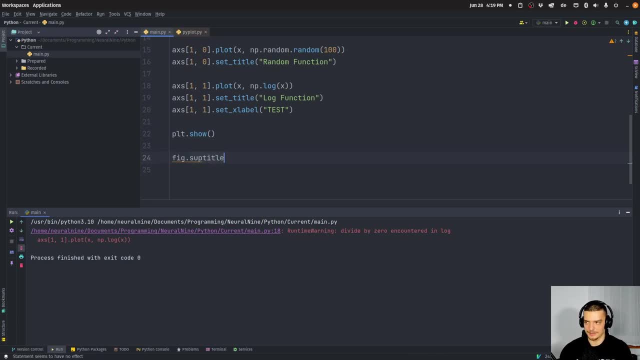 And then you can see that this particular plot has this x label test here, And of course the whole figure itself can also have a super title. So we can say figure sub title four plots, for example, And of course we want to do that before the show. 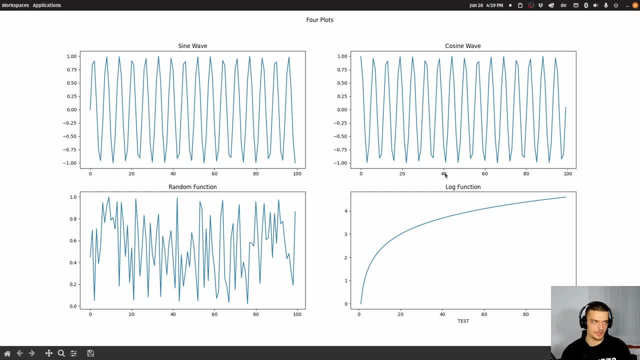 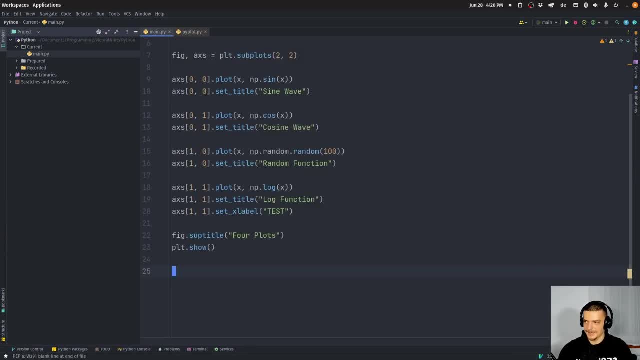 And then we have sine wave, cosine wave, random function, log function. we have the four plots subtitle up here. So this is how you do subplotting. Now, before we get into the more advanced stuff, I want to show you how you can export something. how you can export. 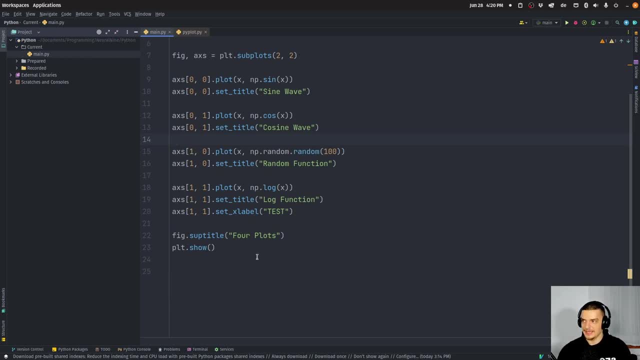 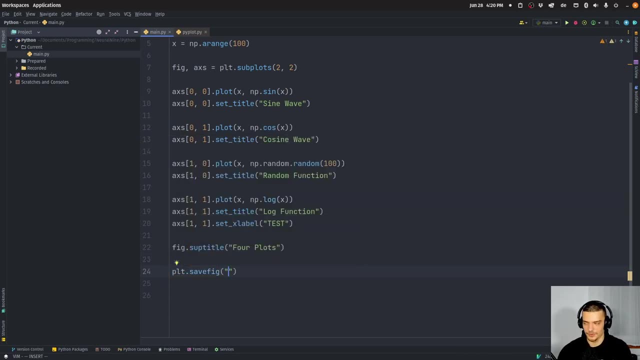 a graphic, instead of plotting it, instead of showing it actually. And how we do that is we just call the PLT dot save figure function, So PLT save fig. and then we're going to say, for example, four plots, dot PNG, And I think that already should be enough to produce. 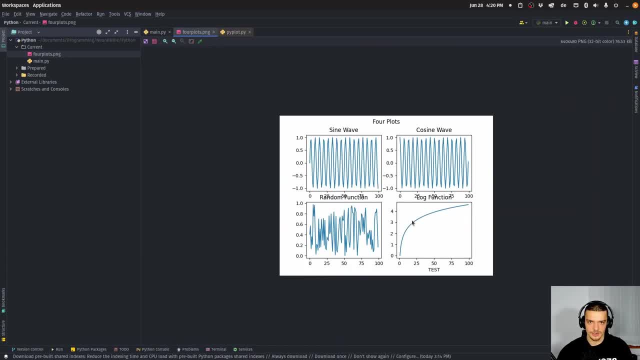 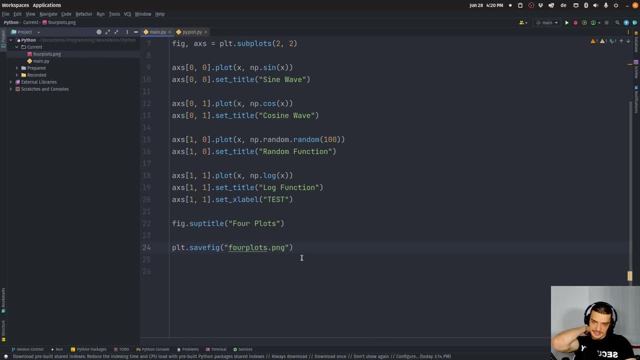 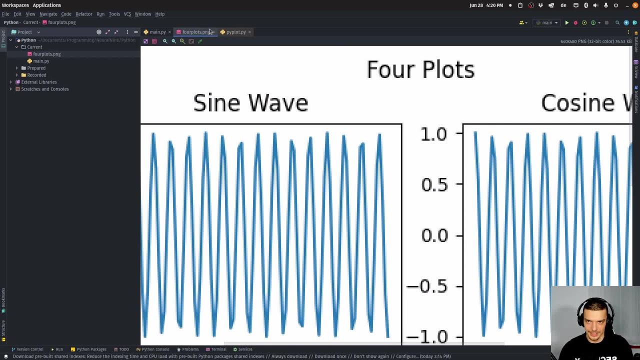 produce a plot. There you go. we now have a PNG image of the plot, As you can see here, um, so that works, But of course we can also specify different parameters here. So you saw that the quality isn't that high. So you can see that this is not a very high resolution. 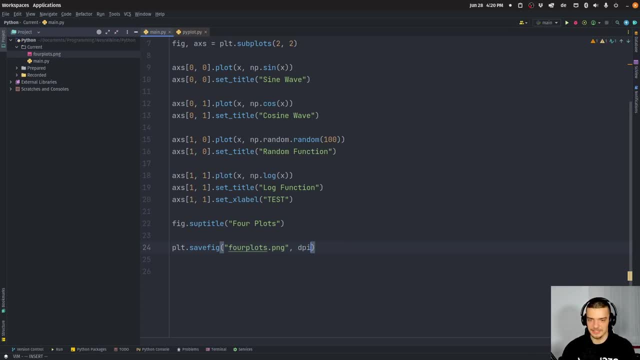 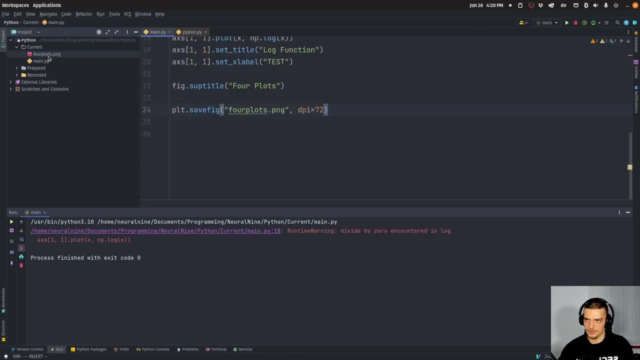 So what we can do is, in the save figure function, we can specify the DPI to be equal to 72,, for example, And I think that this should result in- or does it not? sure doesn't seem to result in- a higher quality, maybe if I go for 300. 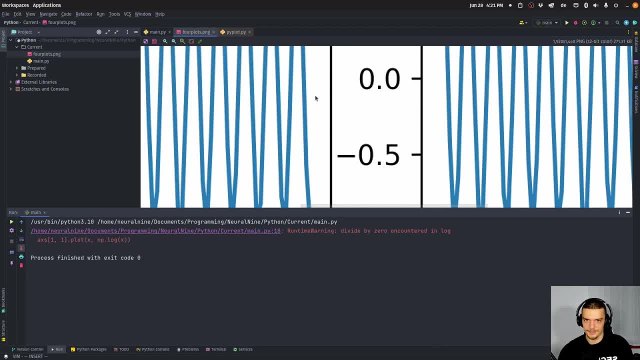 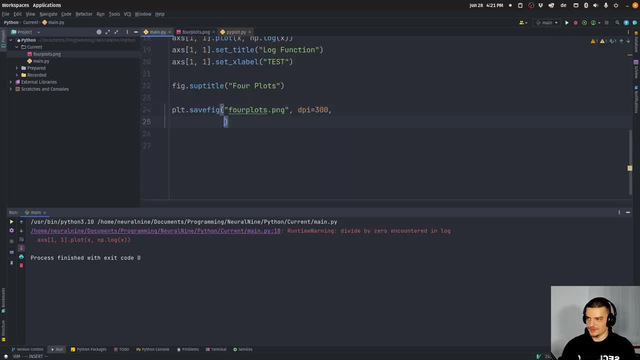 Oh yeah, then it results in a higher quality. There you go, So that is something we can change. then we can also say that we want to have transparency. So trans parents equals true, which basically makes it without the white background. then I can also set this to false. 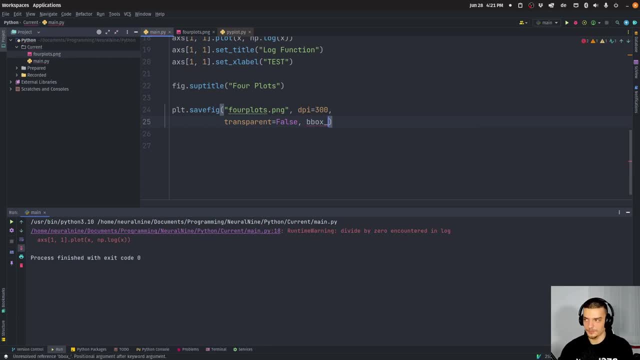 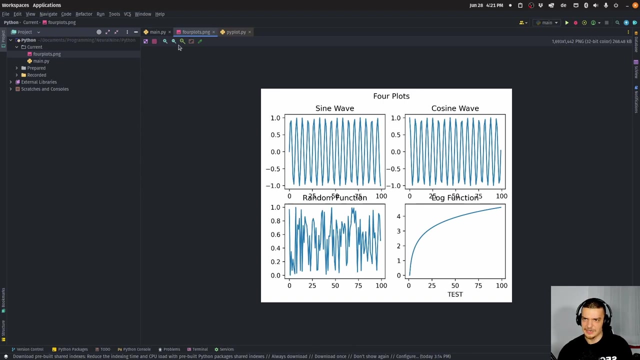 against it. we can see the results. actually, the box boundary, box inches, is going to be equal to tight And, yeah, this just, I think, cuts off the distances here. Now I'm not sure if, if I call, I think they should be able. I should be able to do that with PLT tight layout. 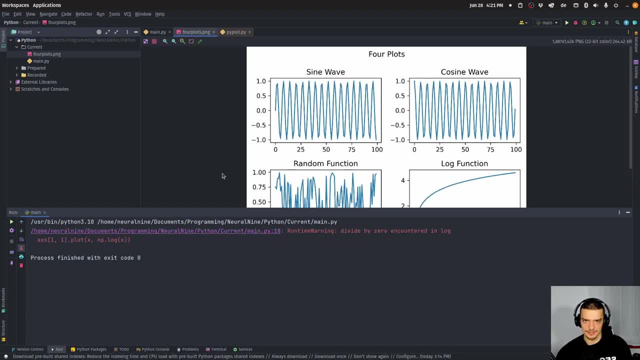 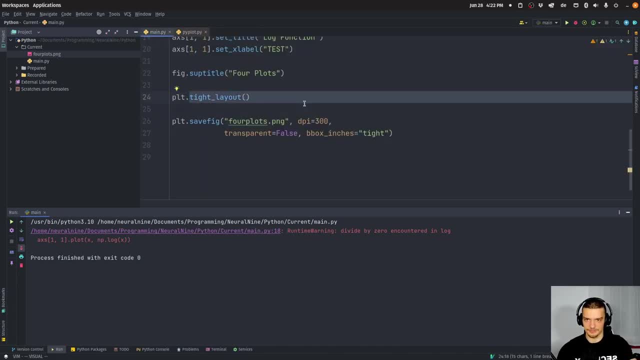 Yeah, then we don't have this overlap between the labels and the headings or the ticks and the headings. So PLT dot tight layout basically structures everything so that it doesn't overlap unnecessarily And this basically just cuts, cuts away the boundaries or the padding. So if I don't do this, we have, I think, more space towards. 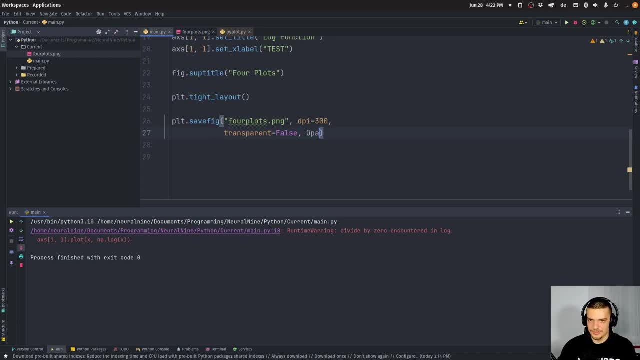 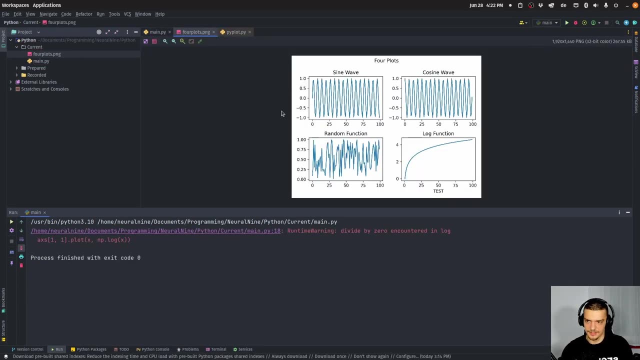 the edges, if I'm not mistaken, And then we can also say: I think pad underscore inches 0.2.. What does this do? Again, I think it just adds more padding. So I think we should see that if I set this to 20.. 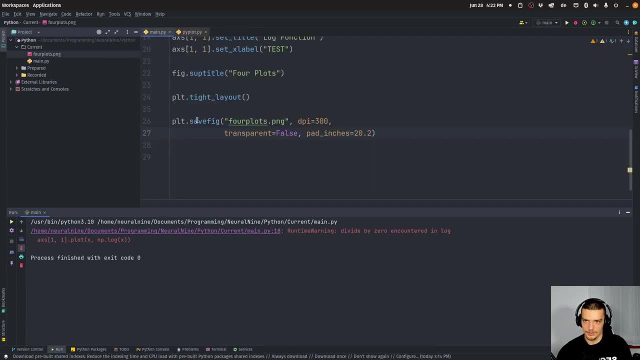 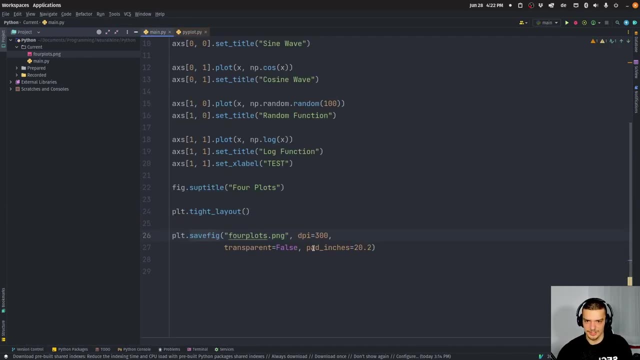 No, it actually doesn't change much. Does it say what this parameter does? I'm pretty sure it's about padding, but maybe it doesn't work in this particular case with a subplot. But we can. you can read that up into documentation And maybe I'm going to. 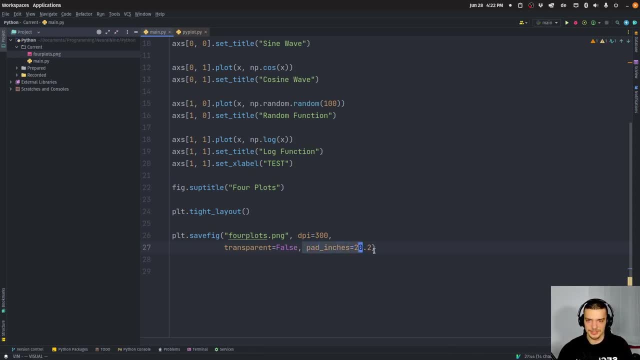 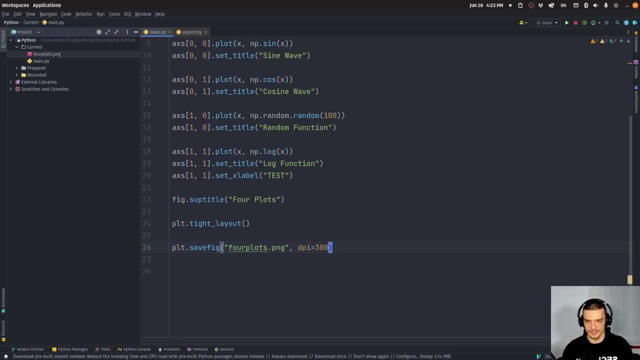 add some annotation here off what it actually does. But you can also specify- this is the important thing. you can also specify some parameters here to decide how exactly the picture is going to be exported. But instead of doing p it show, you can do PLT, save figure or say fig, and then you're going to actually export it into. 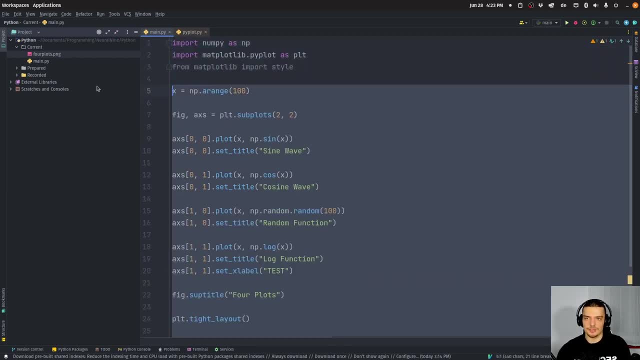 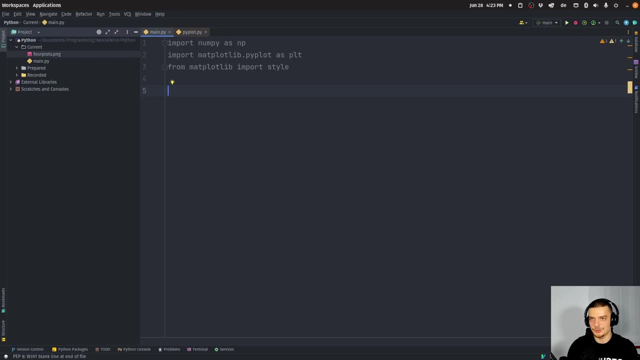 an image. So now we're going to move on to some more advanced stuff, to 3d plotting and animations. So up until this point we plotted in two dimensions. we had scatter plots, line plots and stuff like that In two dimensions. Now we want to get into three dimensions And for 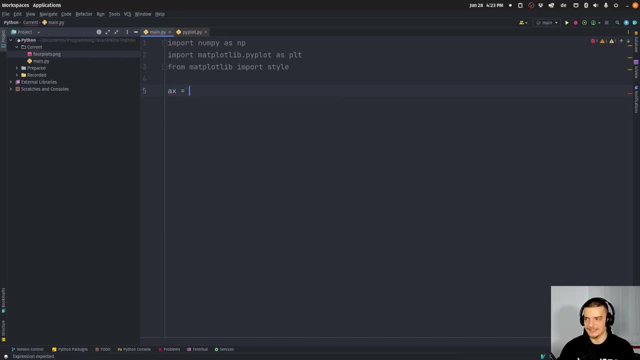 this. we're going to create a new axis. we're going to say: axis equals to PLT axes, projection equals 3d, three dimensional projection. And now what we can do is we can define x, y and z value. So NP, random, random, 100,. I can copy that two more times: 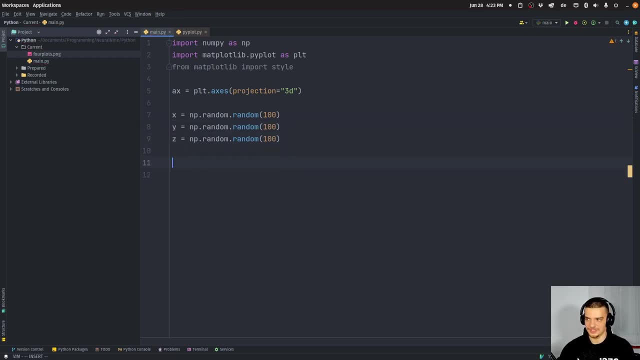 And I can change this to x, y, z And then, instead of scattering in two dimensions, I can say axis scatter x, y, z, and then I can say axis dot set. underscore title: uh yeah, 3d plot, and then plt show and you can see we have a three-dimensional visualization. 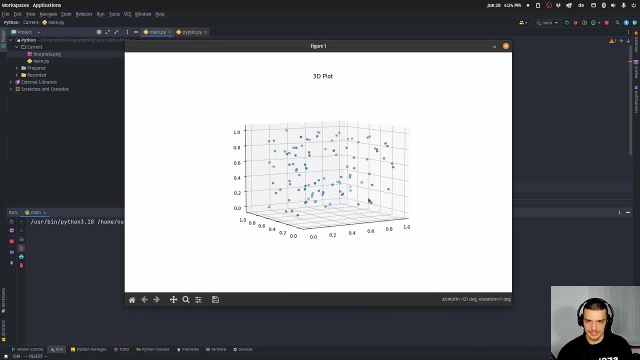 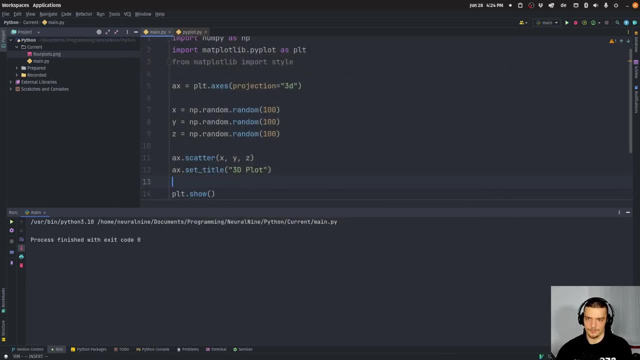 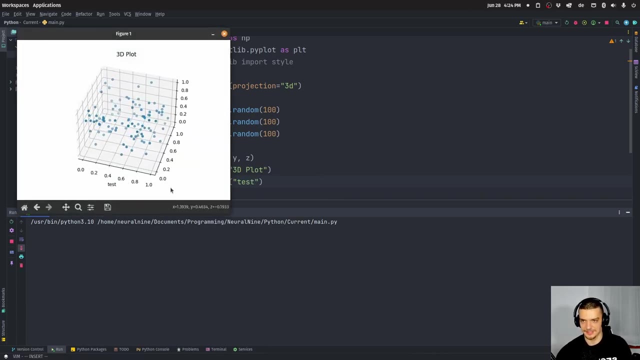 now, and i can also rotate this. you can see, we can look at all these scatter plotted points on the different axes, uh, and of course we can also do the same thing here. so, axis set, x, label test, and this of course then labels the x-axis, and the same goes for y and z. 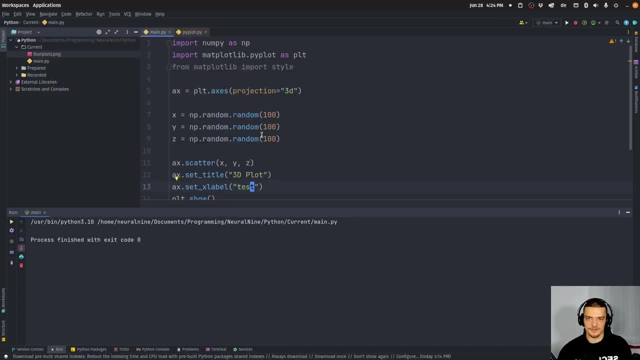 so all the stuff that we already know about also works in three dimensions. now if i want to say, uh, if i want to plot a line plot instead of a scatter plot, i can just use the plot function here again. so in this case, of course, it would make sense to use 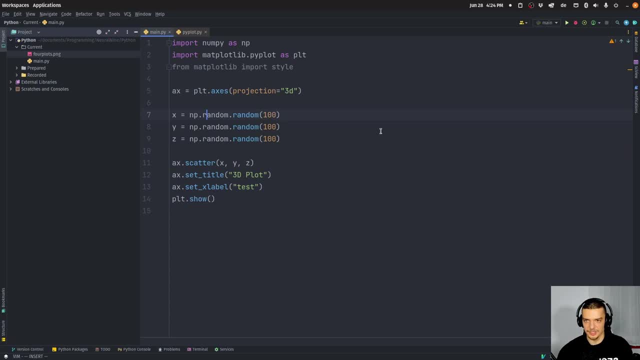 uh, different values. so i would not use random, i would use a range for x. so a range for x, let's say, for example, a range from zero to 50, with a step size of 0.1.. And then I would say: 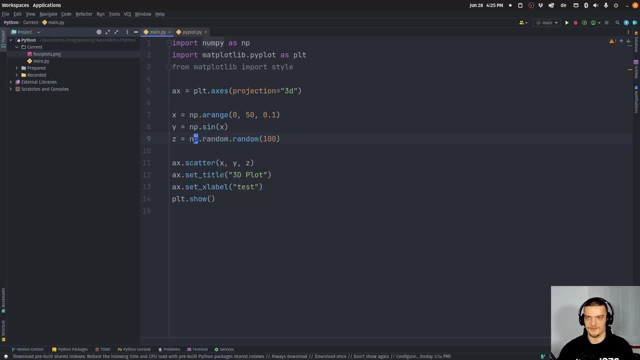 np sine of x is going to be the y value and np cosine of x is going to be the z value. And then I'm going to just say plot x, y, z. doesn't make a lot of sense necessarily, But you can see. 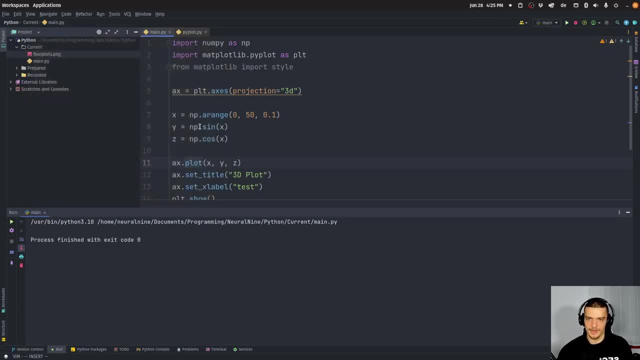 this is the result of that, Or maybe I can just say here: a range from zero to 50, with 0.1, here as well, And then this is just going to be cosine of x plus y or something, And then you can. 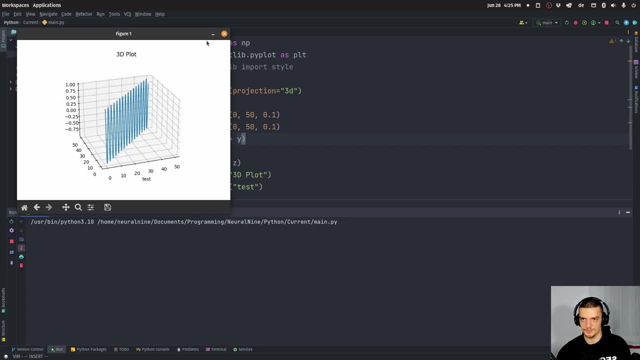 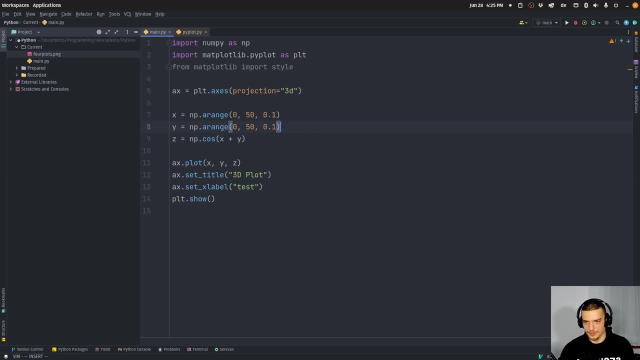 see we get this function here in three dimensions. Yeah, so that is a simple line plot. Now the interesting thing here to do in three dimensions is a surface plot. So we want to have actual areas, actual surfaces, being plotted, And how we can do that is we can generate x and y values. 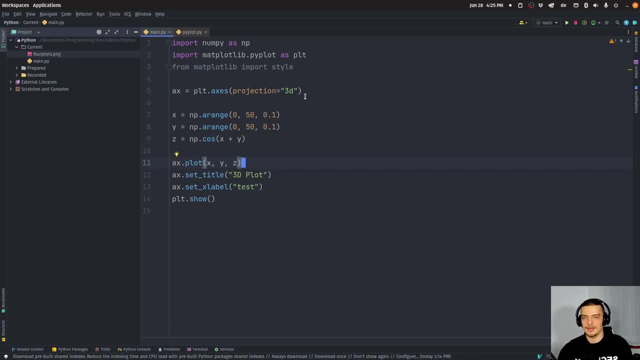 then we can create a mesh grid, a so called combination. So basically you can imagine it like that, And then we can create a mesh grid, a so called combination. So basically you can that we have the- the x values 12345,, for example, and then we have the y- the y values 12345.. And 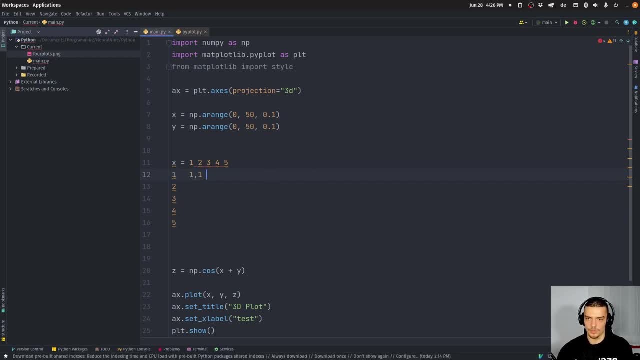 what we want to do now is want to plot all the combinations, So one one, one, two, one, three and so on, want to have a grid of all these values, that we can plot surfaces. How we do that is actually not too difficult, So we're going to just change the range here a little bit. For example: 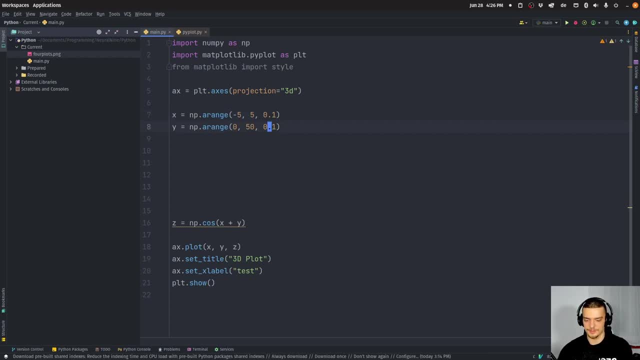 from negative five up until five with 0.1 step size. negative five or five 0.1 step size. And then, in order to actually create the mesh grid, we're going to say x, y, capital, x, capital y. 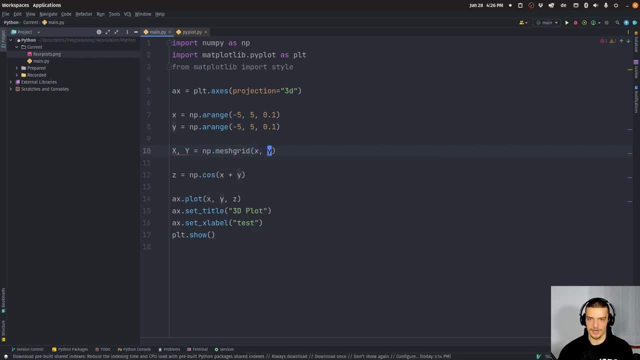 equals NP mesh grid from x and y, And then the z value is going to be actually capital. Z is going to be NP sine of x times NP sine of x. So that's going to be the mesh grid, And then we're going to 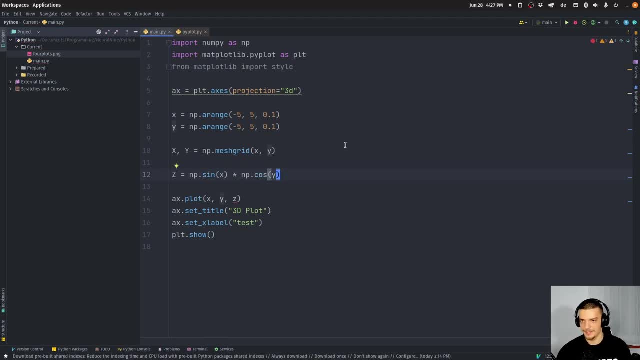 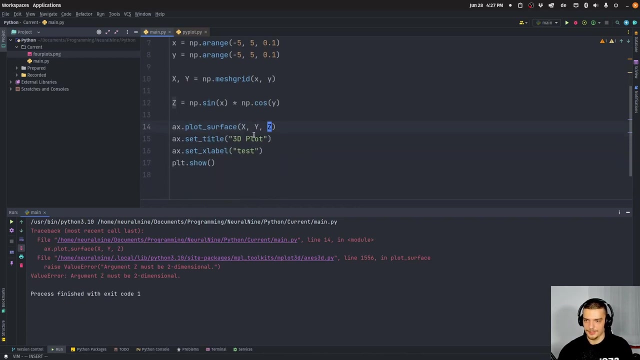 and p cosine of y, for example. And to actually plot the surface we need to call the plot surface function and call x, y and z, And we can also specify a color map here. Z must be two-dimensional. What's the problem here? 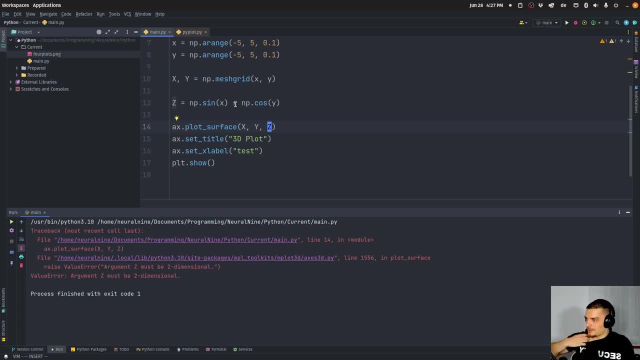 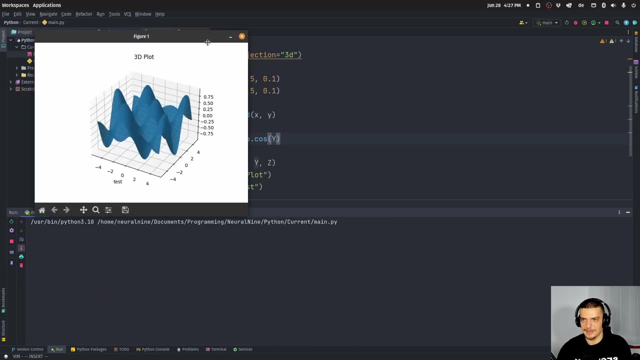 Let me just check. We have the axis 3D, We have the values. We create the mesh grid. Oh, I'm using the lowercase x and the lowercase y. This is the problem. There you go. Now you can see. we have this surface plot here. 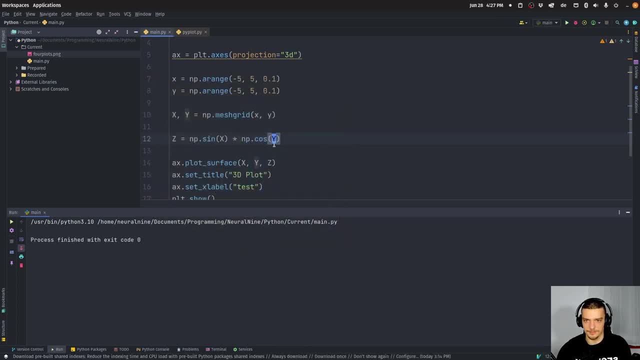 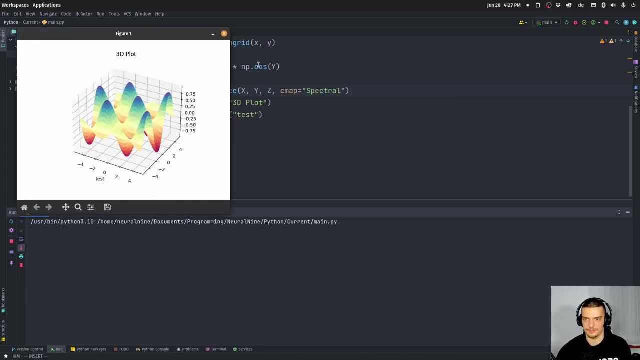 And of course the surface plot can also be made more interesting by specifying a color map, by specifying the cmap parameter, And we can use spectral as a color map here, for example. And then we have this beautifully looking surface plot here in three dimensions. 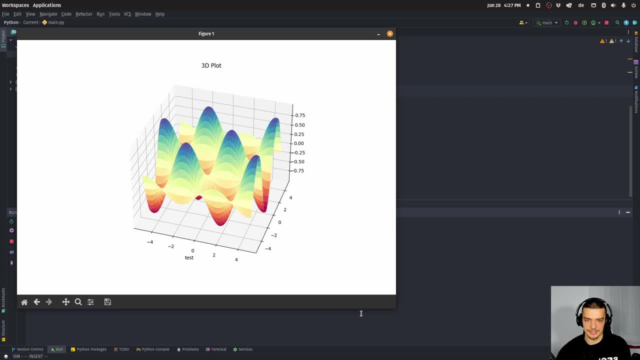 And what you can also notice here in the lower right corner when you look at it while I rotate the graph, you can see we have this azimuth and this elevation parameters. You can see that basically when I rotate it to the left or right. 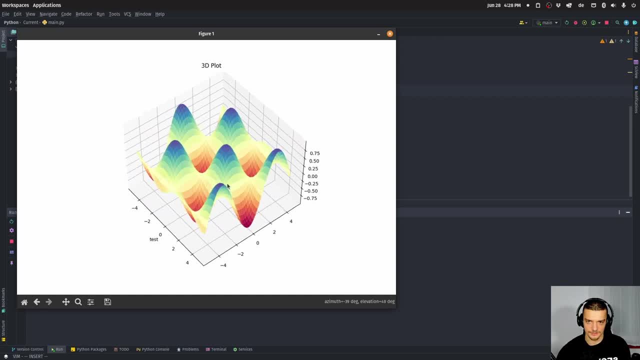 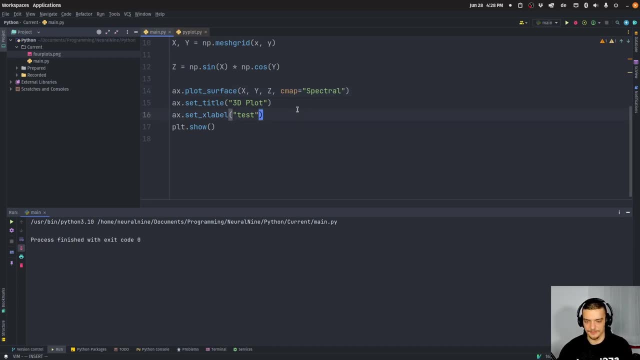 we change the azimuth And when I rotate it or when I shift it up and down, you can see the elevation changes. And we can of course also just set this automatically. So I can say axisview underscore init. It can be set to an azimuth of 0 and an elevation of 90.. 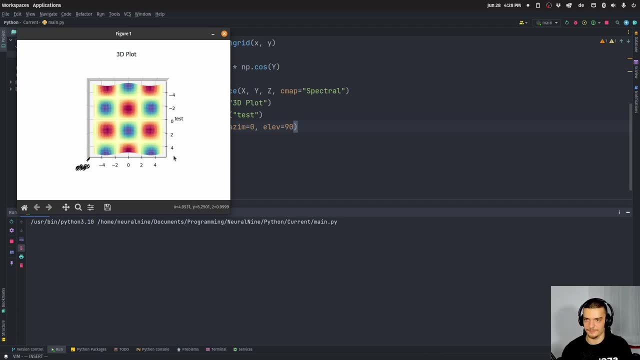 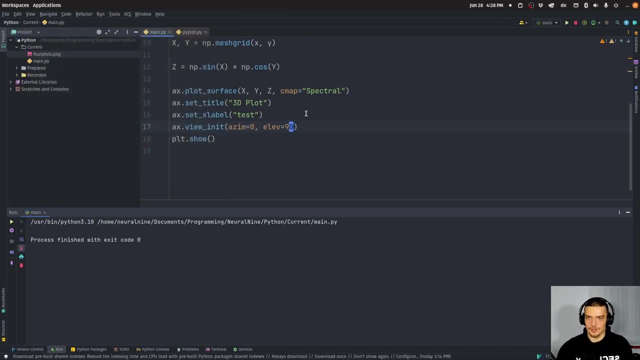 And then we would get a different detail view from above, But of course I can still rotate it, But this view would be the default then. Yeah, So that's it for the 3D plotting. Now we can finally get to the animations. 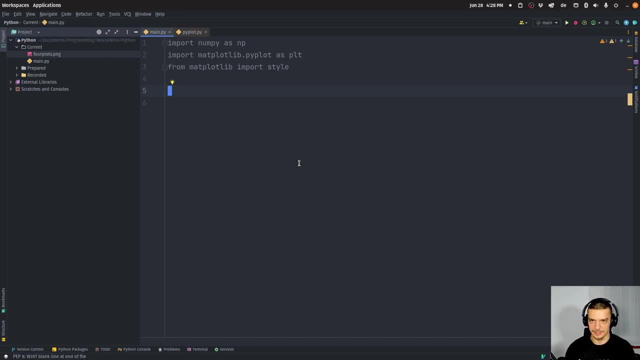 because we don't have to constantly just look at a static image. We can also see some animations, And one animation I want to show you here as an example, and then you can apply the same principle to all the other plot types that you know. 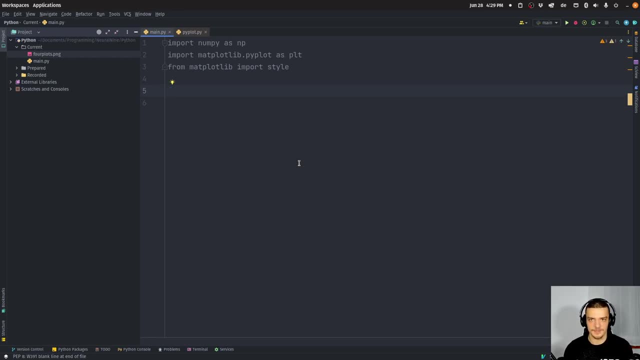 is: we're going to flip a coin, We're going to flip a 50% coin, so heads or tails, And then we're going to just keep track of the results. So we're going to say here: import random from core Python. 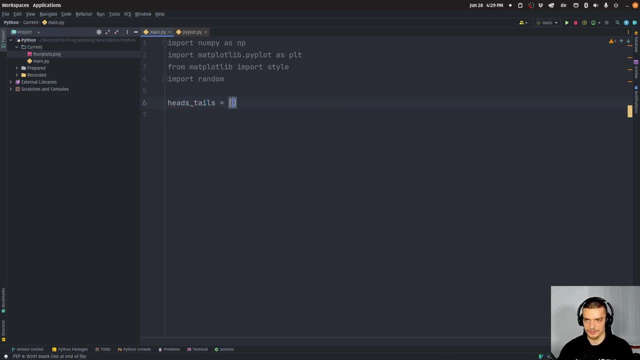 We're going to say heads underscore tails equals 00 by default. And then we're going to just say for some placeholder in range, we're going to do 100,000. And coin flips and we're going to say here head tails is going to be random dot rand int zero, or one is going to be added. 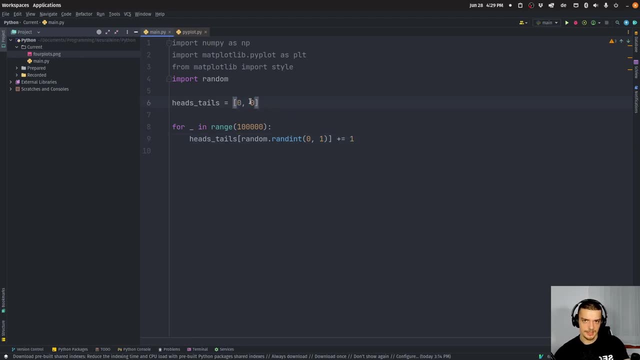 We're going to add one to that. So we have either index zero, which is heads, or index one, which is tails, And one of those two is going to be increased by one with every iteration, 100,000 times. Now we're going to plot a bar plot. 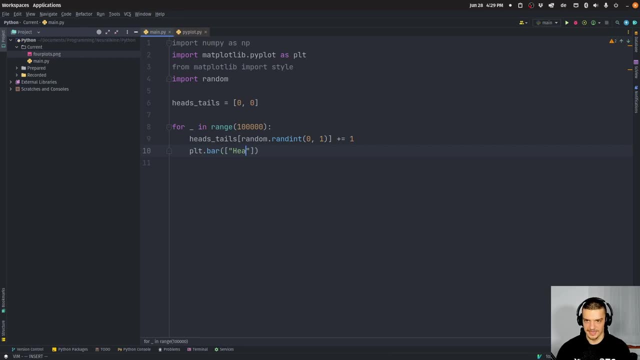 So PLT bar with heads And tails here, and we're going to pass heads, tails as the y values. we're going to say color is going to be equal to red and blue for the different bars. So we can also pass a list here as the color. 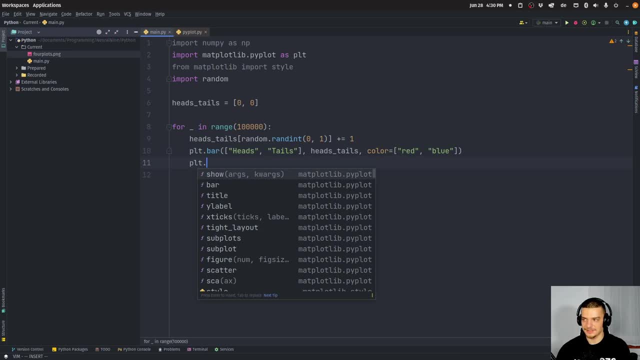 And instead of now just showing it, we're going to use the PLT pause function, So 0.001 delay. And this function is like show, but it's it animates actually the procedure. So it shows, but then it continues with the plotting and in the end we want to do show. 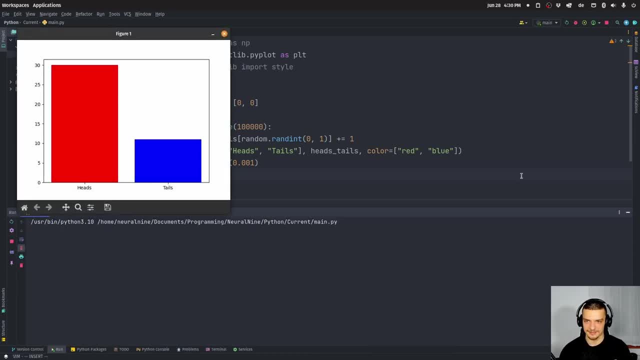 so that we can see the final result. And this is what we get then as an animation, And, due to the law of large numbers, we should eventually get something like 5050, since it's a 5050 procedure. In between, the values might be farther apart. 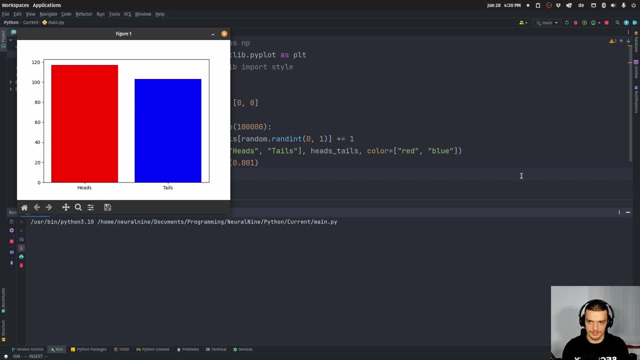 but at some point they should be roughly the same And you can see that tails is catching up here slowly. But yeah, you can see how many times we get heads, how many times we get tails. you can see the progress on the y axis. 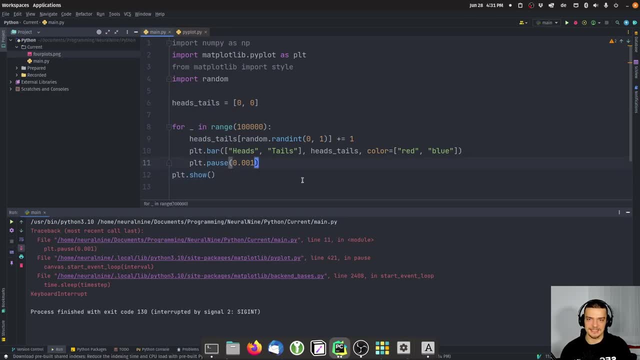 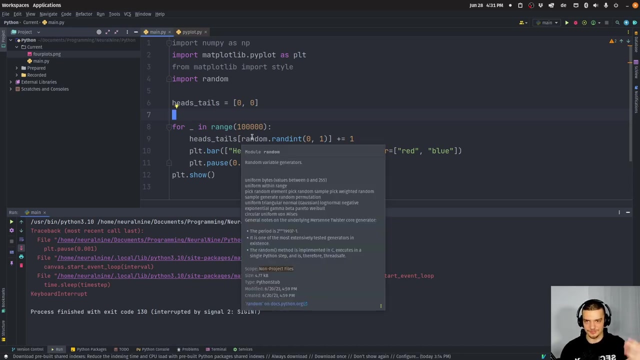 And this idea. this is just one example here, But this idea of doing something and then using pause instead of show. this animates the function. So whatever you do you can, you can actually animate it by using pause instead of show, because then it just shows, it continues to do an iteration. 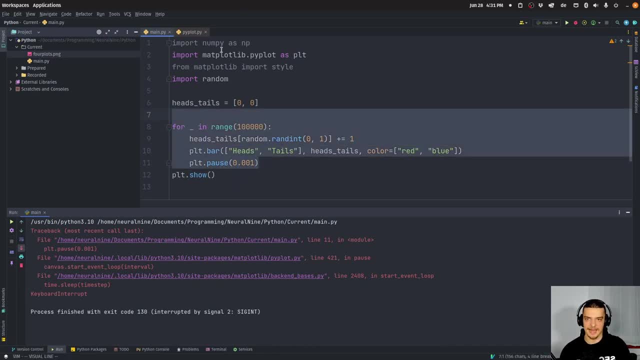 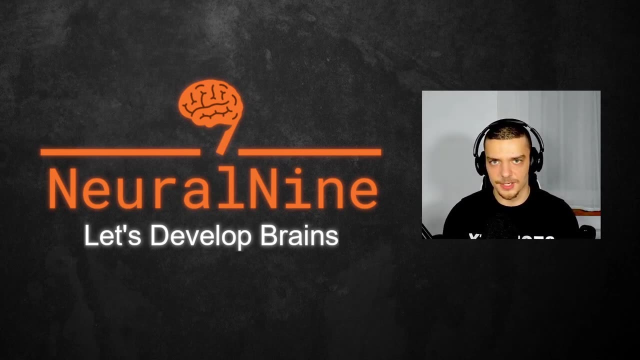 then shows it again, and so on and so forth. So this is how you animate the functions. So that's it for today's video. I hope you enjoyed it. I hope you learned something. If so, let me know by hitting the like button and leaving a comment in the comment section down below.